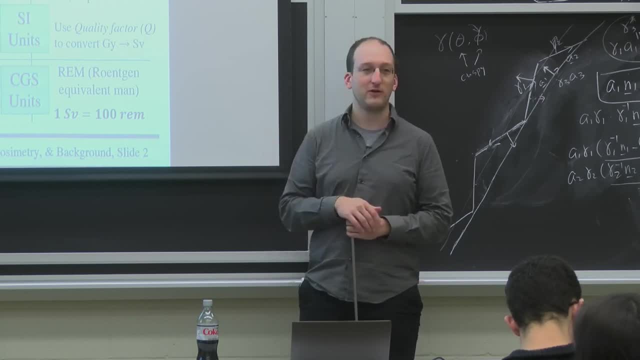 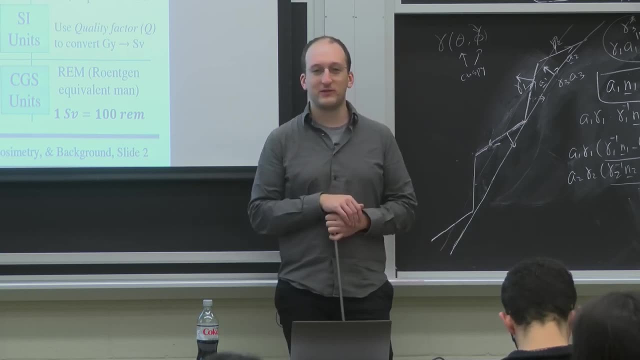 There are some that are too hard And there are giant pieces missing, like most of what we're going to go into today on sources of background radiation and where do cosmic rays come from and what are they. So thanks to whoever said that, because it spurred me off on a. let's make this. 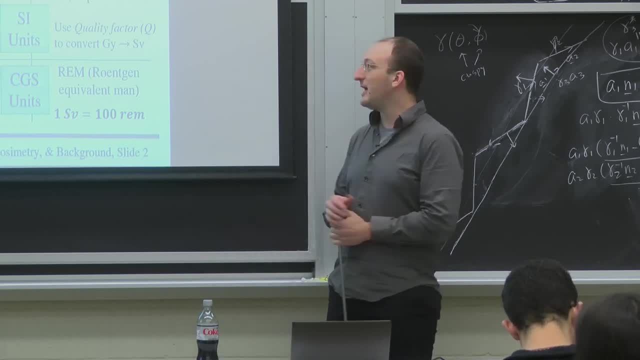 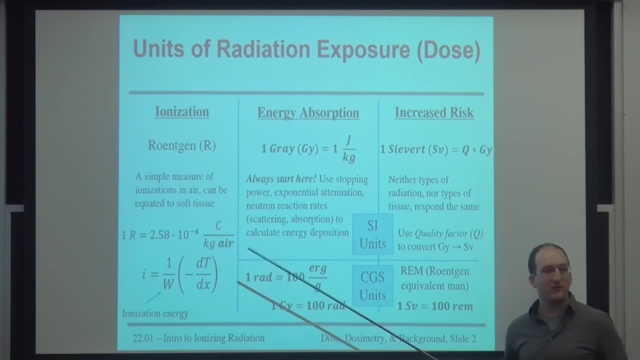 into a book kind of thing. I want to quickly review what we did last time. We went over all the different units of dose and radiation exposure from the Rentgen, which is pretty much just valid for those measurements in air, And I realized that yesterday I brought in the Sybil. 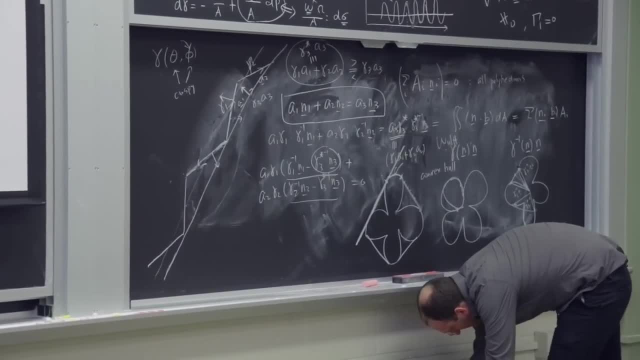 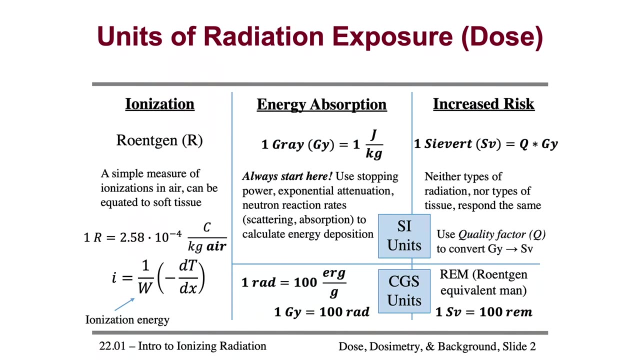 Defense Dosimeter and passed it to one person And we didn't continue bringing it. So I'll bring it to recitation. It's not in my bag. There's the unit of the gray, which is just joules per kilogram, which you can calculate from stopping power or exponential attenuation equations. This: 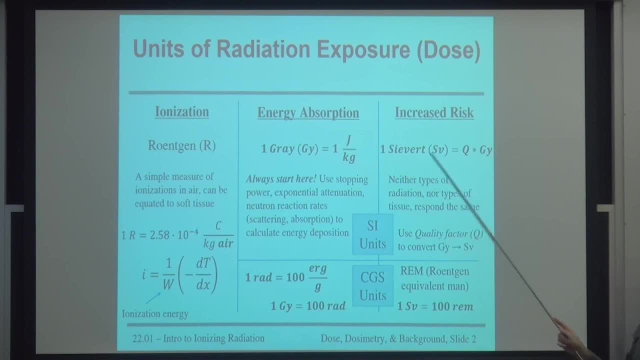 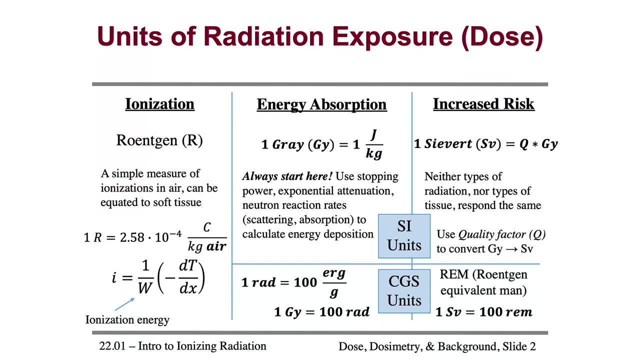 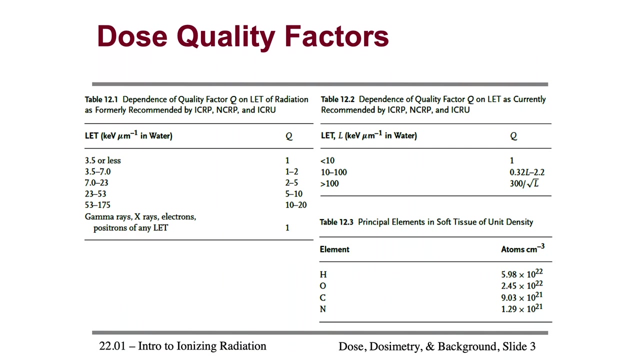 is where you start, because it's how you get from the world of physics to the world of biology, into units of increased risk or sieverts, which is just gray times, a bunch of quality factors which are either tabulated or- I'd like to see somewhat better- calculated. They are calculated sometimes, but by 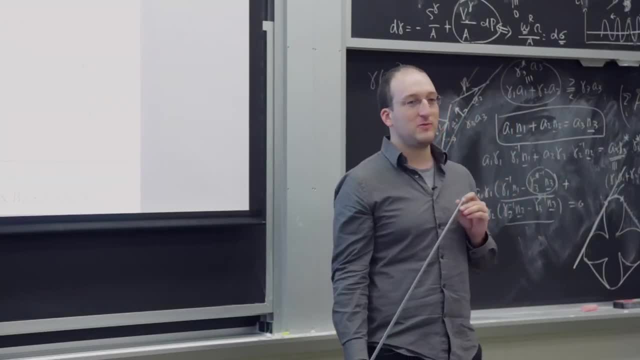 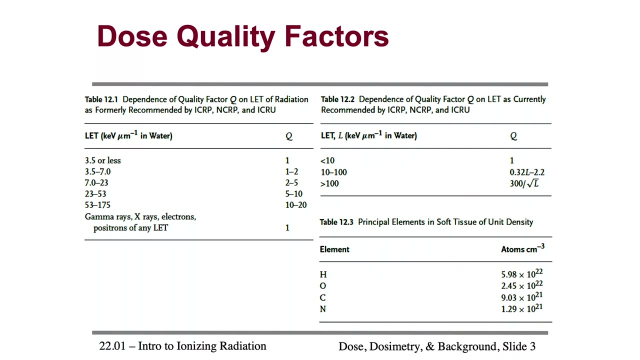 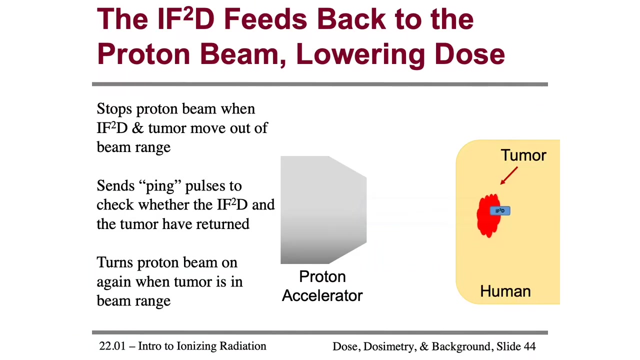 empirical relations, because that's usually good enough. Biomeasurements tend to be pretty sloppy and I'm not that upset that these are empirical relations And I'm going to skip way ahead past the detector stuff. We didn't quite finish up the IF2D idea. I. 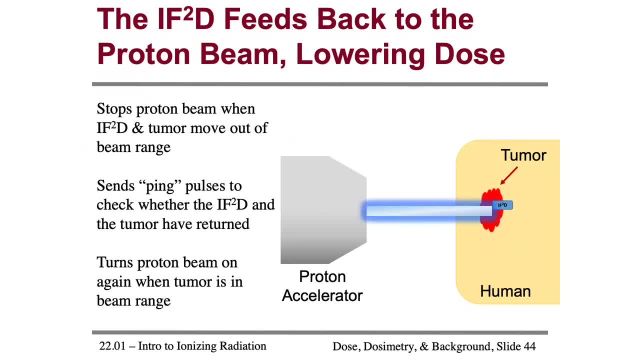 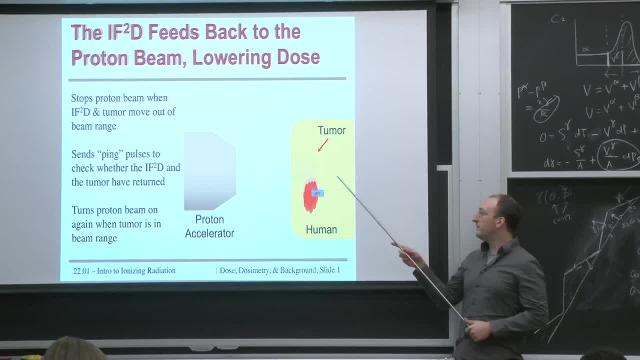 think this is where we ended last time, where we were talking about how do you detect dose during cancer, And I think this is where we ended last time, where we were talking about how do you detect dose during treatment, And I was outlining one proposed way that we're thinking of using this F center-based. 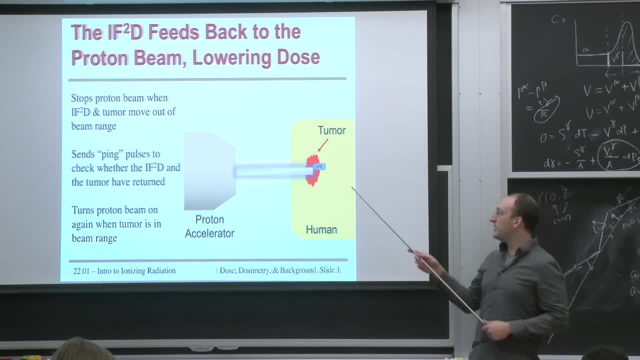 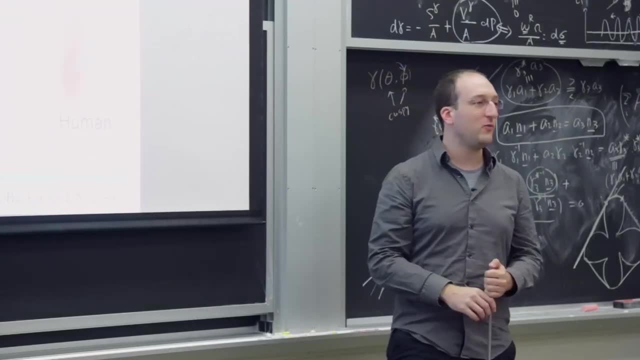 dosimeter which changes color when it gets irradiated. You can implant it in the tumor And as it moves from things like breathing or swallowing you could feed back to the proton beam and only irradiate when it's in range or play nuclear operation and try not to hit the sides. 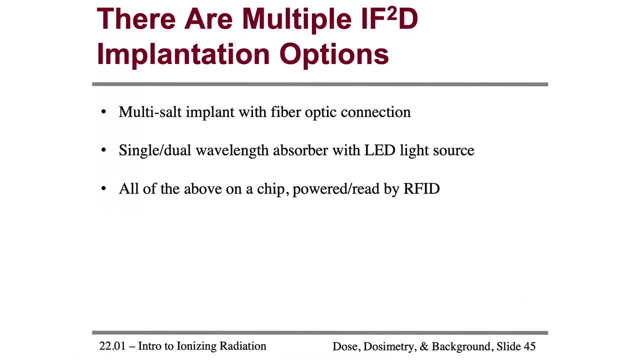 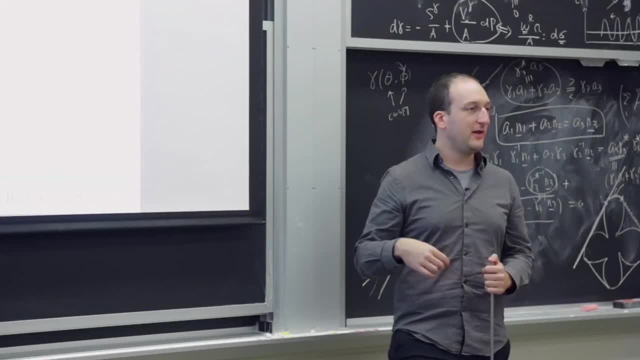 however, whatever you want to do- And there's multiple implantation options for this- We've thought about things like implanting a fiber optic cable into the tumor and then having a port on the side of you that could do some in-body spectrometry, which would be pretty cool. You could also put it. 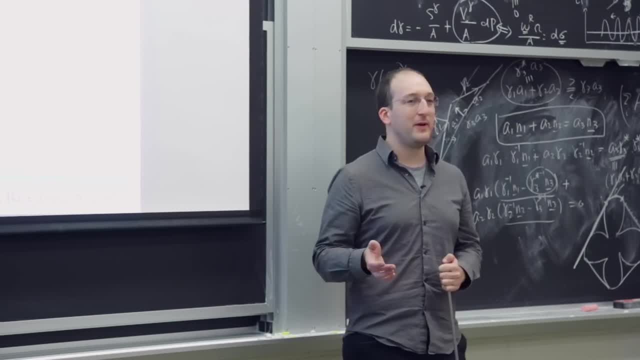 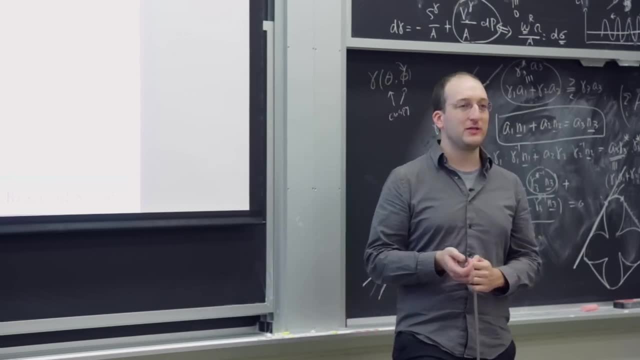 all on a chip. You could have the emitter, either a broadband or single color LED, the F center and the spectrometer all on a chip that's implanted and with RF, with radio frequency power transfer. So you don't need to put a fiber optic port and plug it into the side of you or however it goes. 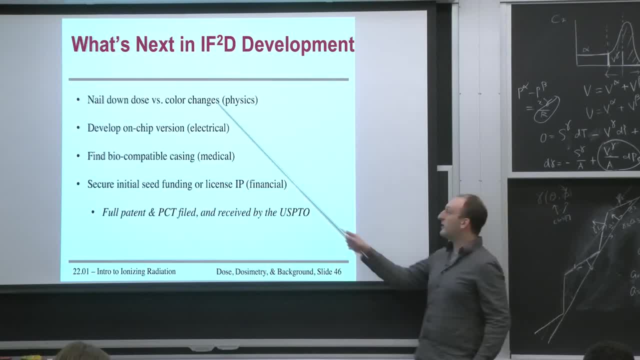 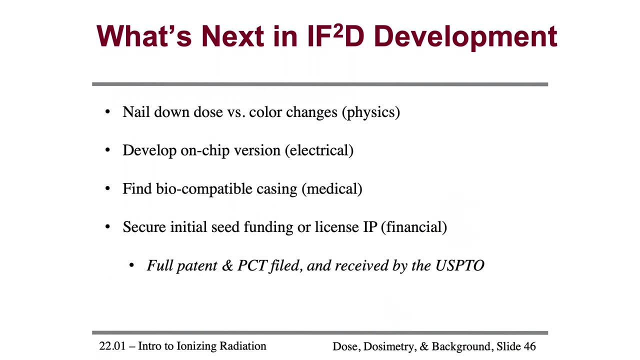 And what we're doing next in this development is nailing down what color change is given by what dose. so the physics develop an on-chip version, find a biocompatible casing. We've done the IP part, which is pretty cool, As you can see, with patent Office at least has taken in the application. 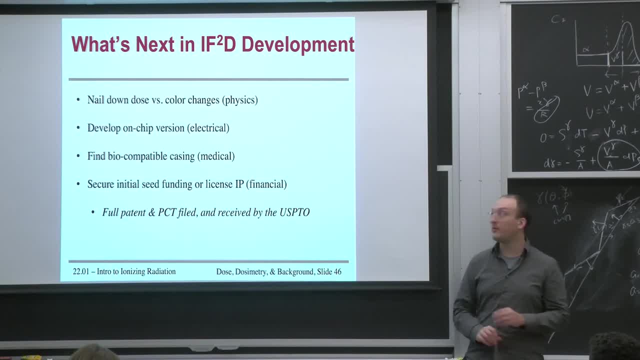 But it's neat that you need to know pretty much everything you learn at MIT to pull off a project like this: from the nuclear physics stuff to the material science, to the 22071 electronics, to the medical stuff for biology, to the financial stuff for econ, In order to pull off an actual nuclear startup. 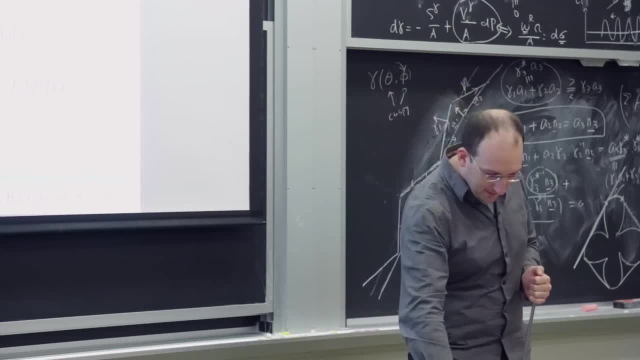 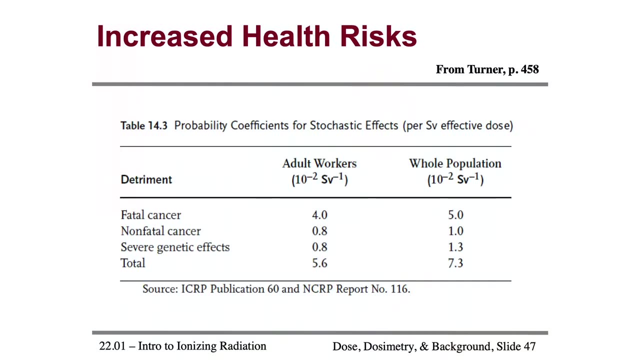 project like this. you need everything you learn here. It's kind of a neat case study. But now let's get back into what does a Sievert really mean in terms of increased risk. It usually means the increased risk of some sort of long-term biological effect. 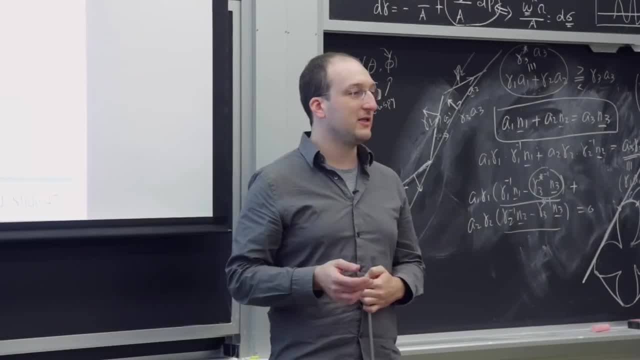 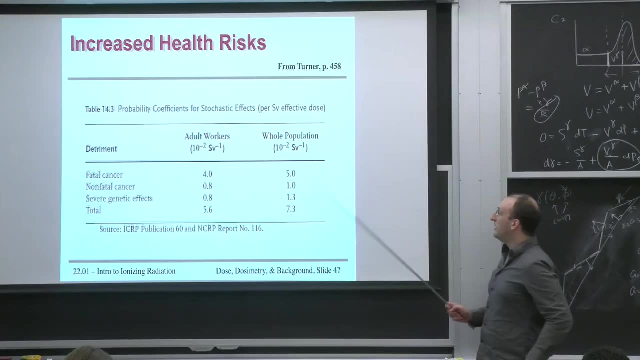 whether it's cancer or some other genetic effects, let's say mutations, anything that would take a while to manifest and would manifest by slow but steady cell division, And if you notice the difference between adults and whole population, let's see. Yeah, so sorry. You can see right here that these are not very much dose, Let's say in a realm of 10. 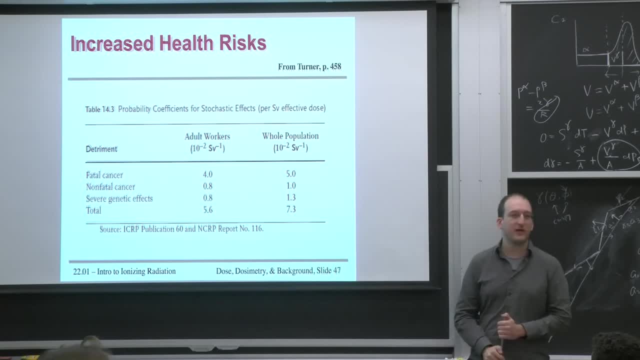 to the minus 2 Sieverts can give you some increased risk for cancer or some other effect. So we're talking like on the realm of 40 millisieverts or so would give you some additional cancer risk. That's not a lot of dose. 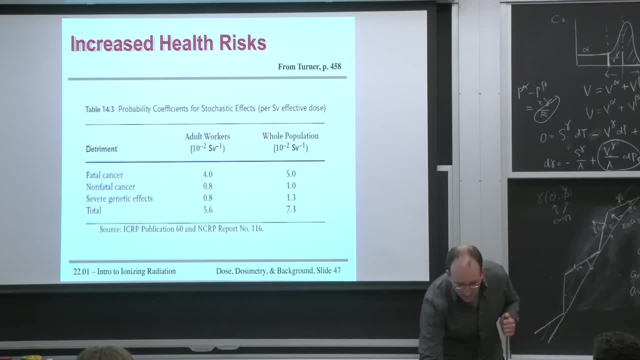 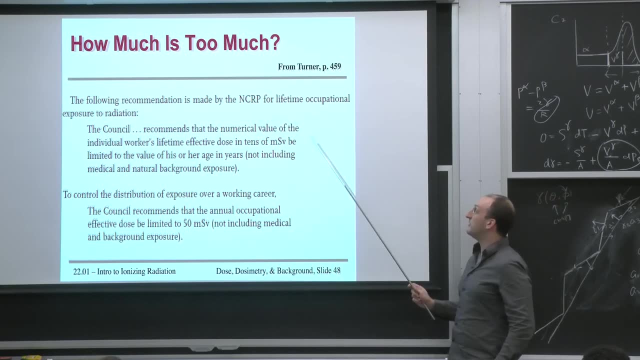 That's up to, about the limit of the occupational dose that you're allowed. So when we talk about how much is too much, I've taken some excerpts from this Committee on Radiation Protection document. This is from Turner, but the entire document, as I mentioned. 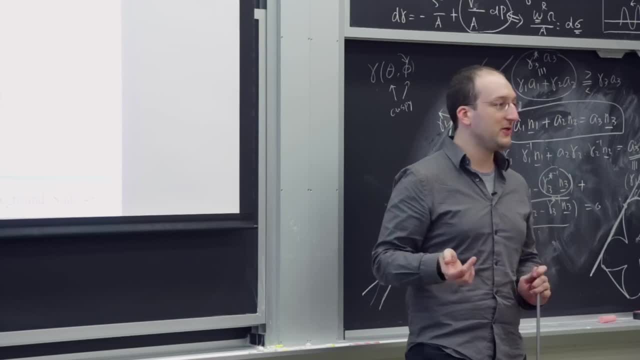 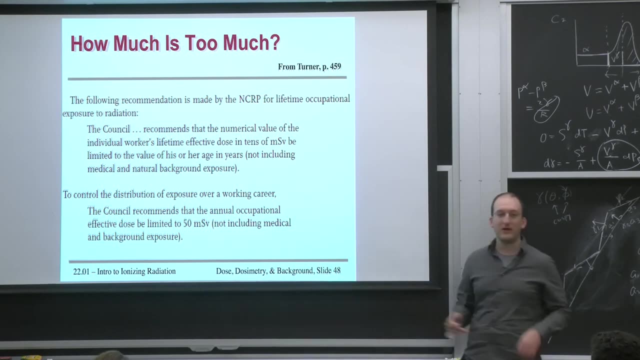 is up on the learning module site So you guys can see the actual verbiage where this is defined. So your lifetime dose should never exceed in tens of millisieverts the value of age in years, which means in some years if you get a little bit less dose. you can get a little bit more dose And still be considered safe or not have any appreciable increased risk, And while you're working you should never get more than about 50 millisieverts in a given year. How is it for radiation workers? 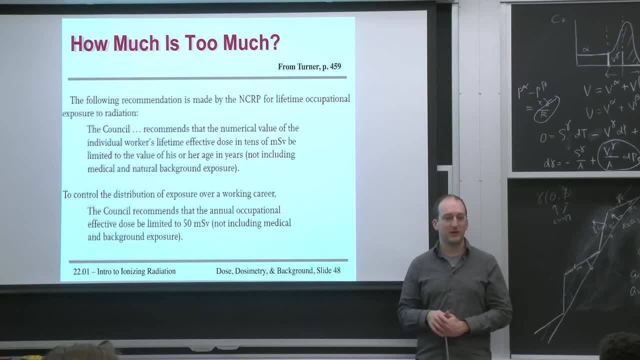 So for you guys, what dose are you allowed per year working at the reactor? 5 rem per year. 5 rem per year, which is 50 millisieverts, OK, awesome. So it's a breakdown for like to your eyes. 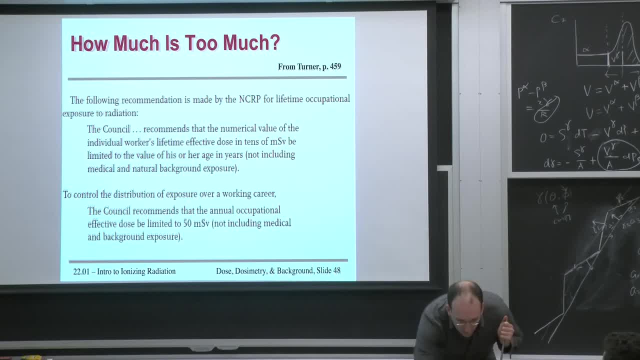 into like a specific organ, but we just care. We mostly care about the blood. Oh, sure, Yeah. So to come back to that, if you're saying that there's actually tabulated differences for different organs, that's where they come from. 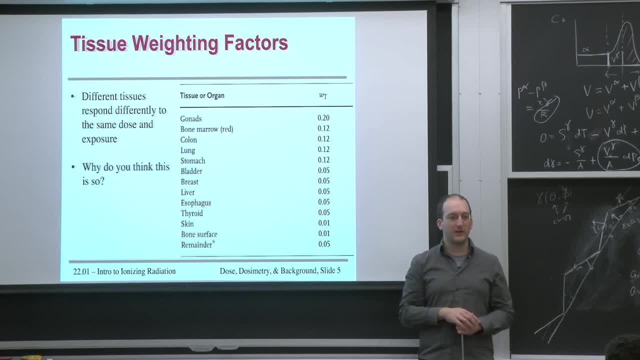 Because you can take- let's say you can take- less radiation to the same organ and get the same dose in sieverts measured in equivalent risk. So I wouldn't be surprised if these are the organs that you're not allowed to irradiate as much. 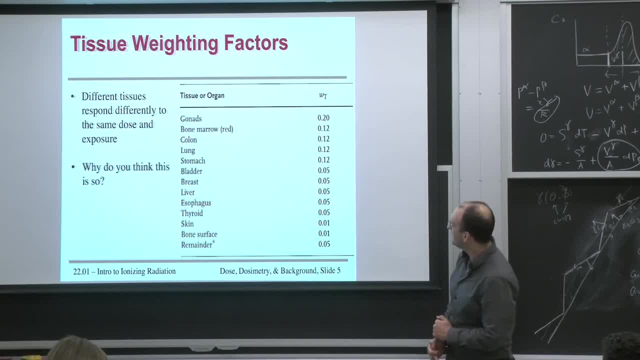 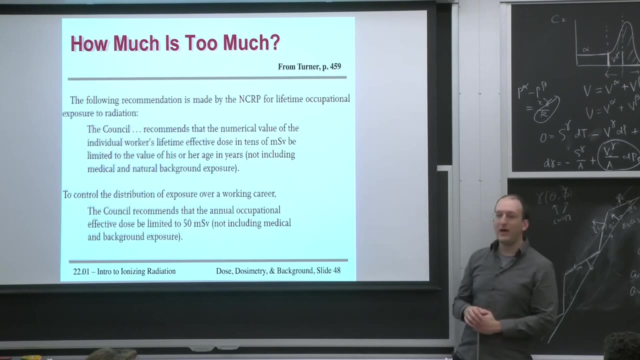 The eye is the only one that they have restrictions on. I'm surprised the eye isn't here. Does it say retina anywhere? Oh, OK, Well, that's just one table, It's not necessarily the complete answer. Yeah, so 50 millisieverts isn't that much. 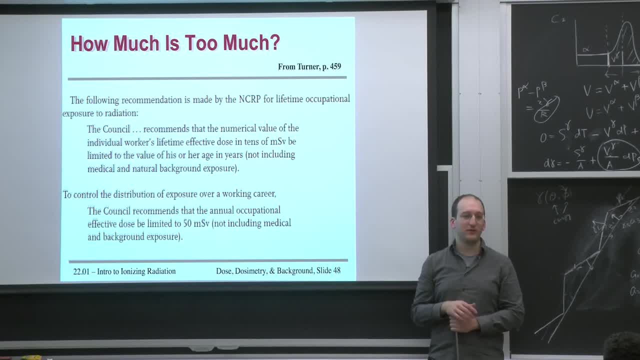 Although, if you think of it in the old XKCD units, a banana equivalent dose- eating a banana- gives you about 0.1 microsieverts. So you would have to get 50,000 bananas in a year- No, I'm sorry, 500,000 bananas- in order to incur that. 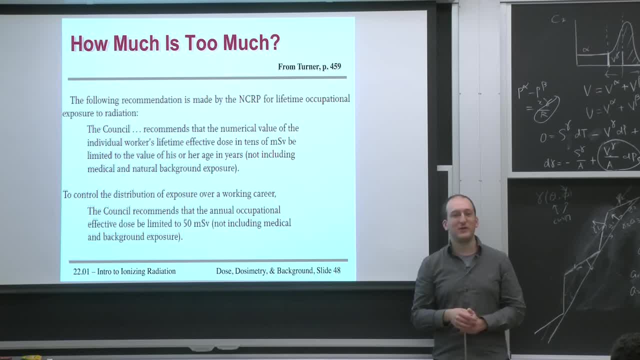 And well, yeah, I was talking to someone at dinner last night about the banana burning experiment, where we measured the activity in becquerels And then we can calculate how much dose in sieverts it would take. And he said how many bananas would. 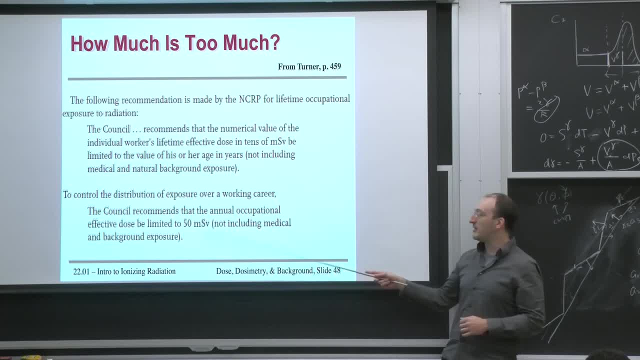 it take to get some increased cancer risk. About double this. It would take about a million bananas to give you about 100 millisieverts. And I said you know what else it would cost? And he goes: 100 millisieverts, no shit. 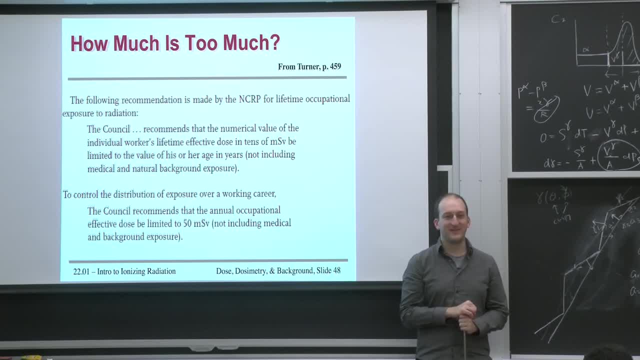 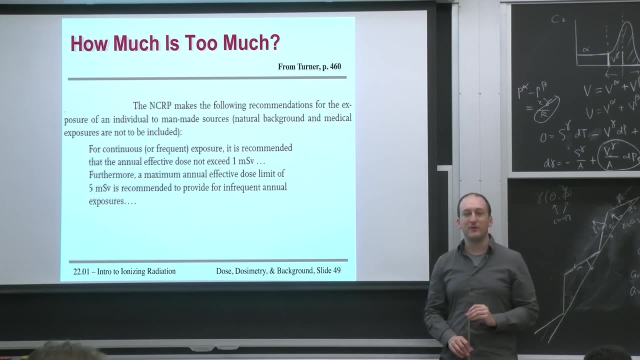 And I said that's right. Yeah, Yeah, See, Totally didn't plan that, but it just worked out that way. Yeah, And then how much is too much? Let's say, for the general public, for background, for excluding things like natural background. 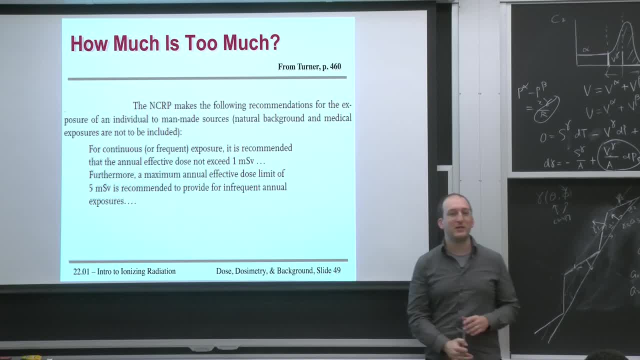 and medical exposures. you're not supposed to get about more than one millisievert just walking about outside, And you don't tend to get that much more. Now why does anyone think? why are medical exposures not included, despite them being pretty radioactive procedures? 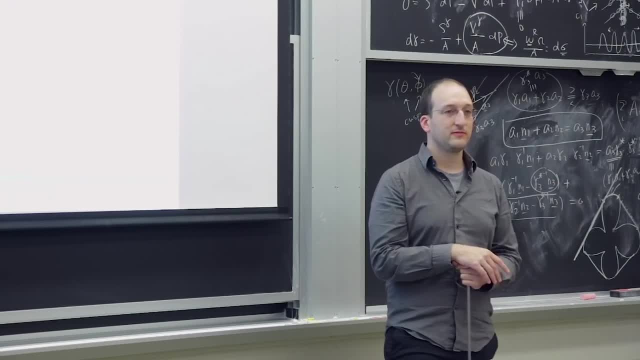 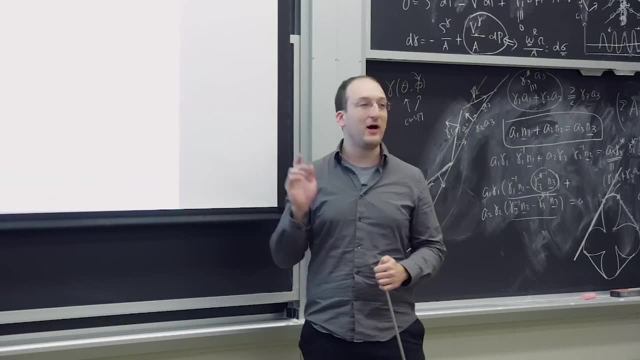 Yeah, Because they're very targeted. They are targeted, They are targeted, And so they could give a lot of dose to certain organs. But the amount of dose isn't necessarily why we don't count medical procedures. Anyone have any idea? Yeah, 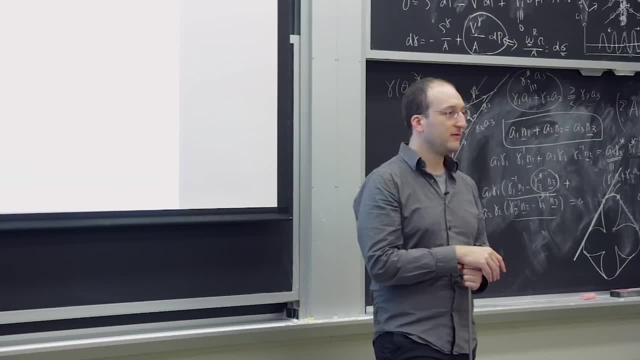 Is it because you should be wearing a lead vest if you're going to get an x-ray? In some cases you'll get, like, if you go to the dentist you'll get a lead x-ray, But let's say you get a huge chest x-ray, right? Why don't we care that a chest x-ray is way more than you get? Because these things tend to save lives. So you're absolutely willing to get extra radiation exposure that may have a delayed effect if the immediate effect is to save your life. 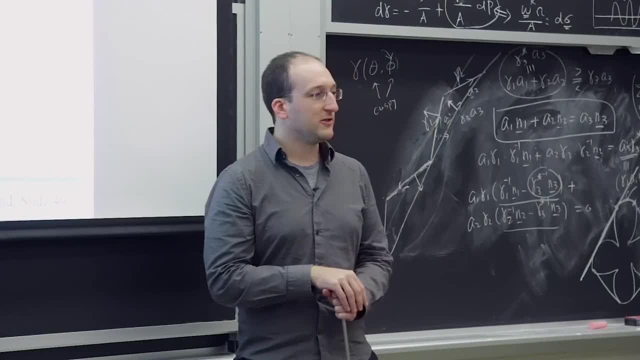 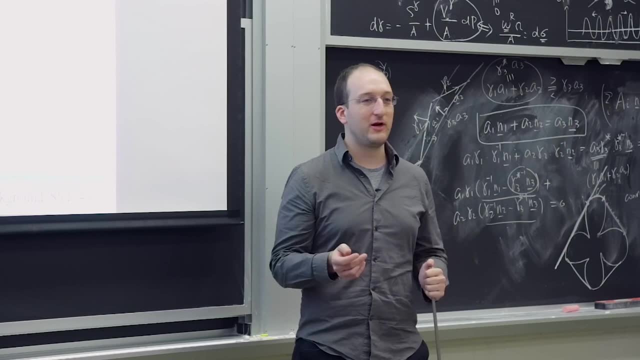 You got a question. No, OK, yeah. so we don't count medical things because chances are you're doing them to improve or save your life. So what's a little bit of radiation compared to, let's say, finding the blood clot or the aneurysm? 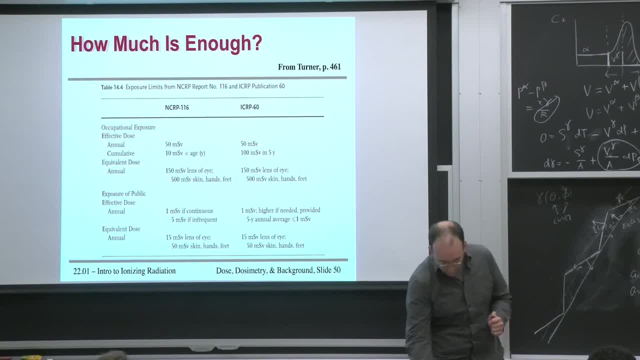 or whatever it would take, And then how much is enough? This is the table that you're familiar with. Yeah, they actually talk about the lens of the eye And that's a heftier dose, But also the lens of the eye is not a very massive organ. 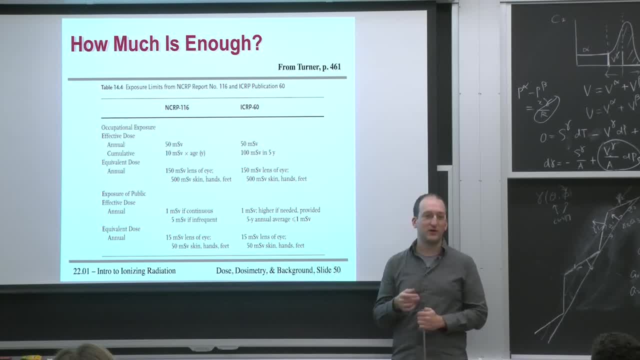 So this would mean: do not stick remaining eye in neutron beam, right, Yeah? Or you've seen that sticker: do not stare into laser with remaining eye, Yeah. the same goes for the neutron beam ports coming out of the reactor, yeah. 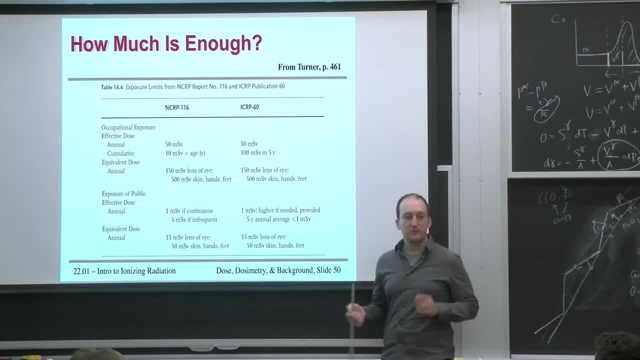 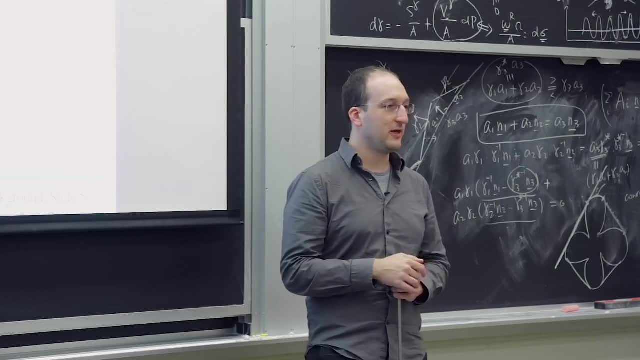 But the lens of the eye can take a fair bit more dose per unit mass than the whole body. The lens of the eye is not a particularly fast developing tissue. It can cloud up with an insane amount of radiation exposure That would take a lot more than 150 millisieverts to do. 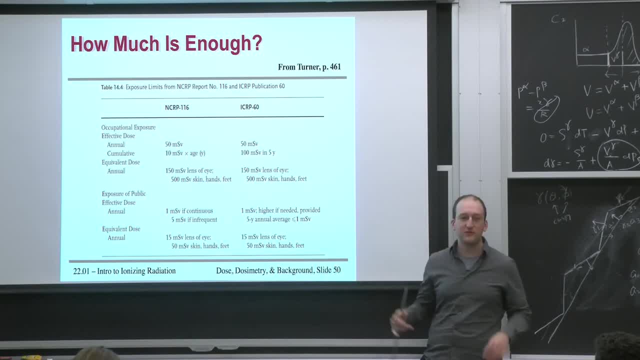 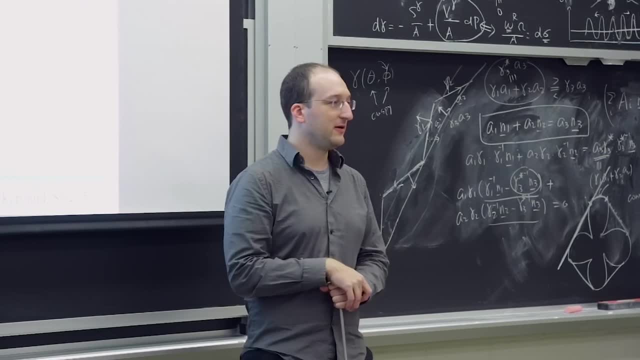 though, And then things like 500 millisieverts for skin, hands, feet- pretty much just groups of muscle, bone and dead skin that aren't really not much is going on biologically. Blood's flowing through it, but that's about it. 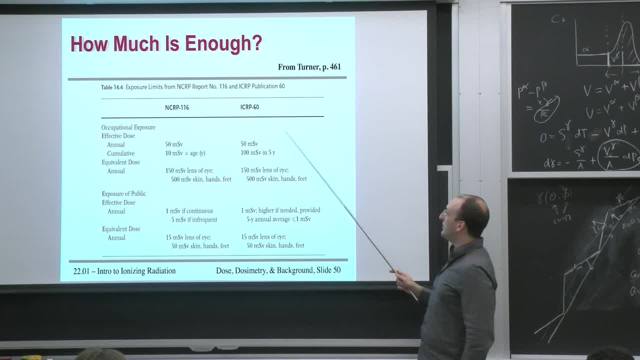 And notice that the regulations, They do differ a little bit, but on the whole they're fairly similar. Same for the eye, same for the feet, same for the ear. Cumulative is a little different. This says 10 millisieverts times age. This allows you a little bit more. Whichever recommendations you follow, they're all pretty similar, And our knowledge of how much dose leads to how much risk hasn't changed a ton in the last decade or so. There's been all sorts of arguments for or against it. 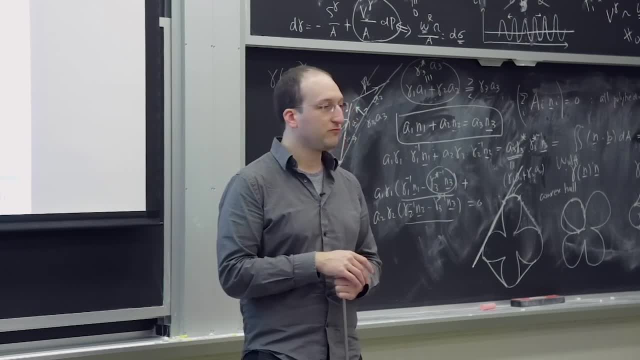 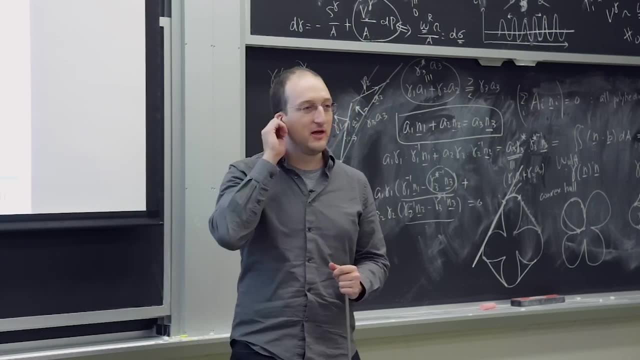 Has anyone heard of this LNT or linear no-threatening Threshold model of dose versus risk? This is something we'll talk a lot about on the last day of class. This is the theory that the amount of risk versus the amount of dose is linear. 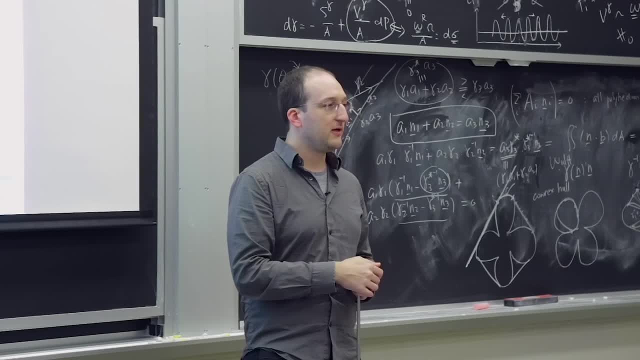 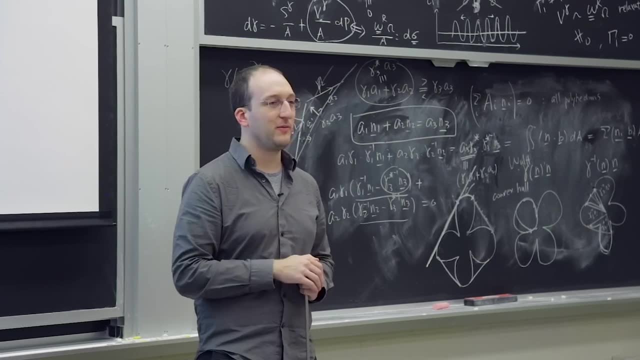 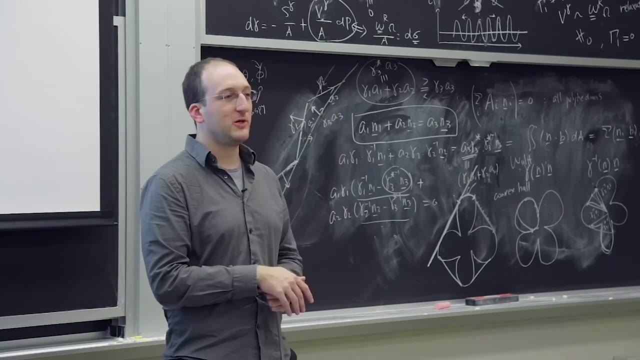 And no threshold means that every little bit of dose gives you additional risk. This is not supported very much by science. Actually, I'd say it's not supported by science. The converse argument is also not supported by science. We just don't have the statistics at super low doses. 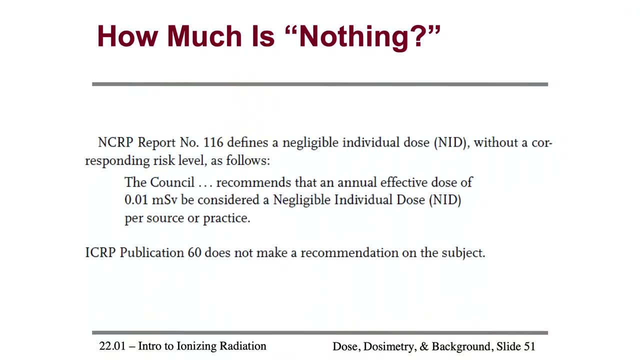 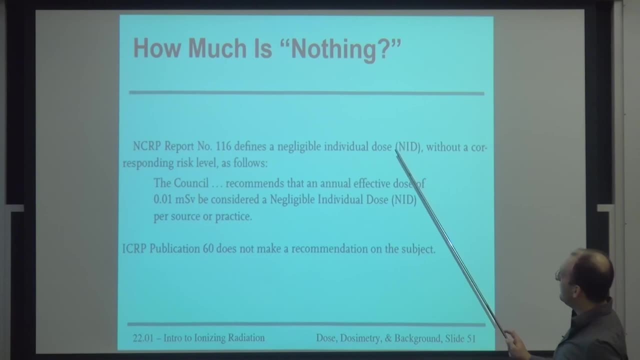 to say what happens, But the official recommendation is that there is a unit of dose that we define as nothing, And it's 0.01 millisieverts, about 100 bananas per event. let's say Yeah. where does it say? 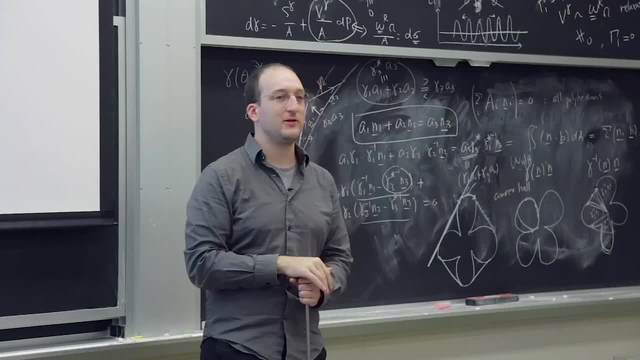 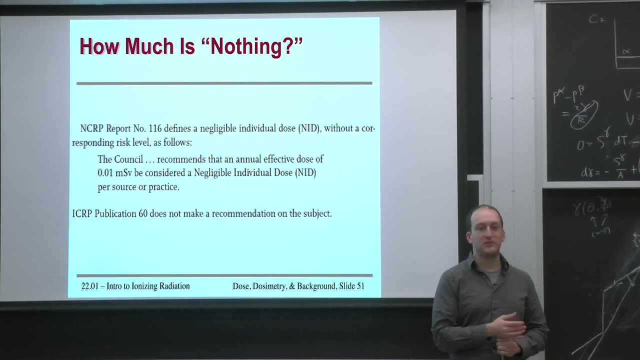 Yeah, per source or practice. So eating 100 bananas in one sitting is considered to give you zero additional risk according to the official guidelines. So the guidelines put in place do not follow the linear no threshold model, but anyone that would claim that one or the other model is absolutely. 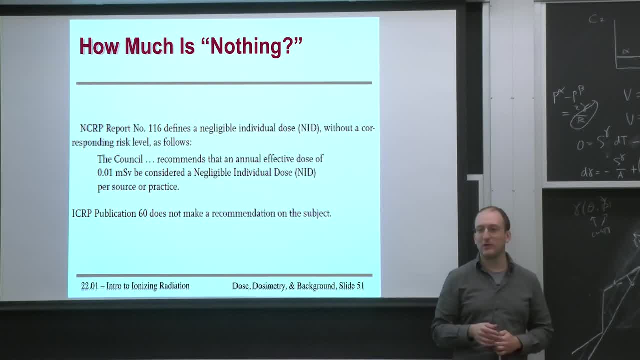 correct, has either got a huge sample size of people that we don't know about or is probably extrapolating beyond what the data will tell them. So you'll see this argument flaring up quite a bit. For the last day of class. we'll have you read some arguments. 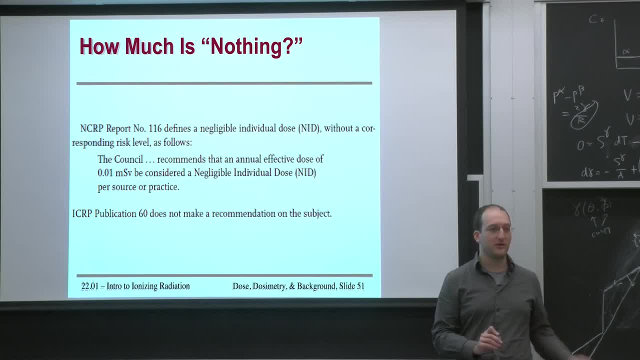 for and against the linear no threshold model. that aren't just blogs on the internet, but they're actual published articles that have passed peer review And it's really hard to tell exactly what's going on at low doses. But meanwhile, Yeah, Meanwhile, let's focus on what you do: get that we can measure. 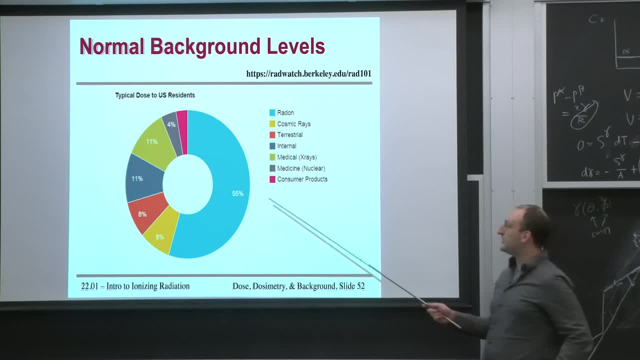 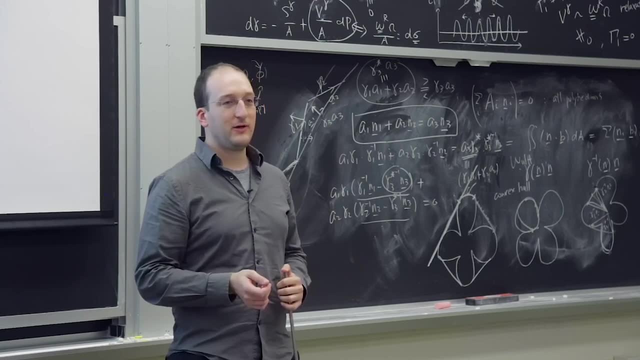 The actual contribution from background levels is about 50% radon. This is a natural decay product of radium. It's just everywhere. It's here right now. It's all through the atmosphere. This is why you want your basement to be rather well ventilated, because it's 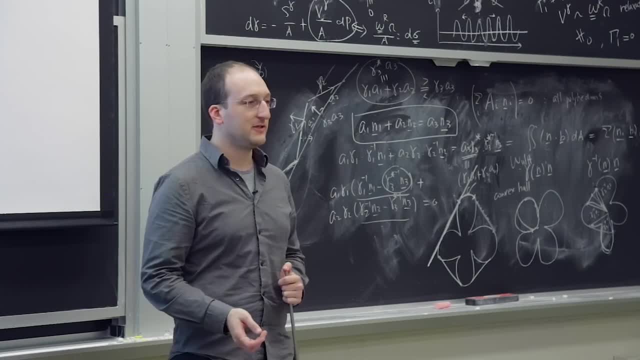 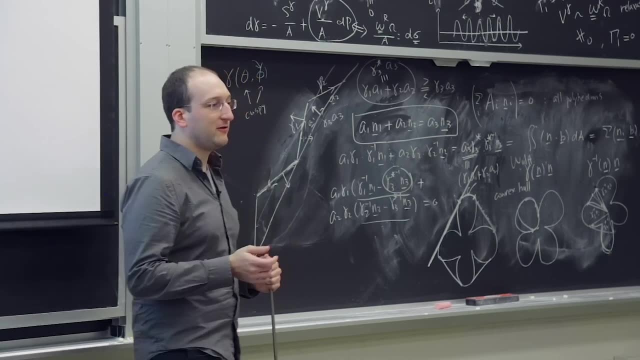 a heavy noble gas that accumulates down in unventilated basements. So you don't actually want your house to be sealed up super tight because you can have radon accumulation, especially if you happen to live near a granite deposit or on granite bedrock. 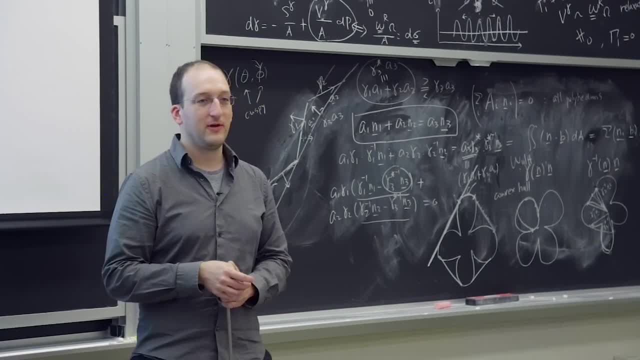 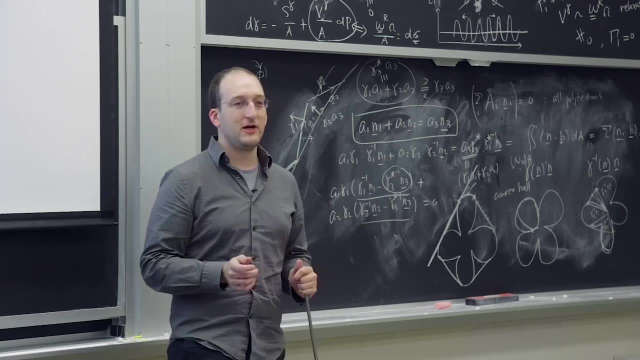 which, like everyone in New Hampshire does, radon levels are a little higher. There's actually a story about a guy that used to work at a nuclear plant somewhere in Pennsylvania- I don't know where, But he lived on top of a pretty good granite deposit. that 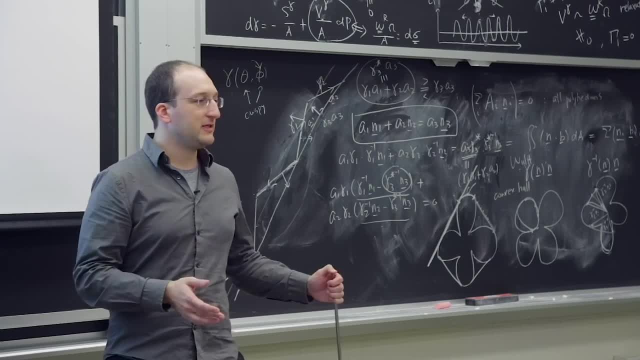 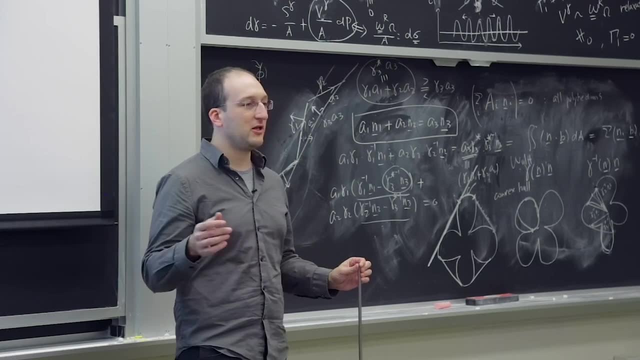 was a few parts per million radium ore. So the radon levels in his house or in his basement were much, much higher than would normally be allowed for background, And this guy used to set off the radiation alarms coming into work. Then he would breathe the nice clean, radiation-free air. 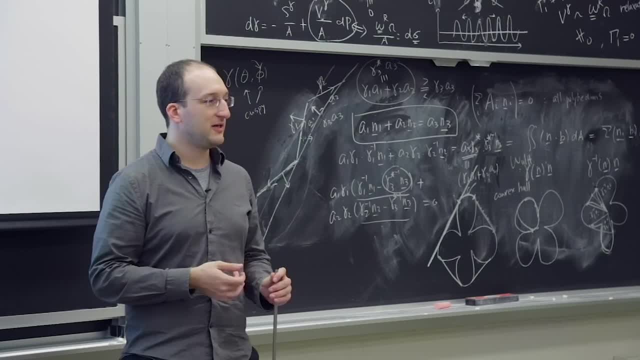 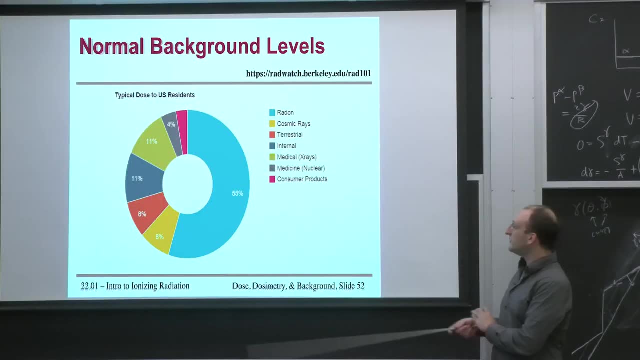 in the plant and go out without setting off the alarm. Eventually, something had to be done. I don't actually know what was done, But if any of you can find that original story, that'd be pretty cool. Cosmic rays: another source that you can't shield from. 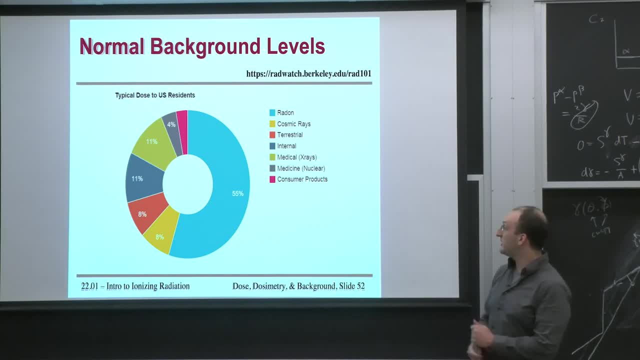 is about another 10%, And we'll talk a lot about where these things come from. Terrestrial radiation- well, we'll count that as stuff in the soil. stuff in the cinder block Wood happens to be a fairly radioactive substance. 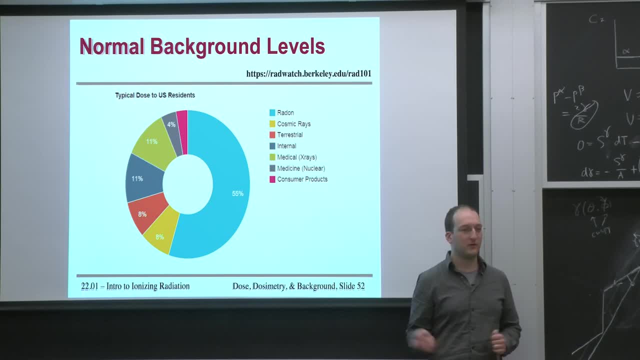 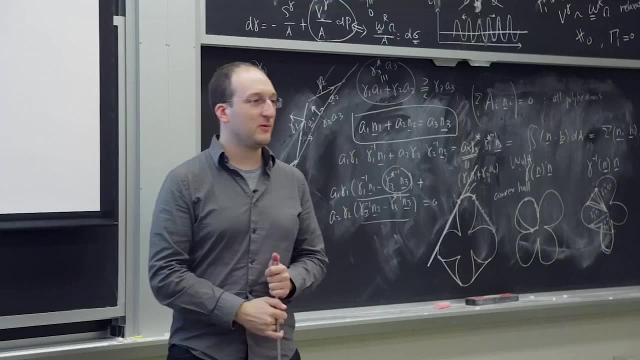 pound for pound, But it's not very dense compared to things like brick or banana ashes. It's probably about the same as wood Internal coming from you. You'll have this on problem set number 8, because you all now know your internal radioactivity. 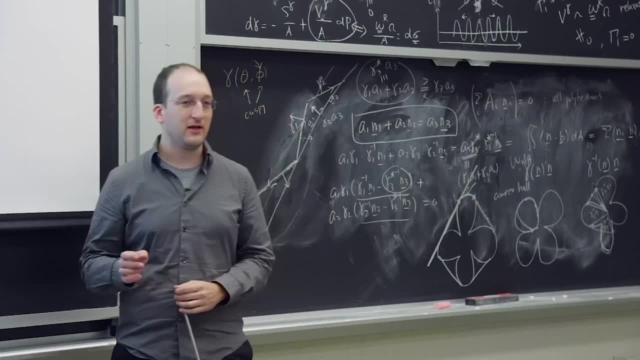 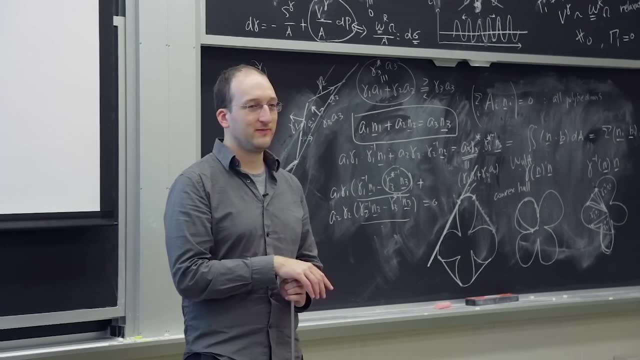 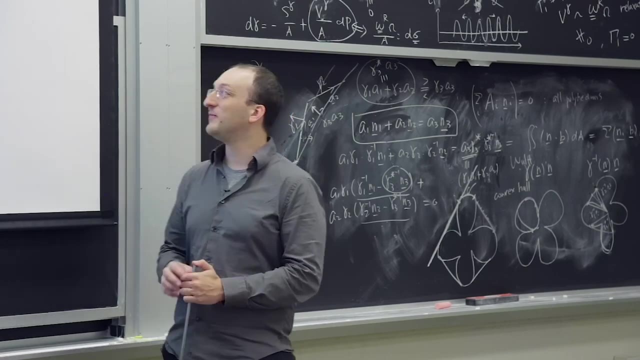 thanks to going to environmental, health and safety. Did anyone see anything disconcerting in your spectra other than a tiny little potassium peak? Anyone, I'd say, oh, it's too bad, But that's great, You know, especially for you guys that work at the reactor. 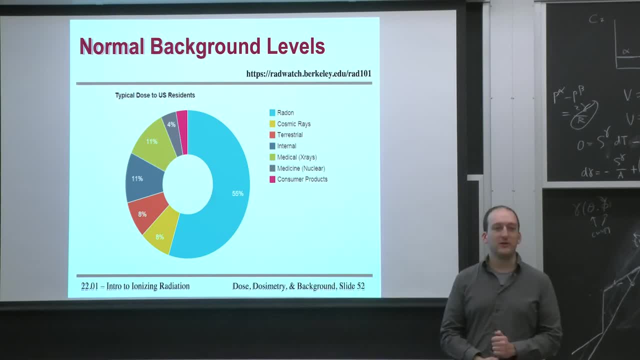 Medical x-rays. it's assumed that everyone gets a couple of these a year. You all go to the dentist and look for cavities, You break something, you may get an x-ray of your hand or foot And this is, let's say, an average amount. 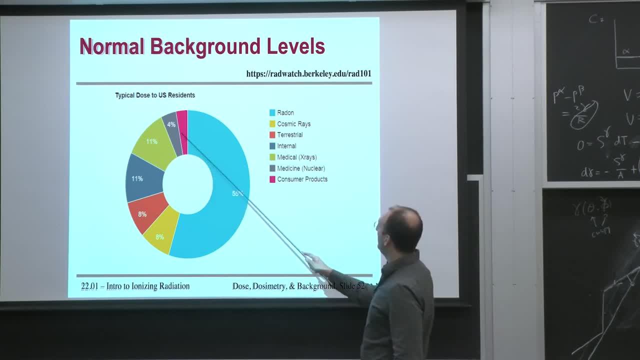 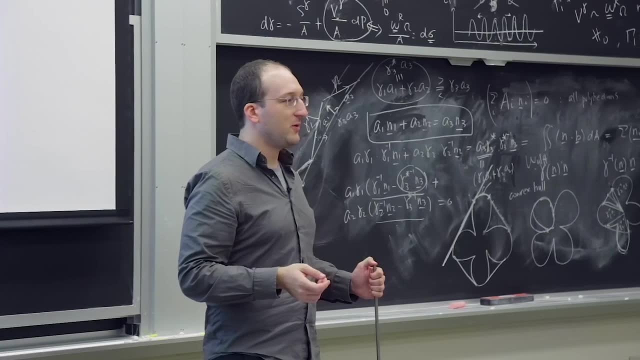 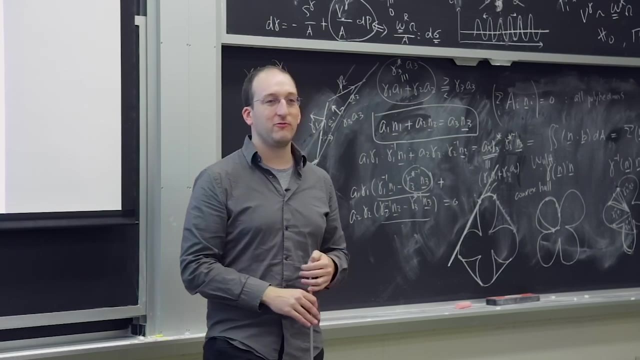 of medical x-rays And the little bit of stuff left over consumer products. This isn't counting things like Fiestaware, those orange glazed plates and bowls that were painted with a uranium-based neon orange paint. So we also don't tend to drink from revigorators anymore. 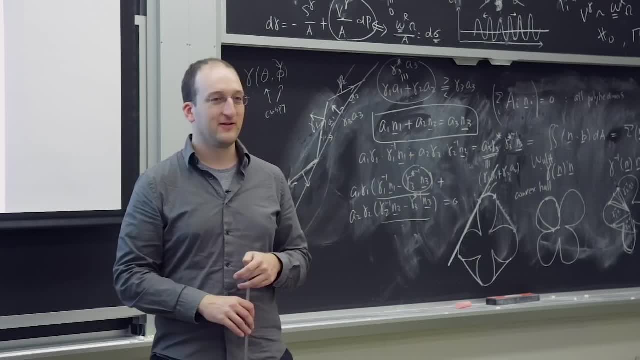 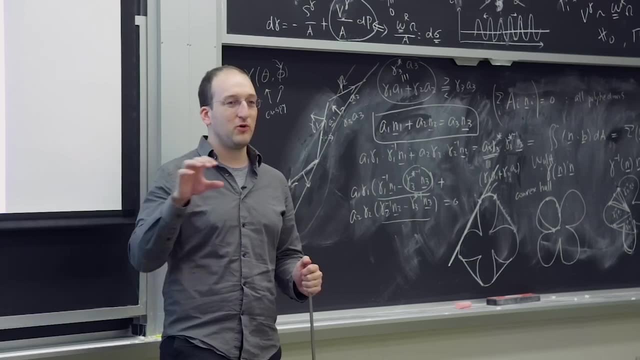 Has anyone ever seen or heard of a revigorator? Oh yeah, It was like the 50s or 60s Or even earlier. yeah, So like back in the 20s, people would put radium ore in these containers and pour water in it and say: 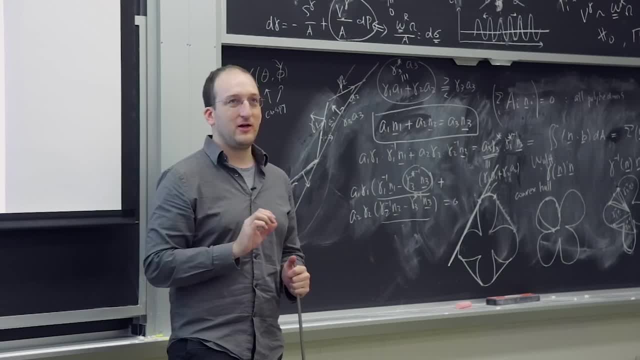 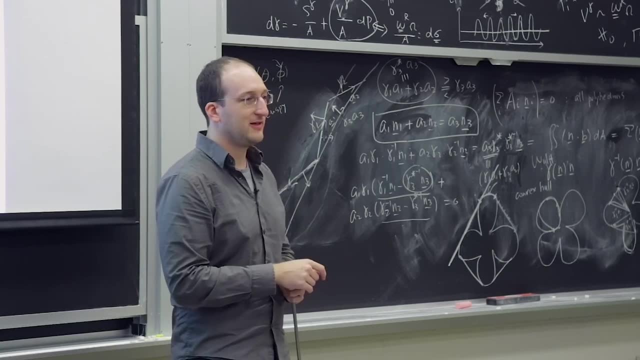 natural radioactivity gets in It. cures like croup or the Jimmy Legs or a stigmatoid rheumatism or whatever other quack diseases there were in the 20s. You can still find them on eBay. That's not accounted for in today's consumer products. 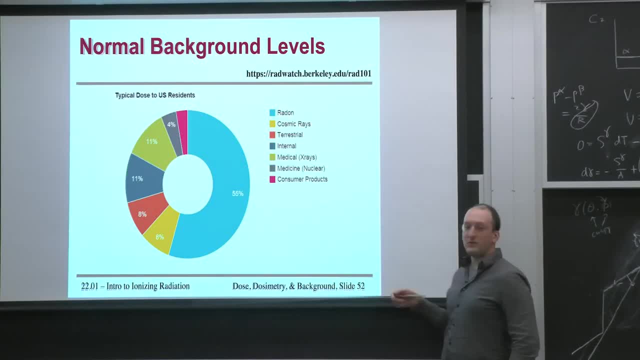 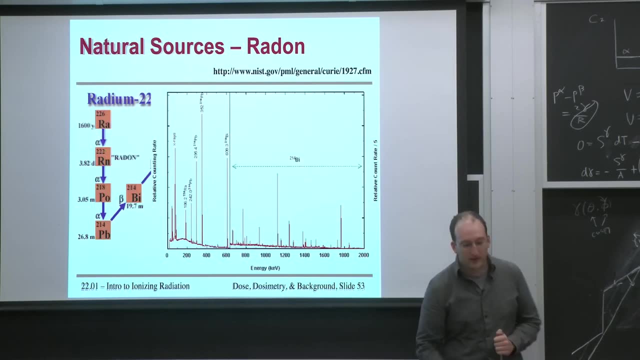 But this all accumulates the amount of dose that you tend to get on your own. You might get a couple millisieverts a year of dose just from background, especially depending on where you are And the big one whose spectrum I think you're all familiar with by now. 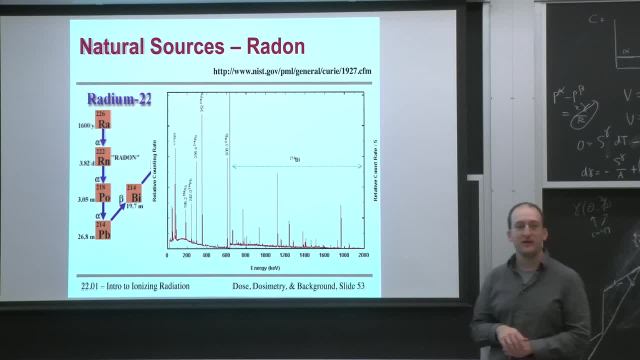 is that of radon, because we saw most of these peaks in the bananas. Anyone have any idea why you would find so many radon decay products in bananas, Given that radon's everywhere. we did notice elevated levels of, specifically bismuth-214. 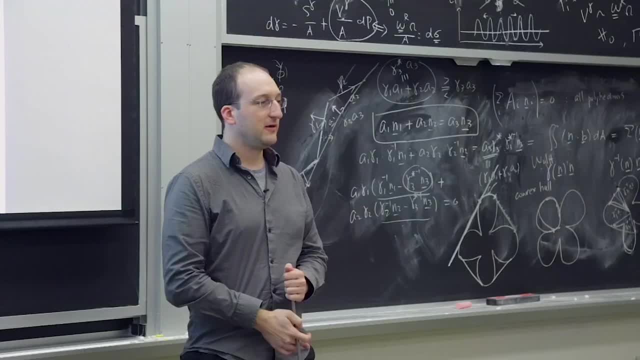 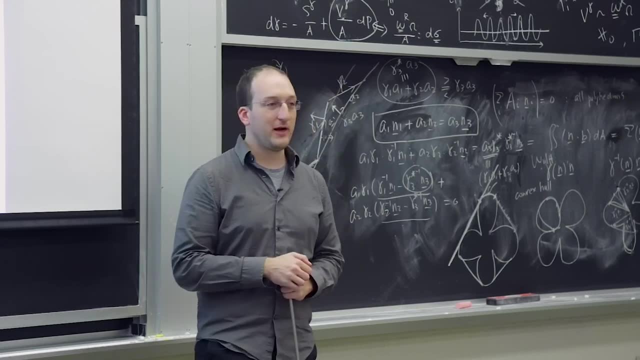 and actinium. I think 228 was the isotope we saw. Where would those come from? The what, Absolutely, yeah. Whatever radium's coming out from the bedrock, that radon has to come up through the soil If it happens to decay in the soil. 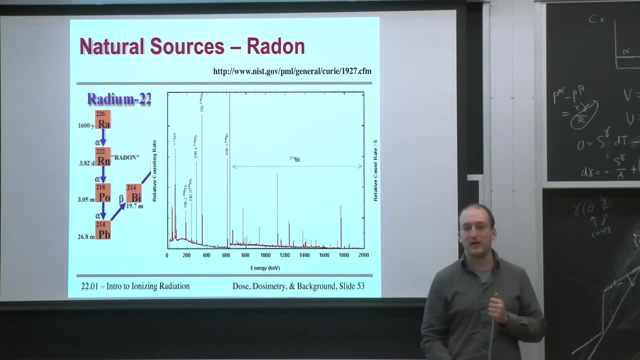 it makes lead, bismuth, polonium, other heavy metals that are uptaken by the plant's tissues. In addition, radon daughter products can plate out on the leaves themselves, So this is one of those reasons that smoking is such a bad thing to do. Aside from the chemical effects. you have giant fields of high surface area tobacco that you then concentrate and dry up into these tiny little sticks. You have an enormous amount of leaf surface area and dry vegetation that has uptaken all these radon daughter products. 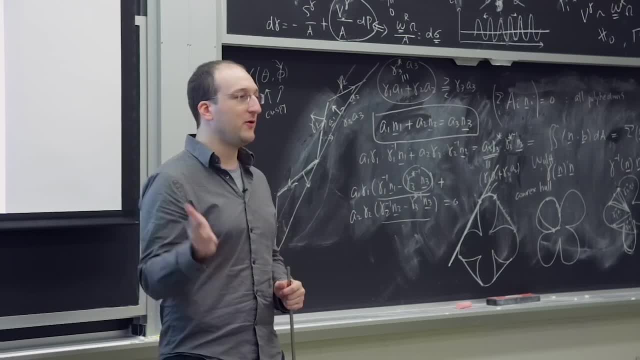 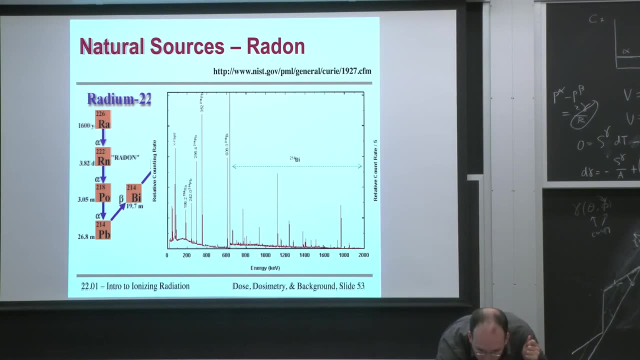 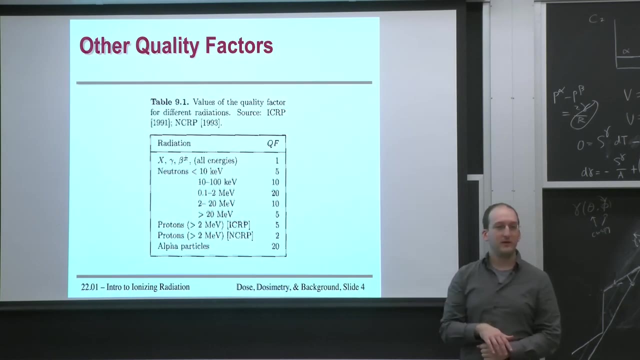 So most of the dose you get from smoking is lead, bismuth, polonium, actinium, radium, Alpha emitters, as we saw last time. to remind you guys of the quality factor for alpha particles, it's as big as it gets. 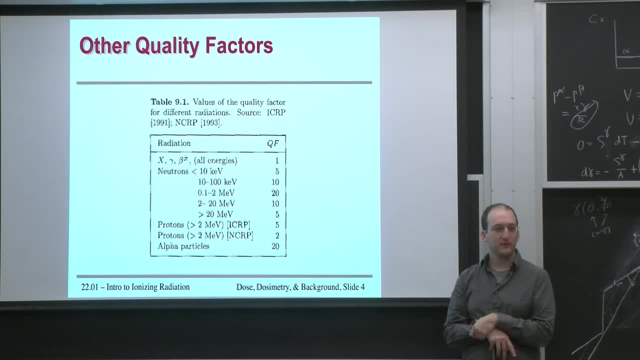 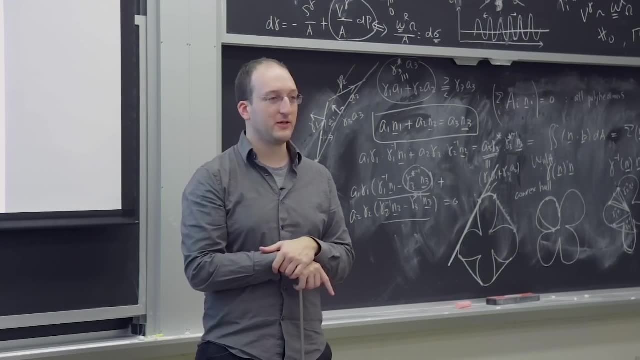 Anyone remember why that is? Why are alphas so damaging if they get into your tissues? Because they're big. MICHAEL SHORTENBERG- They are big, So they have high mass and Short range. MICHAEL SHORTENBERG- Short range. 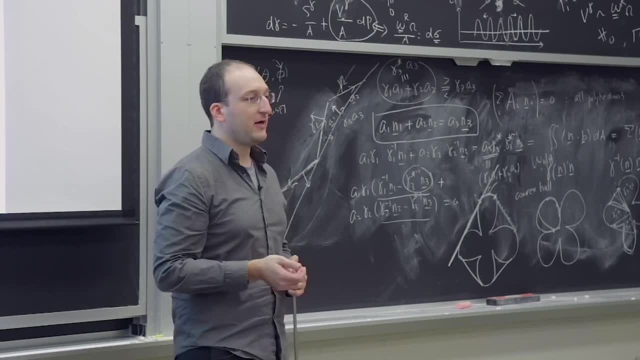 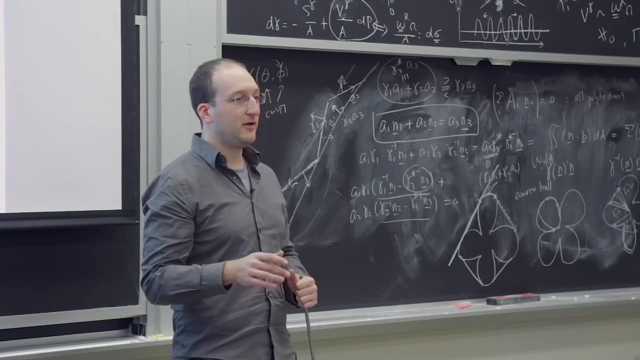 From their high charge, high relative charge, They have quite high stopping power And they will deposit a lot of energy very close to where they are emitted. So their range is very small, so that armor-piercing bullet analogy kind of comes to just an armor-piercing bullet. 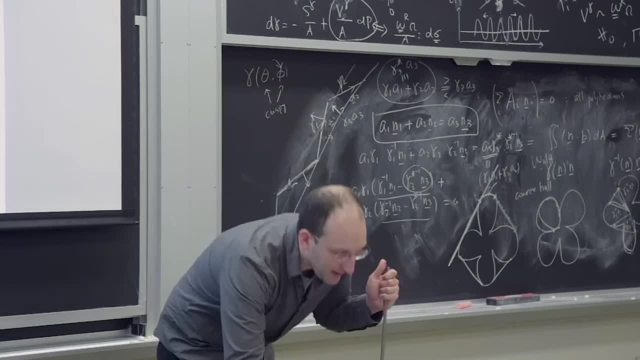 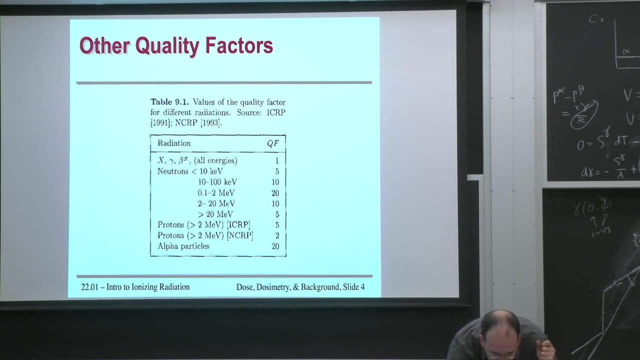 that explodes right out of the barrel of the gun And they do quite a bit of radiation damage. Let me jump back to the right slide without inducing a seizure. I think we've looked before at the radon, So radon decay chain. this is a simplified version. 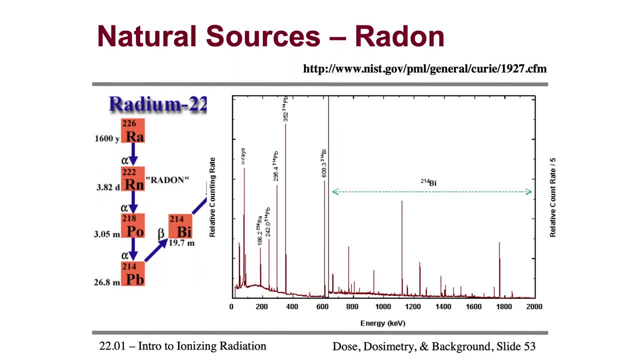 because there are different branches or different possibilities for decay, But some of them have extremely low percentages, So this one's simplified quite a bit. But whenever radon decays it gives off a bunch of alpha and beta emitters that last anywhere from minutes or seconds to days, and so 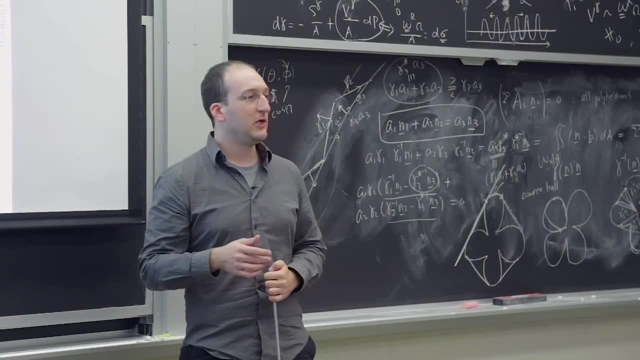 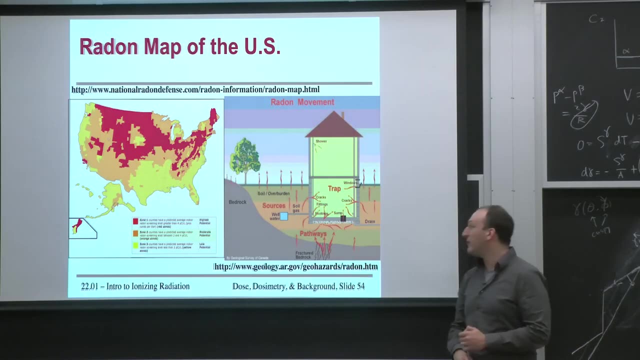 So they'll give off. for every radon atom that you absorb, you end up getting four or five alphas and betas, depending on how long it stays into your system, And then mapping out Radon. in the US you have quite different amount of radon dose. 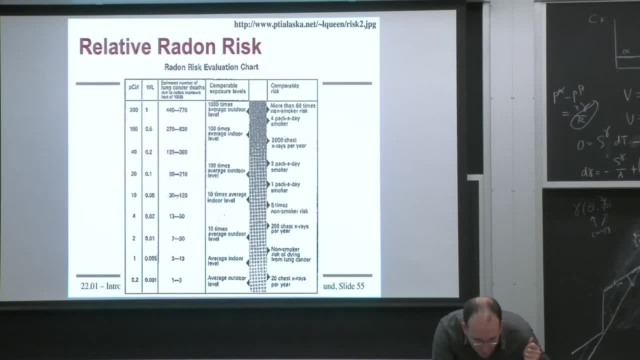 depending on where you are, And I wanted to skip ahead and overlay a couple of maps of the US. So this is a terrestrial. Oh, I'm sorry, that's the wrong one. Let's just look at this one. Anyone notice any patterns here? 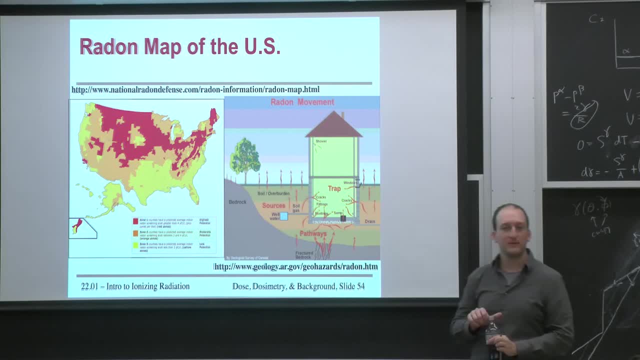 Where do you tend to get the most radon? What sort of features would one live near when you get a lot of radon dose? Mountains- Mountains which tend to be made of rocks, which tend to contain a lot of radium. 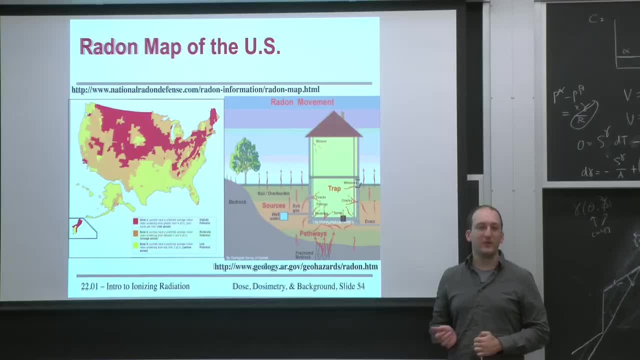 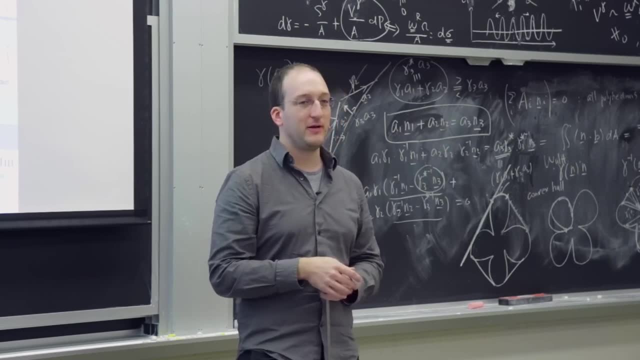 Especially granite and other such rocks. The Conway granite, named after up in Conway, New Hampshire, is about 52 parts per million uranium or radium, So it's a fairly toasty rock. You can actually tell that, you know. you can tell there with your Geiger counter. 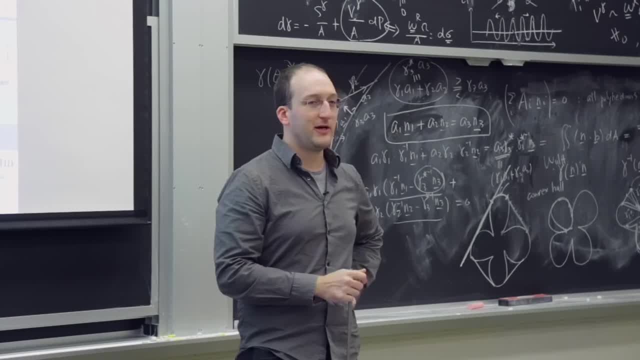 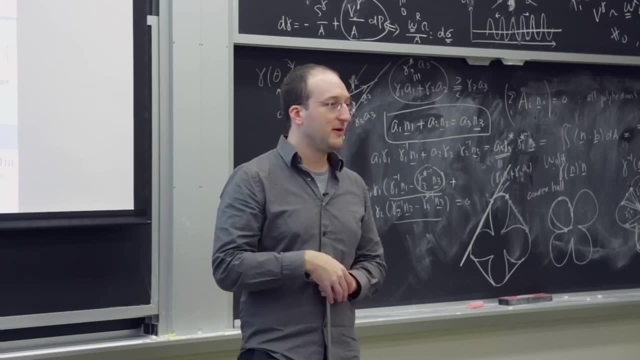 if it's count long enough that there is a little bit of radioactive ore And that Conway granite Not nearly enough to matter at all and certainly not enough to stop you from making fancy kitchen countertops. But I wonder if folks would buy those. 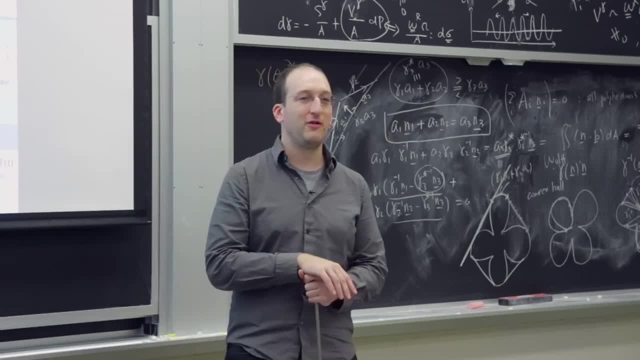 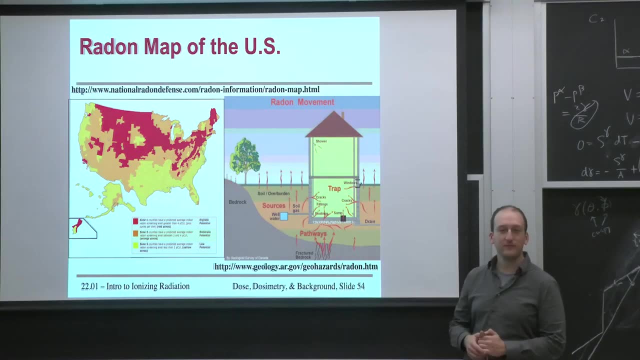 if they knew that there was 52 parts per million of something with a half-life of 9 billion years, I somehow think it would matter to people, but it really doesn't. They put the radiation symbol on it to break it. Yes, engrave that right. 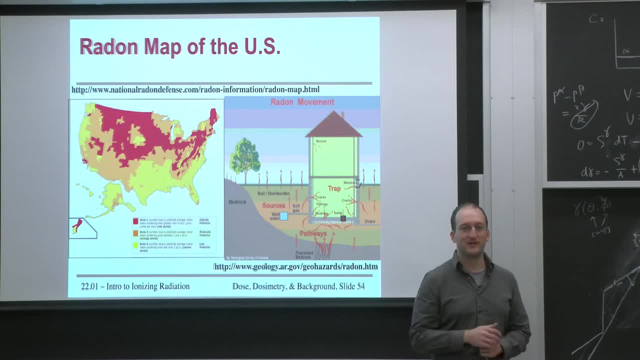 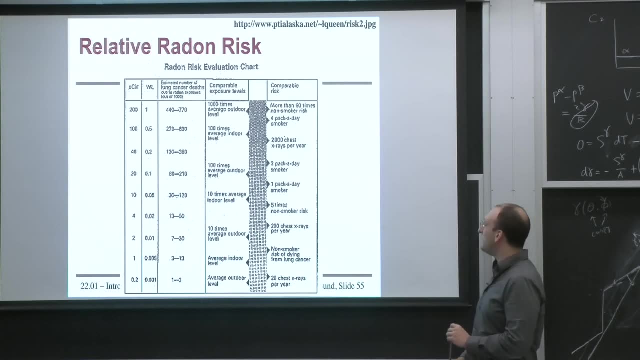 If we made the radiation symbol a little induction stove, that would be pretty slick, Yeah. And then, in terms of relative radon risk, how much actually matters? I like this graph, Despite being difficult to read. it actually shows how much the average indoor level compares. 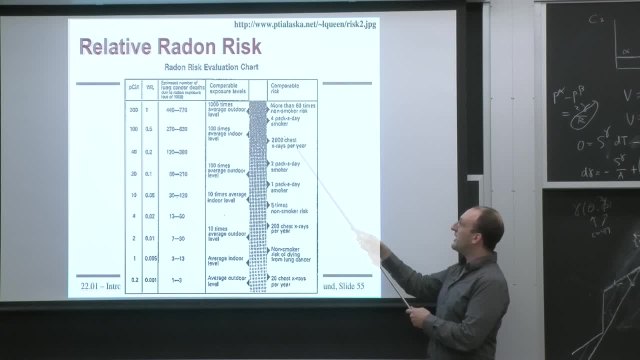 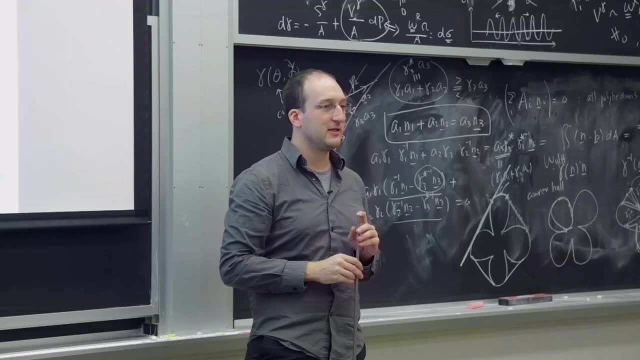 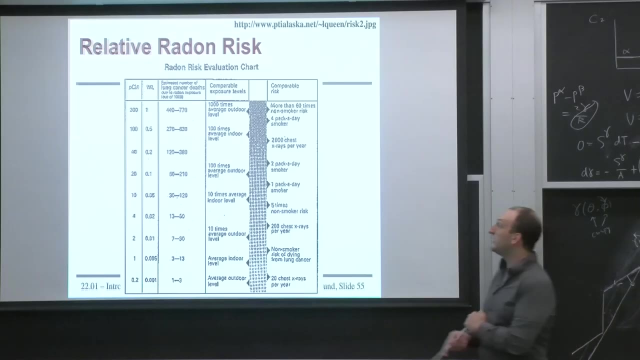 to all the different things you could do, like getting 2,000 chest X-rays per year versus 100 times the average indoor level. That's about what I heard that fellow in Pennsylvania had is like 180 times the normal radon levels from living underground on this giant granite deposit. 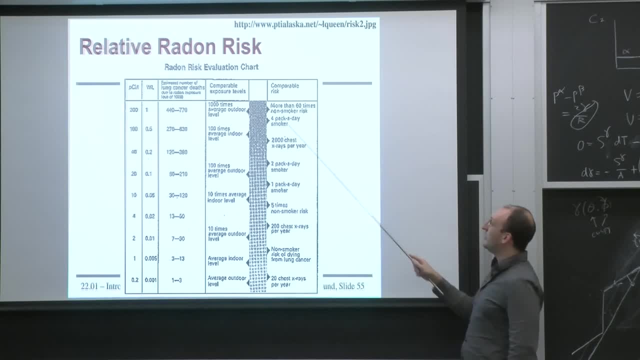 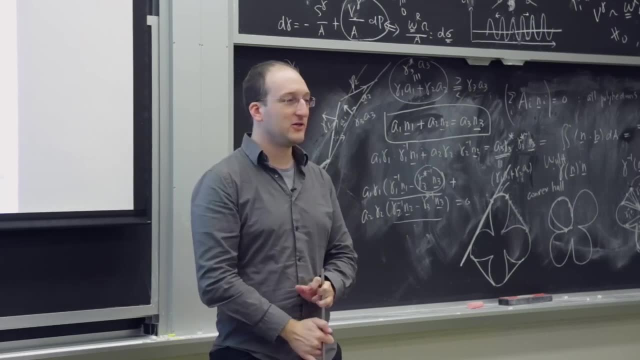 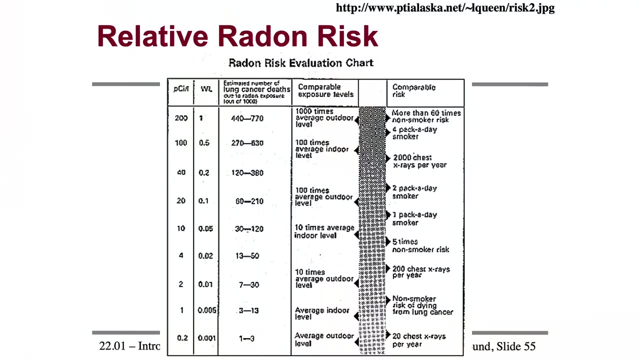 It's like getting 2,000 chest X-rays per year or something like smoking four packs a day. I know some people that do this. They don't tend to be that afraid of the radiation that they're taking in from smoking, But yeah, it's pretty insane how much radiation you get. 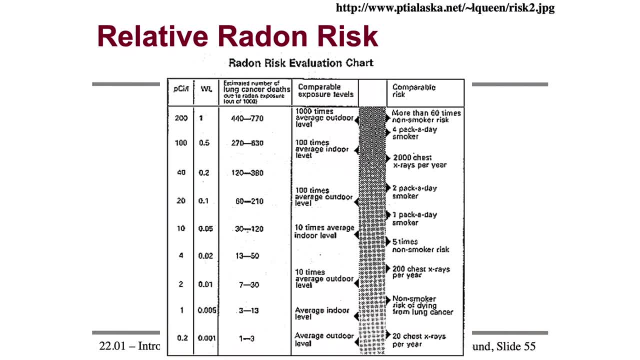 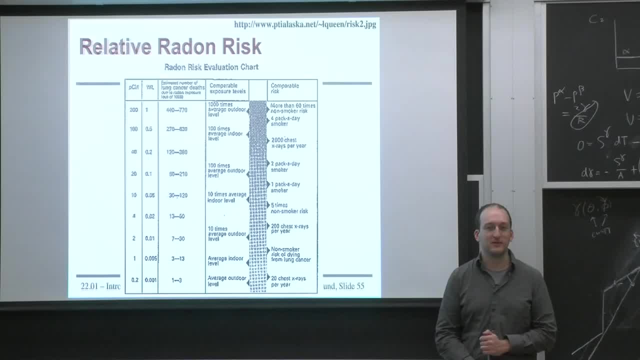 People are afraid to get one chest X-ray, which is not even on this map, right. One chest X-ray worth of radiation gives you much, much less than living for a year in a house, which we all tend to do, Yeah. 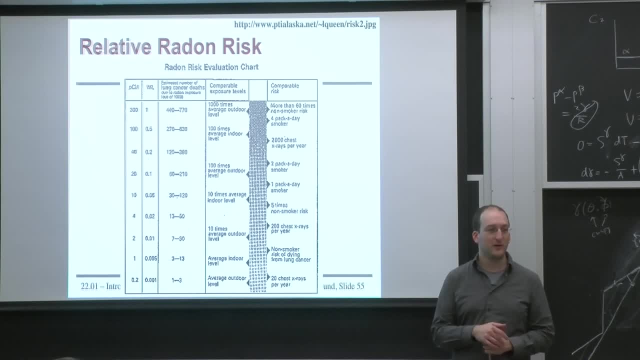 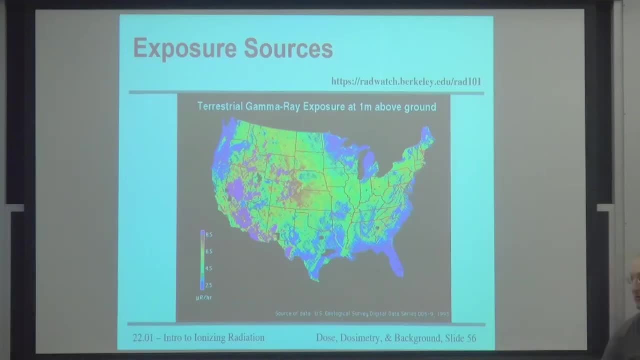 But if you live in a brick or cinder block house, you actually get a fair bit more radiation because these are fairly radioactive building materials And I'll show you those activity levels in just a sec. As far as exposure sources again, 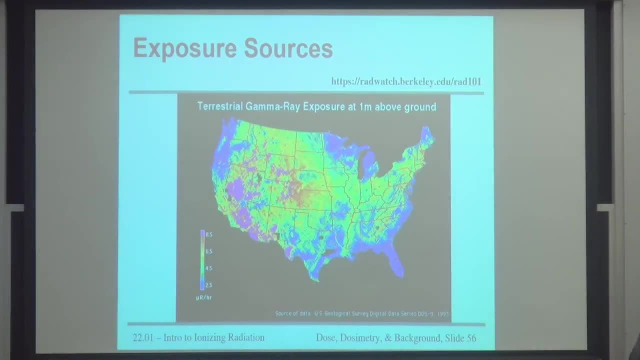 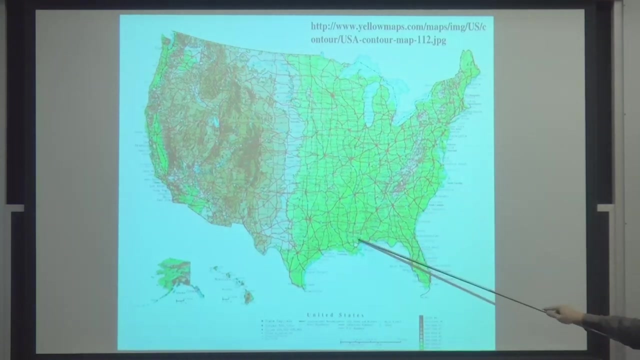 to look at the relative amount of terrestrial gamma ray exposure. you can correlate that pretty well with not green regions on a topological map. So look at the really low levels down here. Correlates with low-lying vegetative areas around here. 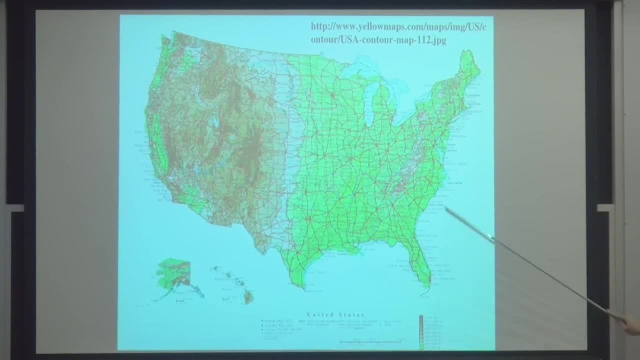 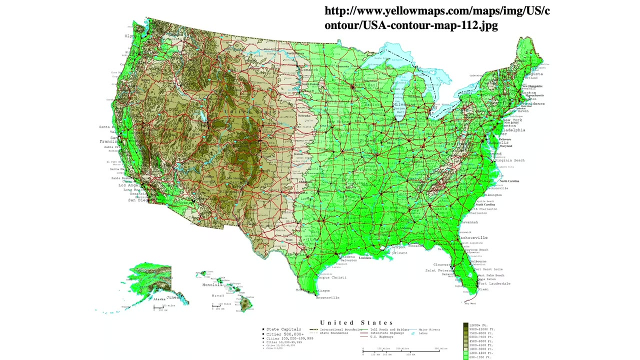 The colors are a little more extreme on my screen But you can see this is all low-lying right here, from Louisiana, Florida, up the East Coast until you get to the Appalachian Mountains and such So pretty striking correlations there. 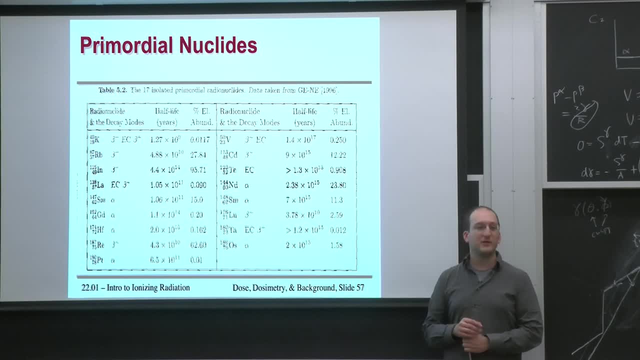 And it all comes from what we call the primordial nuclides. These are unstable nuclides that have such long half-lives that they still exist, despite the universe being 15 billion years old, Or whatever supernova formed our solar system. 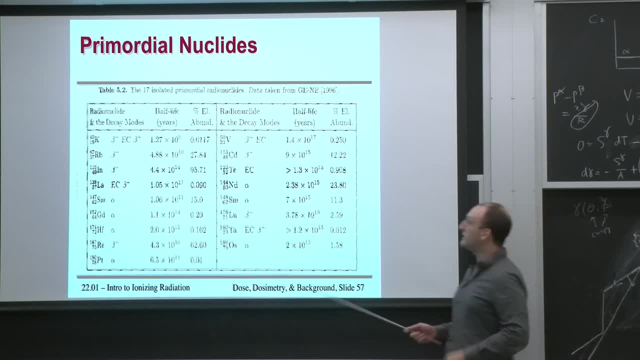 being 5-plus billion years old, Things that we've already studied almost to death, like potassium-40.. And you can see that it's about 0.011% of all potassium is radioactive potassium-40, about 10% of which 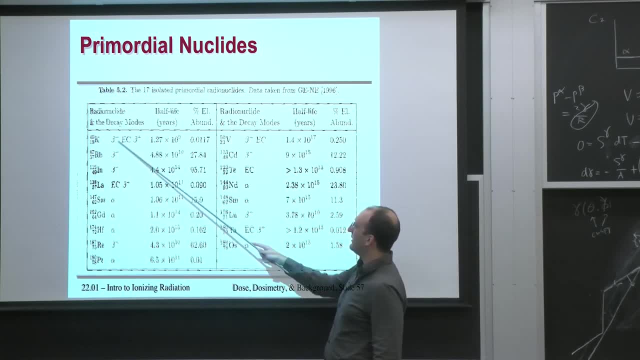 gives off gammas in what is it? 90,, 10?? I forget the split, But can give off either betas and then a gamma, or positrons and then a gamma, Then things like rubidium in the same column. 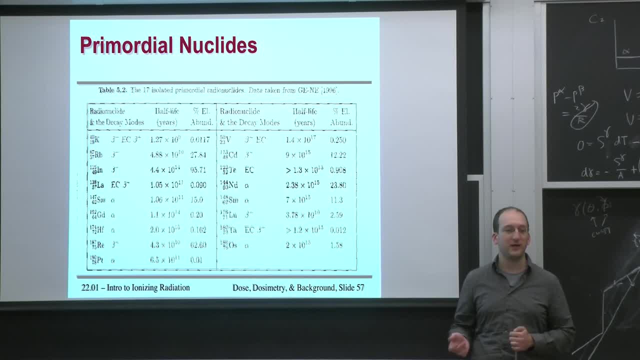 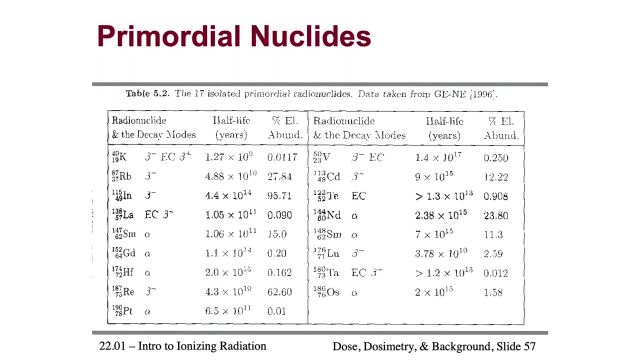 as sodium, potassium And cesium, so it behaves kind of like a salt-like element. There should be some for. are there any for chlorine too? Some of the other important ones to note: oh, platinum- Does anyone have any platinum jewelry? 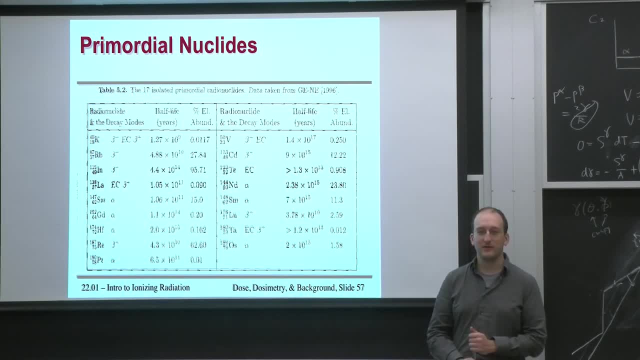 Does anyone have any platinum jewelry? Good answer: yeah, I don't either. I teach at a college, So also I don't like wearing jewelry. Yeah, But there'll be all sorts of these primordial nuclides that you can't really do anything about. 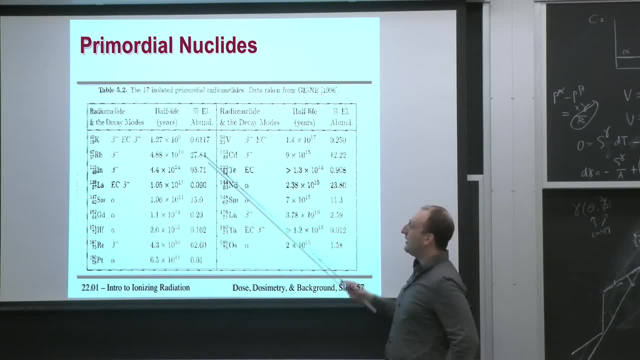 They're just there. Note that the half-lives are really really long And, as you know, now the half-life is going to be inversely proportional to the activity. Despite almost all indium- I mean, look at that- 95% of the indium that you'll find- emits betas. 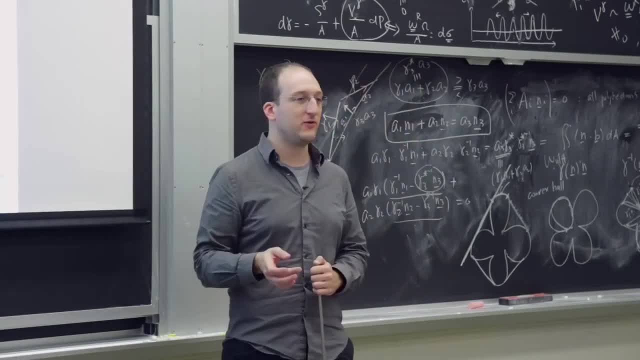 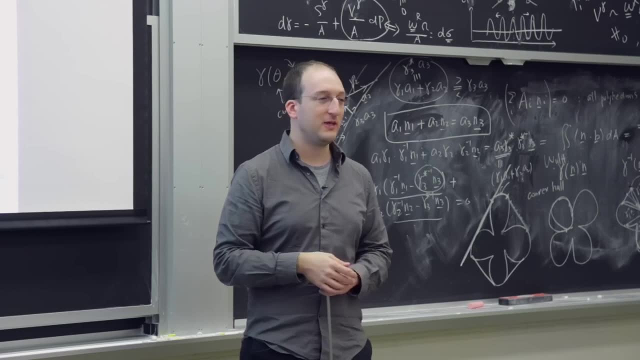 Doesn't stop people from using it as these awesome glass-to-metal seals for vacuum components, Because once in a while it might emit a beta ray, like a whole old gasket might emit a beta once every millennium or so. But these half-lives actually are a measure. 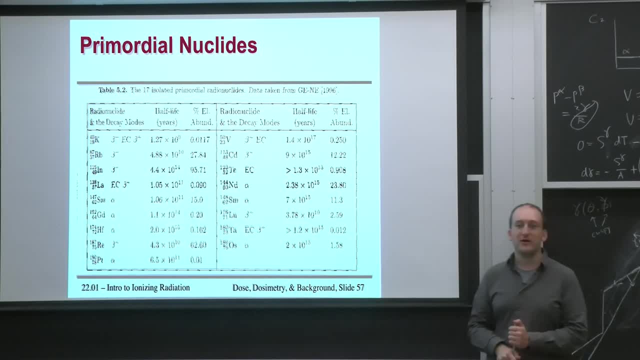 They're measurable, And that kind of begs the question: are there elements with longer half-lives that are just too long to measure? You think of, like, what does it mean to have a half-life of 10 to the 15 years? 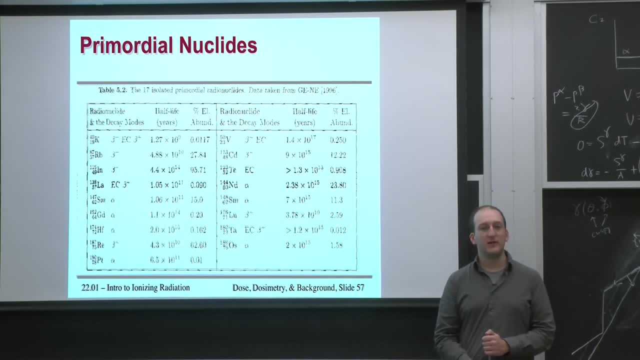 given that the universe is on the order of 10 to the 10 years old right, Is it possible that all nuclei will decay to the end of time? I've seen some documentary such things- and don't call this a science- that say, oh, 10. 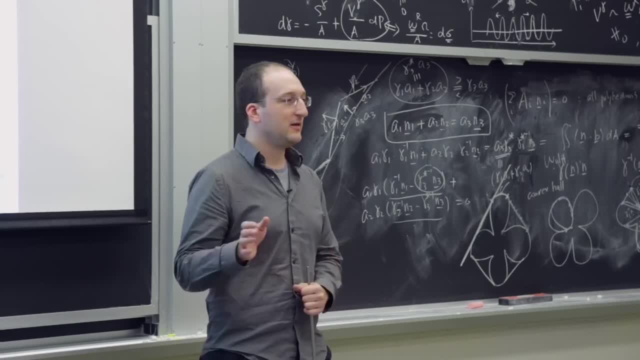 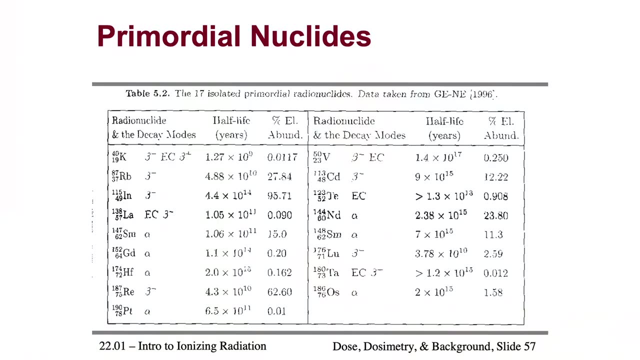 to the 40 years from now, the last protons decay or the last, whatever You know, elements decay into all protons and neutrons, or don't know if that's true, But it does make me wonder. are some of the other so-called stable elements? 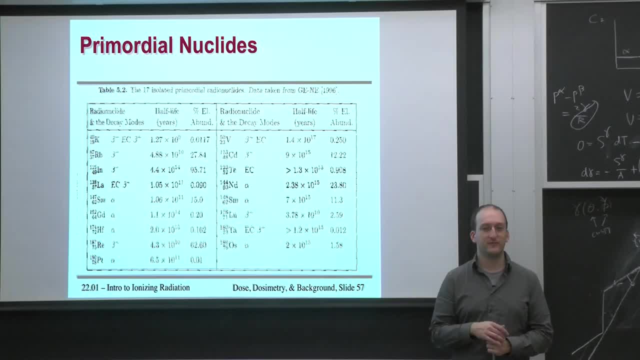 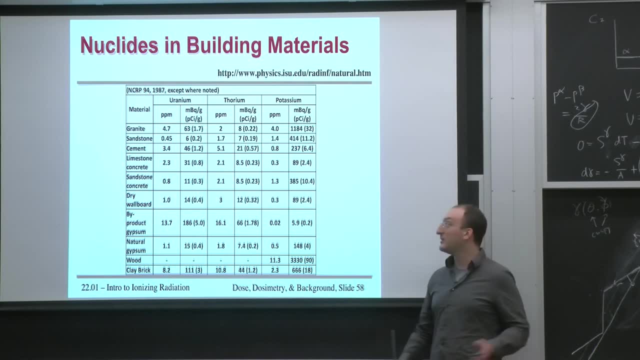 just have ridiculously long half-lives. Something to think about. Let's take a look at the building materials and see what's in well, the typical things around us right now. You can see how much granite, radioactive thorium and potassium are in these building materials. and how many. usually is measured in picocuries per second. Let's take a look at the nanocuries. per gram, A picocurie is already less than a becquerel per gram, because a curie is what? 3.7 or 3 times 10 to the 10 becquerels. 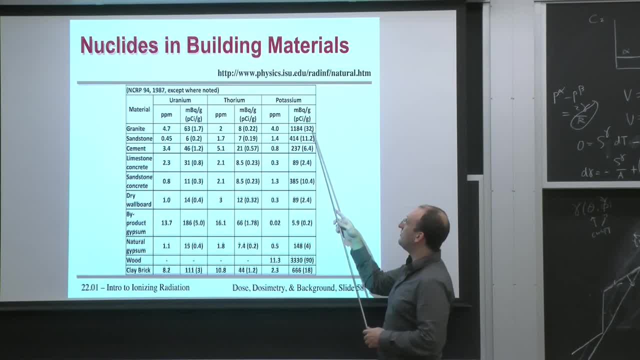 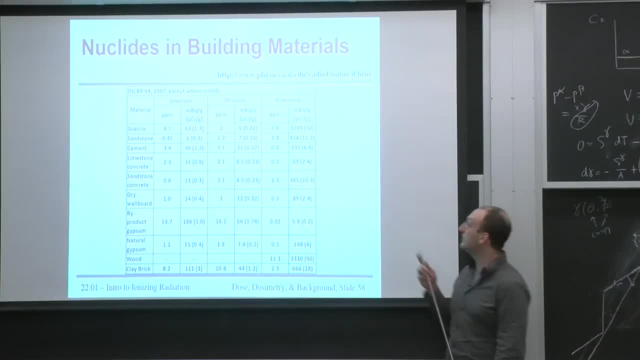 and a pico is a 10 to the minus 12.. So things on the order of a few picocuries per gram. a gram of that material might emit one disintegration per second. not a lot of radiation, But take a look at how much potassium there is in granite. 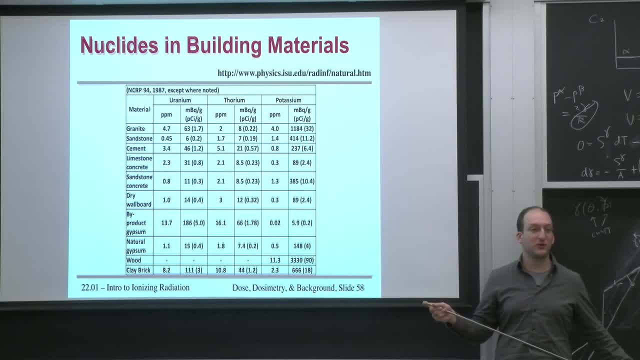 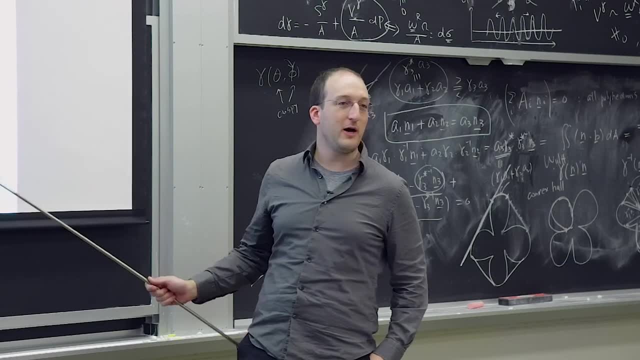 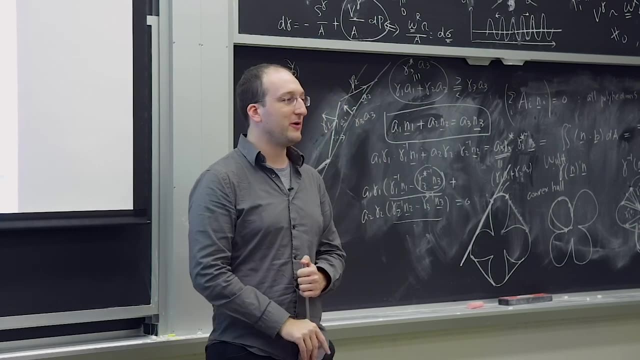 You know nanocuries. per gram, that's a you know integer's worth of becquerels. If you look at wood, check that out. Anyone heard of potash before, One of the ways we get potassium. So if you take wood-based things and you burn them in a fire, 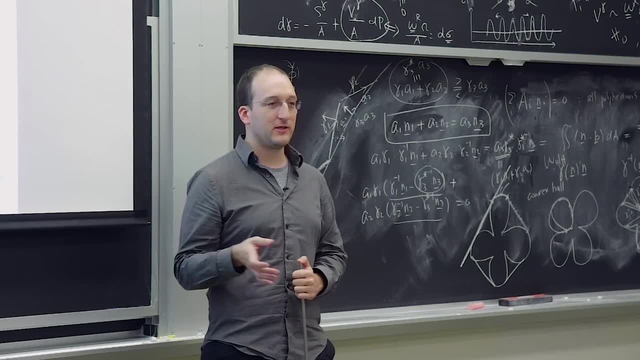 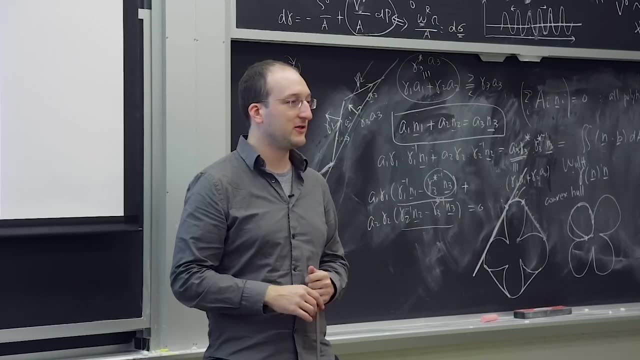 you drive off all the carbon in the water, you're left with these kind of white and like salt and pepper ashes. That's potash. That's the ashes left over in the pot after you burn stuff in a fire. They're quite potassium rich. 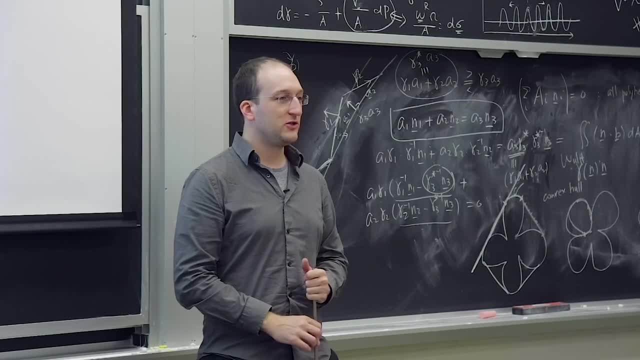 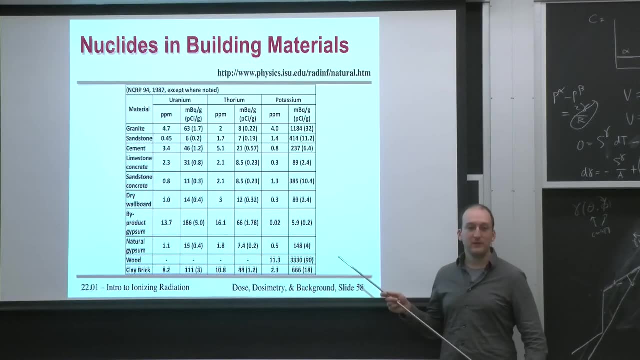 So I think what we'll do next year, instead of burning a bunch of food, is just burn a bunch of wood. Have like a nice bonfire, collect the ashes And we can see how much potassium there is in wood. 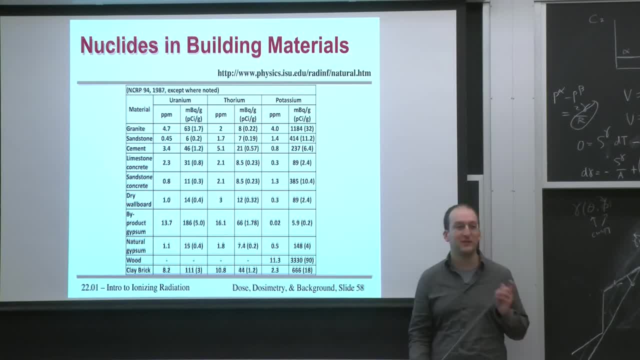 which, pound for pound, if you see on this list, is the most radioactive building material there is Just that. wood happens to be pretty inexpensive and consists mostly of water, lignin and other carboniferous materials. They don't have carbon-14 on this list. 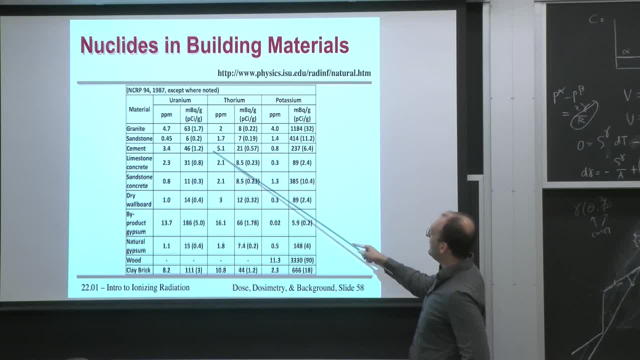 But let's take a look at some of the other ones. So sandstone cement has a pretty toasty signature to it: Gypsum drywall 180,. what is it? 13 parts per million uranium in all the drywall you tend to find. 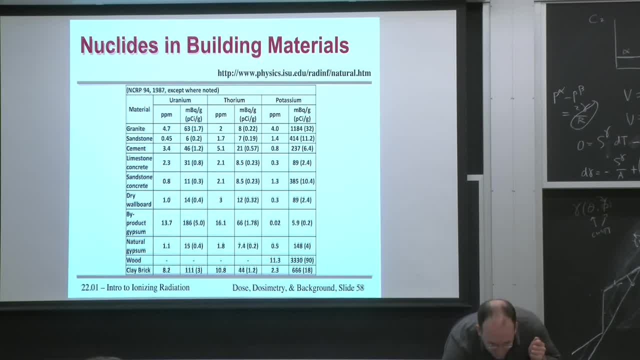 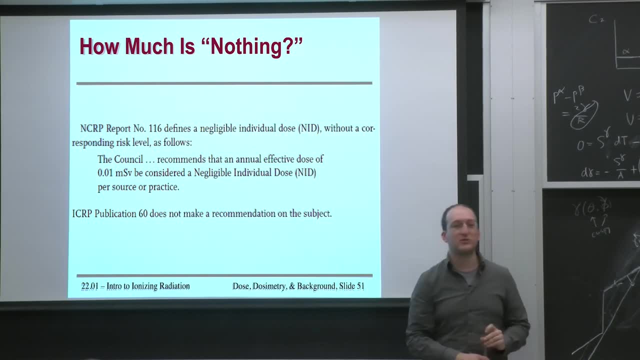 Anyone scared yet, Because you shouldn't be. Like I mentioned before, this is the slide I want to show to most folks in the general public. There is such a dose as nothing And that's pretty much what you get from. let's say: 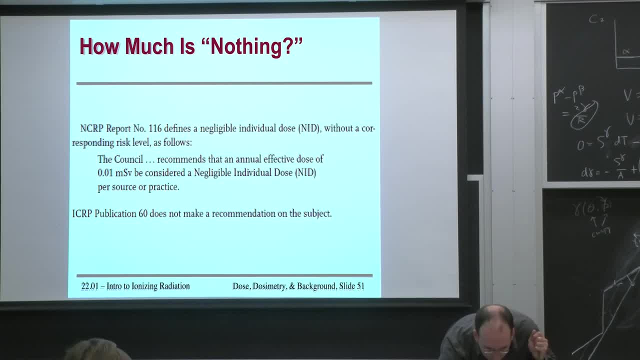 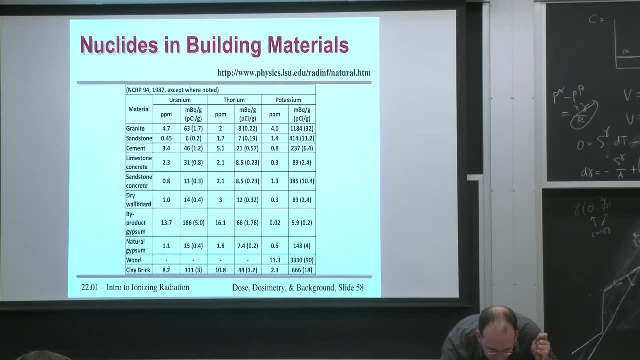 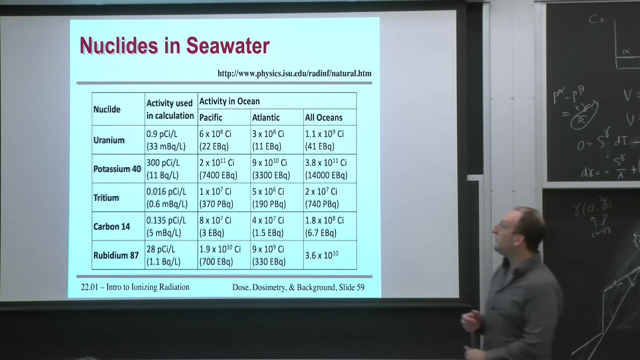 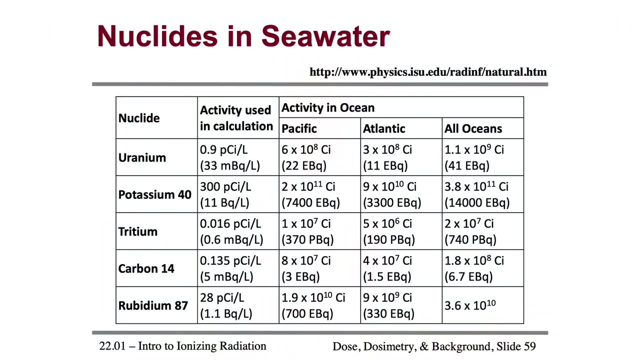 a day's worth of being around these building materials. It's just about nothing. Back to the building materials, There we go. Seawater is another great source of radioactivity, enough so that people have actually proposed harvesting uranium from seawater. 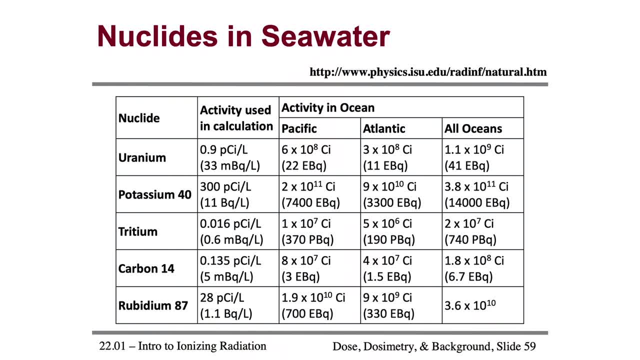 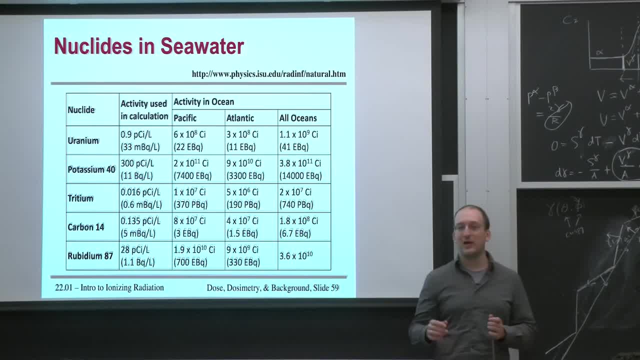 So the total amount of activity in the ocean. there's something like 11 exabecquerels of radiation contained in the uranium in the seawater, which means you should be able to have a gigantic, gigantic trawler flying out around in the ocean. 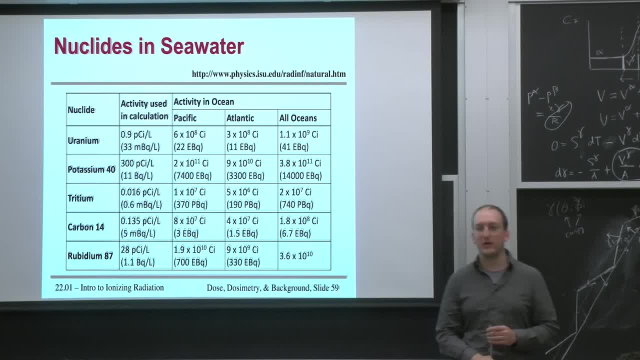 and just floating through the seawater, picking up atoms of uranium here and there, because technically there's enough to power the world for like 2,000 years. The problem is the ocean is big. That doesn't stop people from actually working on it. 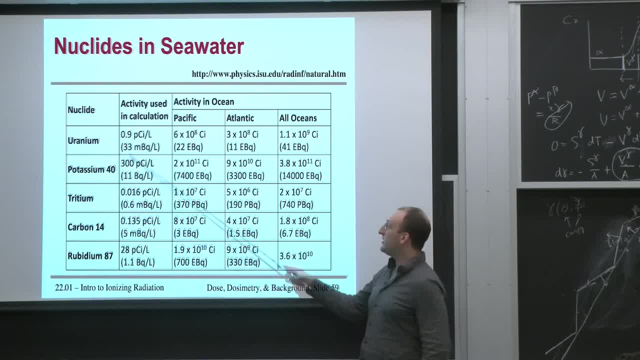 So it's neat to think that there's a whole lot of carbon-14 and tritium and uranium in seawater- 300 picocuries per liter. Anyone have any idea why there's so much more potassium activity than anything else in seawater? 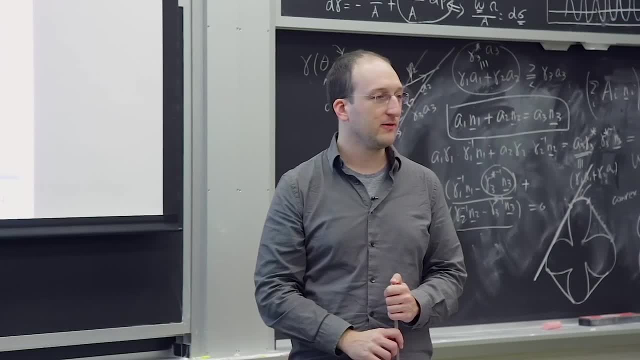 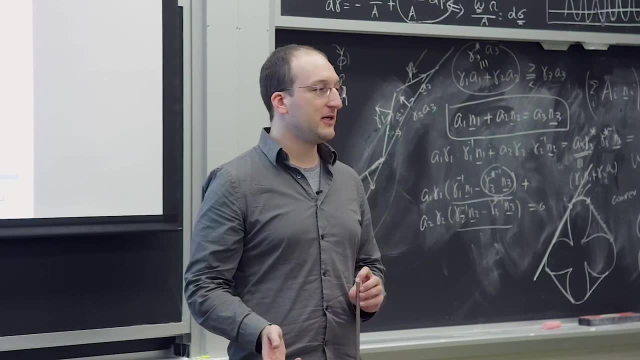 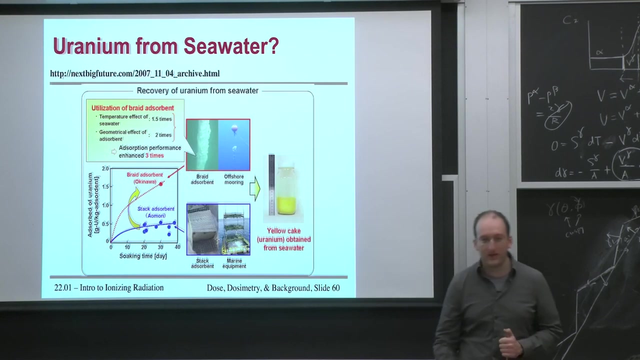 No, Because it's salty. It's because it's salty. yeah, And potassium is just like sodium, So there'll be a fair bit of potassium in the seawater, 0.0117% of which is potassium 40. And so last year people asked what. 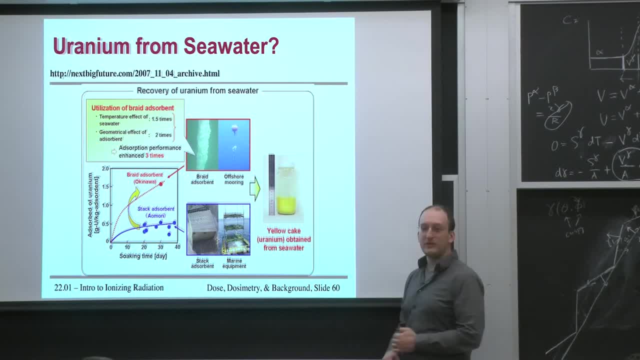 Uranium from seawater. How is that even possible? So this is the part of the course where I'm going to pull out a lot more recent papers to show you some of the cooler innovations going on. So you could use this adsorbent. 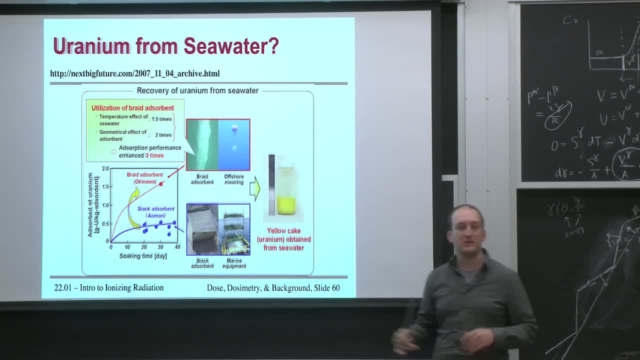 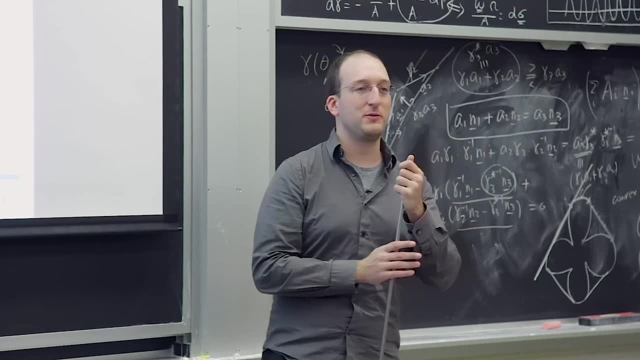 And adsorbent. does anyone know what adsorption means? not absorption: Adsorption is when something sticks to the surface of something. Absorption with a- B is when it actually gets incorporated into the bulk. So folks are thinking about making high surface area. 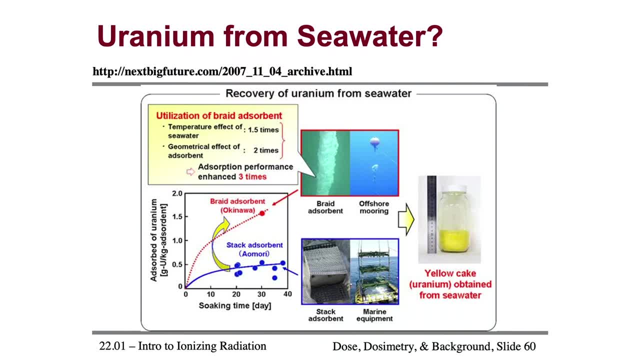 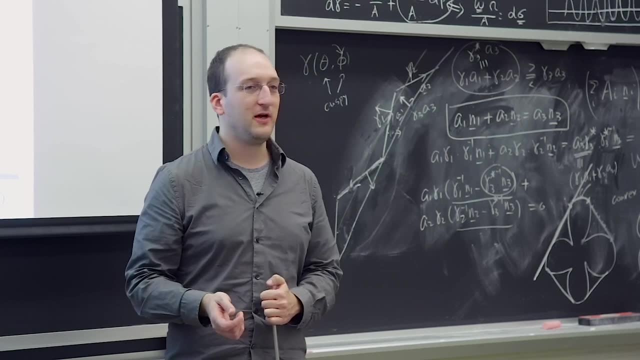 materials that can adsorb selectively atoms of uranium. So you send out this huge braided net or a huge stack of adsorbing material with a D and just go around in the ocean, Attach them to tankers or cargo ships and just have them pull in product. 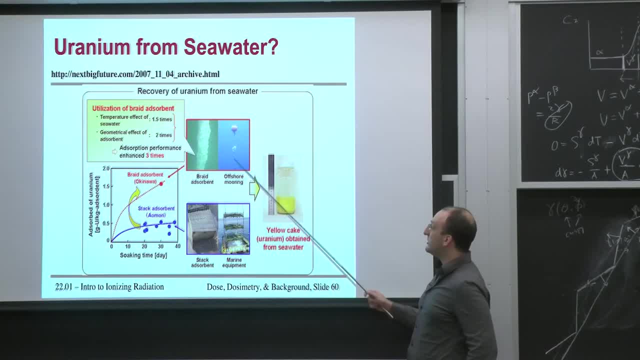 as they go from coast to coast. And by actually changing around the chemistry and the geometry of this, you can enhance things specifically for uranium by about a factor of 3.. And this yellow cake right here, next to an actual ruler, that's 50 millimeters right there. 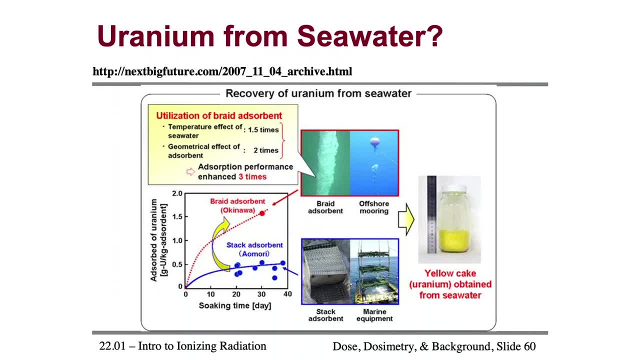 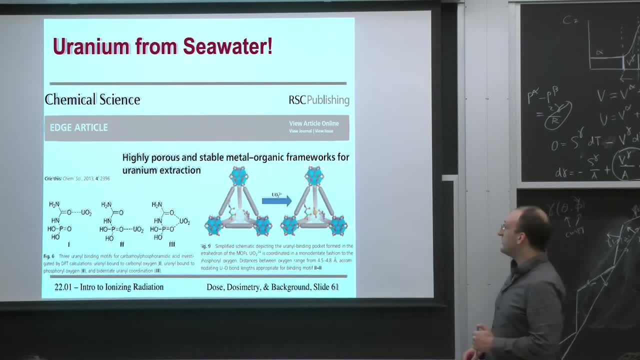 that was obtained directly from seawater, So you can actually pull yellow cake out of the ocean. There's not very much of it, And the way these work is. there are interesting compounds that selectively absorb uranium into their structure, not by direct chemical bonding, but by getting something close. 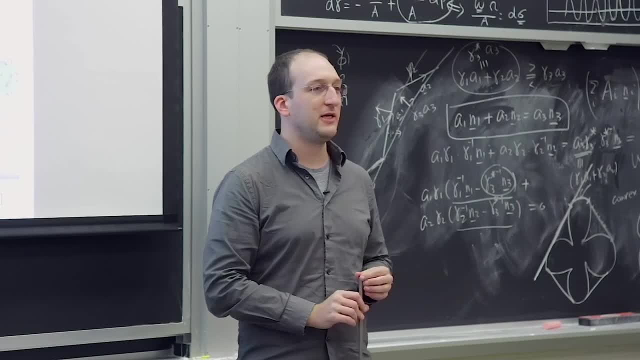 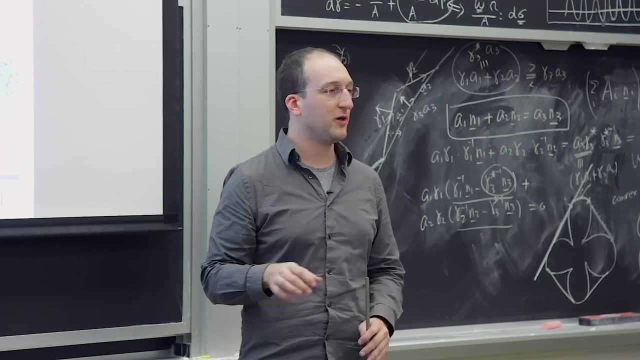 For example, my wife tends to study metals bonding to proteins And it's not necessarily always a full chemical bond, like you might think, but the protein can kind of wrap around a metal ion transport. it places Similar thing going here I'm not going to pontificate. 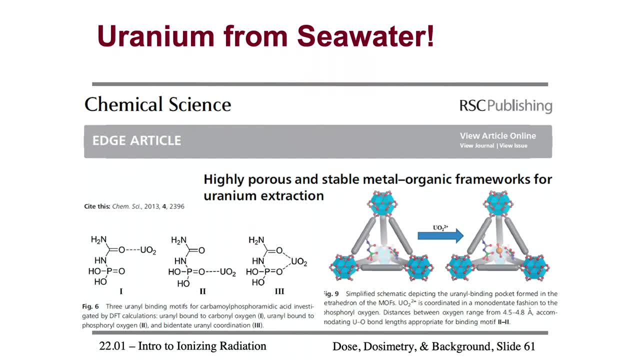 I'm not going to pontificate any more on it, because the title has the word organic in it and I am definitely not an organic chemist. Don't want to tell you anything wrong, But I do want to tell you you can actually. 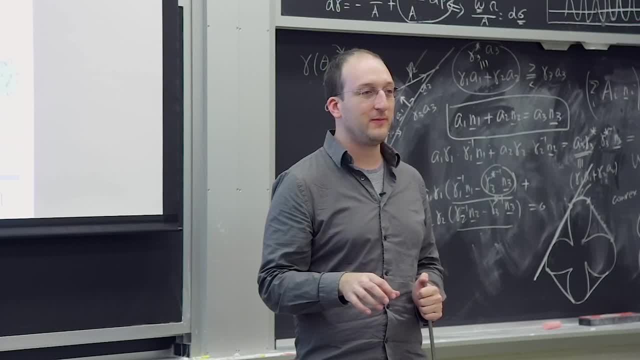 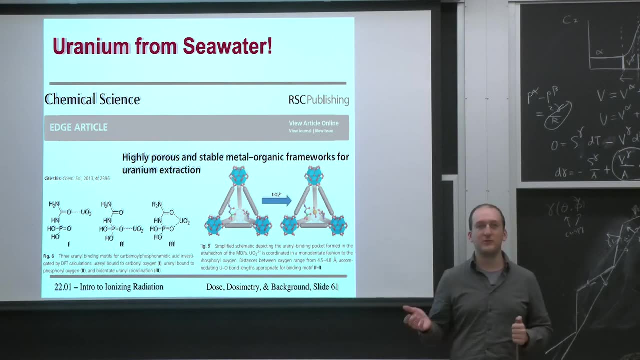 see this paper to find out what sort of compounds selectively grab onto uranium. And if there's a seawater floating through and uranium happens to flow nearby, it can bond to it. You can then somehow squeeze out or burn off that adsorbent. 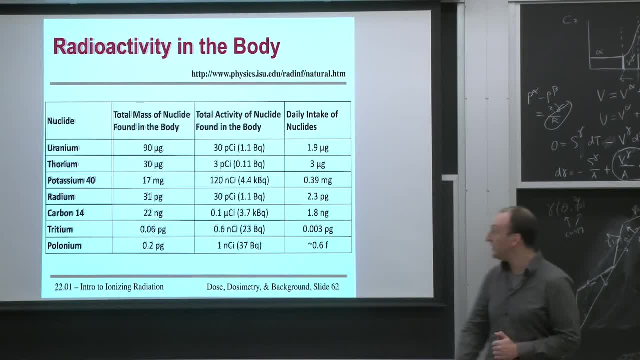 and there you get uranium. Now let's talk about what's in the body and interpreting the spectra that you got from EHS, your full body spectra. If you take a look at how much uranium there is in the body, well, there's some. 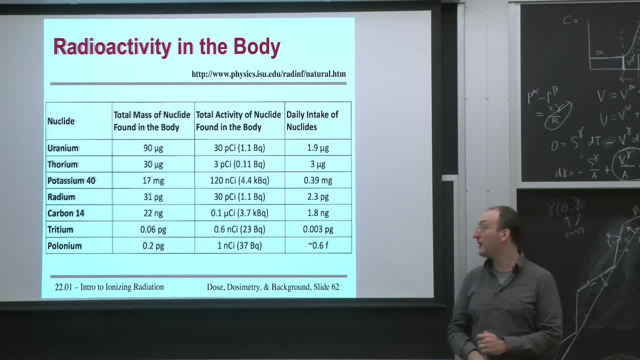 Every one of you has got about a becquerel of uranium in the body, But if you look at the relative amounts- the only things that really matter- a ton potassium 40, about 4.4 kilobecquerels per human. 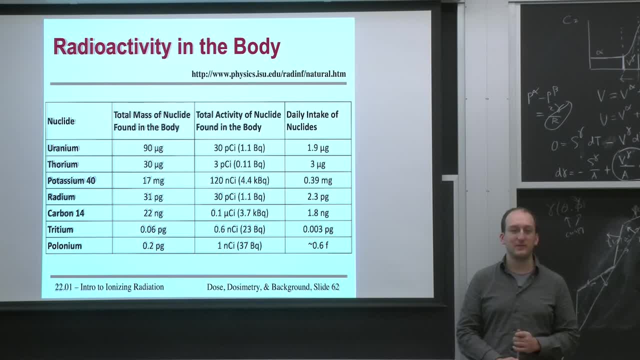 So each of you is giving off 4,400 potassium gammas per second. Most of them just flow right through all the other people. And then carbon 14, about 3.7 kilobecquerels. Pretty interesting to know just how much radioactive stuff. 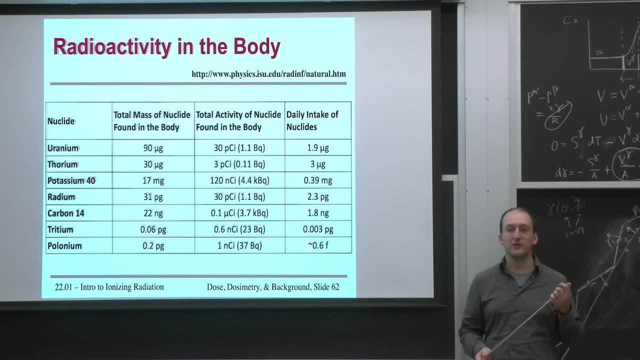 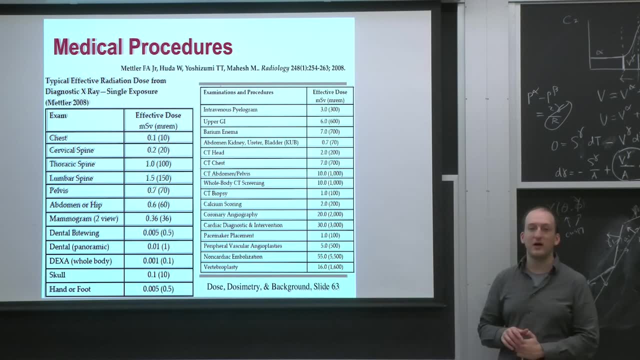 you have in your own body. You will need this table for homework number eight, when I ask you a pretty fun question. Then there's all the various medical procedures, the ones that aren't counted in your annual dose, because they tend to save people. 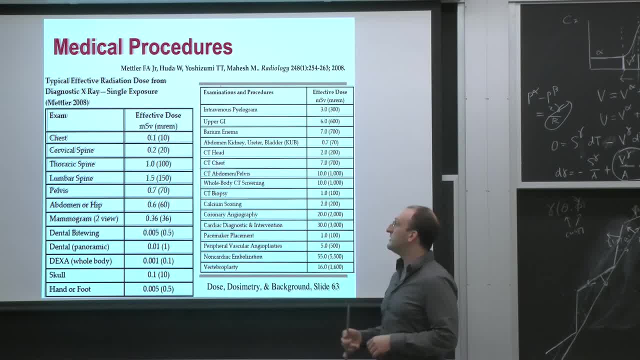 But now let's look at the dose in millirem. So if you want to figure out what this is in sieverts, just divide by 100.. So a regular old chest x-ray- 0.1, let's see how does it go. 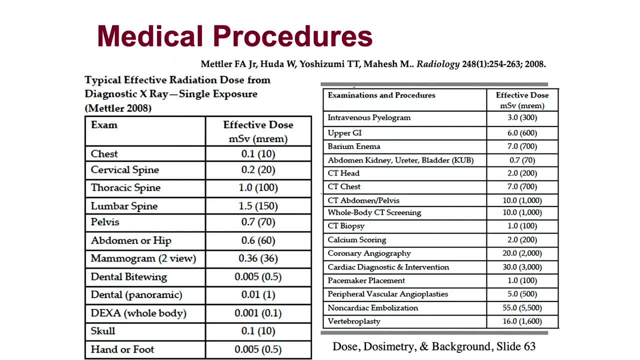 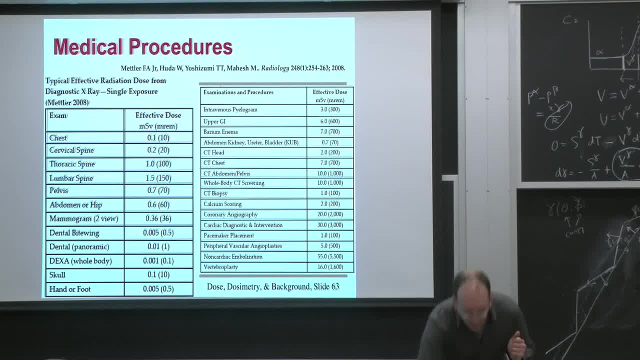 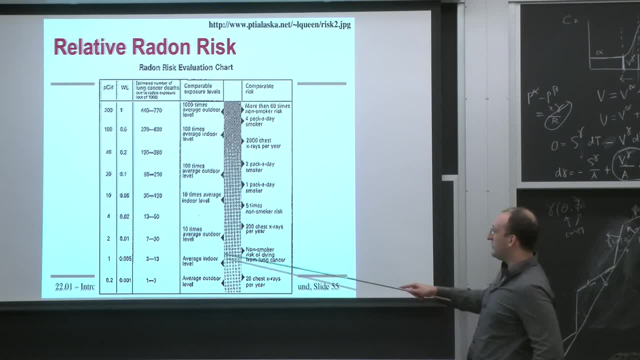 100 rem in a sievert. Yeah, so about 0.1 millisieverts or 1,000 banana equivalent dose, Not terrible. So if we go back to that chart of all those relative risks, if you look at the average indoor level, 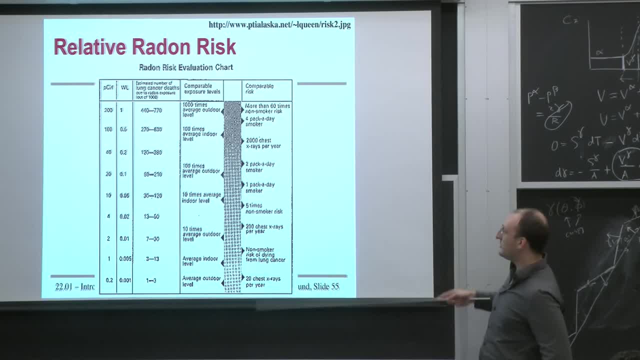 it's like getting- well, I would have to guess- maybe 40 chest x-rays per year. Yeah, Yeah, Yeah, Yeah, Yeah, Yeah, Let's take a look at that. So you're allowed to get around a millisievert or a few. 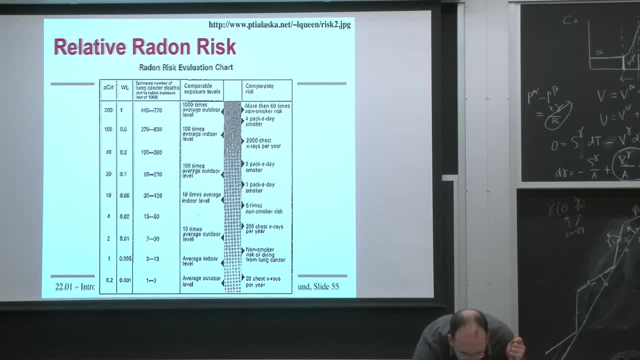 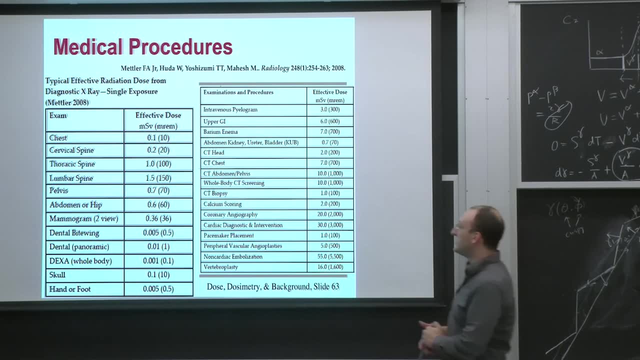 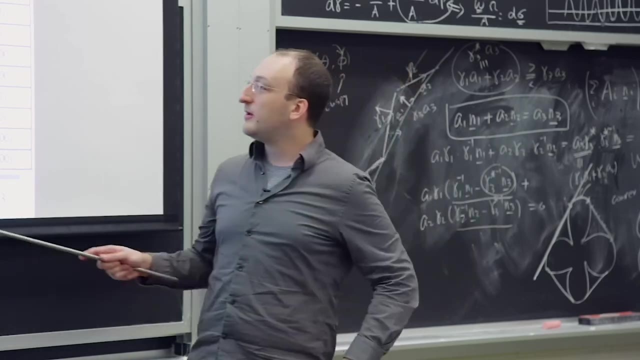 millisieverts of radiation per year. That sounds like it checks out mathematically. Let's look at some of the other crazier ones. Dental bite, wing- Yeah, So anyone ever bite down on something where you have to get an x-ray through the side of your mouth? 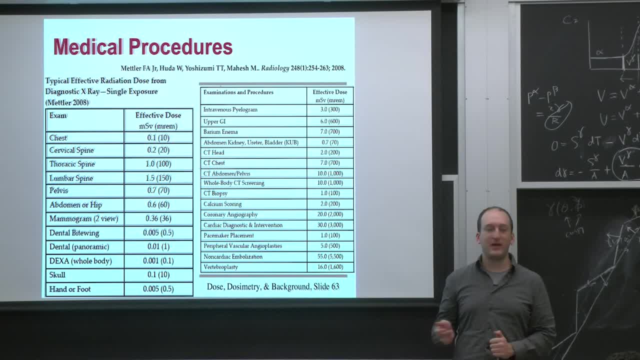 Quite negligible amount of dose, Yet they still put the lead apron on you. I'm guessing that's mostly for show, because that's very, very little dose. It's well beyond the 0.1 micro sieverts of something that counts as nothing. 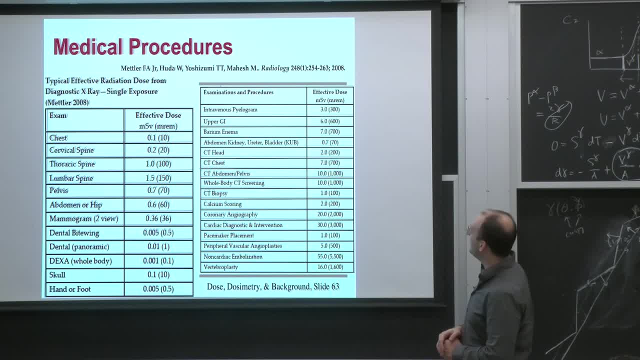 But there's not a lot of dose going into these things. Let's see what really does give you a whole lot of dose: 10 millisieverts for a CT scan or a whole body CT screening, That's a pretty hefty amount of dose. 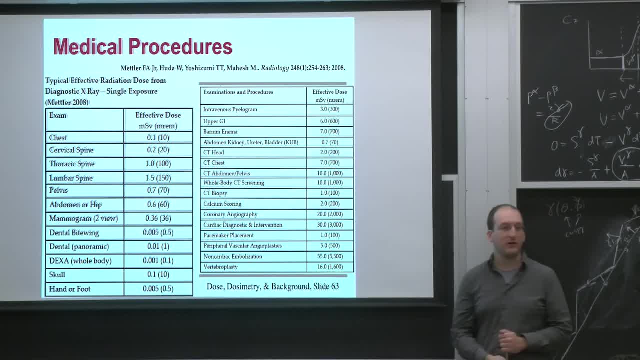 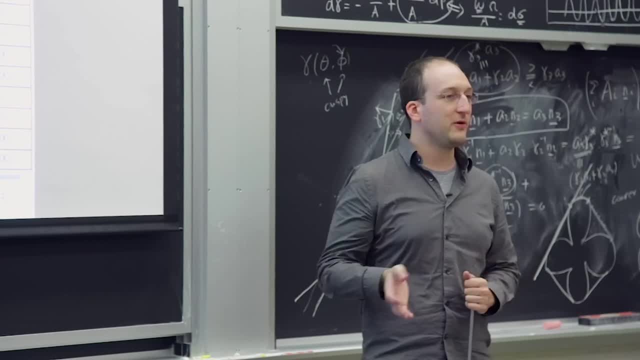 That's right there. with one procedure you may get more than your normal annual background dose, But if you're going in to look for stuff, chances are you need to find whatever you're looking for. So we don't count it And it may give you a slightly higher chance. 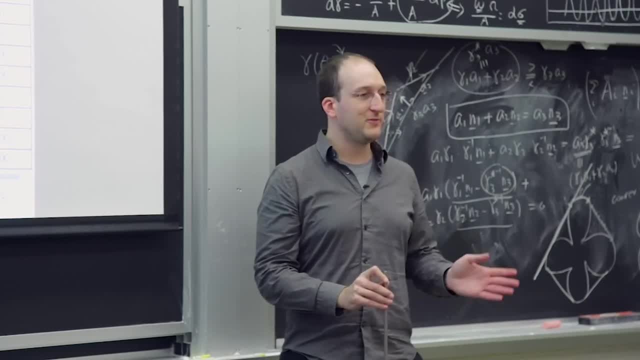 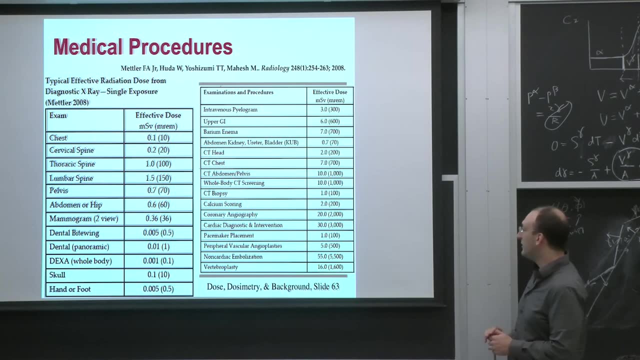 of developing cancer much later down the line when that cell that gets mutated divides. but it's probably going to save your life in the next hour or the next day, So definitely worth it. Let's see the worst. What's the worst procedure we can find? 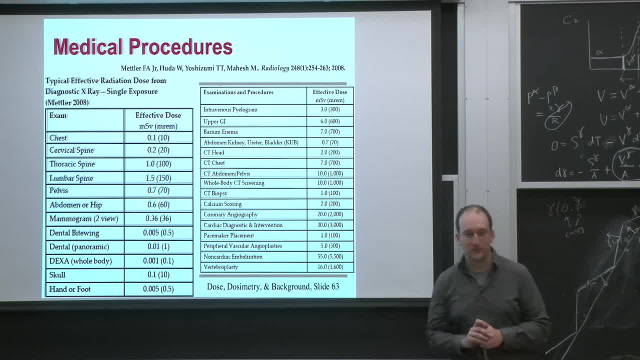 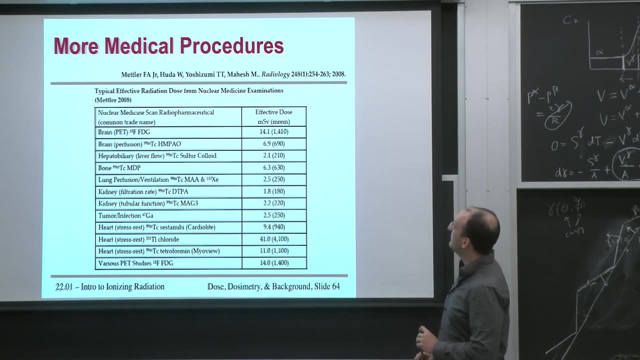 Non-cardiac embolization. I don't know enough biology words to know exactly what that means. Yeah, I think we all know what non-cardiac means. Good, This isn't 7012.. Non-medical procedures Or more medical procedures? I'm sorry. 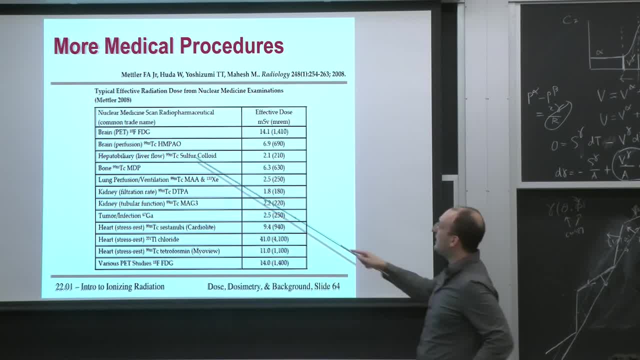 Where's the technetium scan? Yeah, notice how many of these things have technetium imaging, where you'll inject technetium into a certain organ or a certain vascular or lymph or whatever system. Some of these things can give you a fair bit of dose. 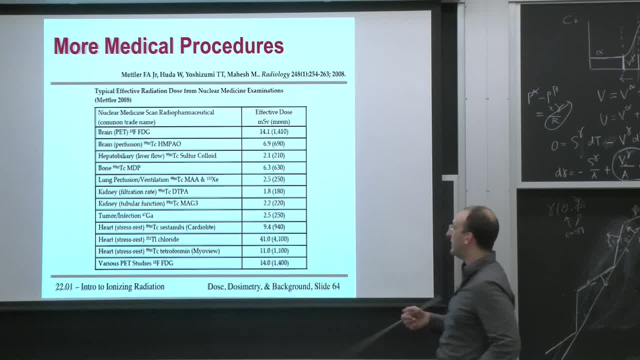 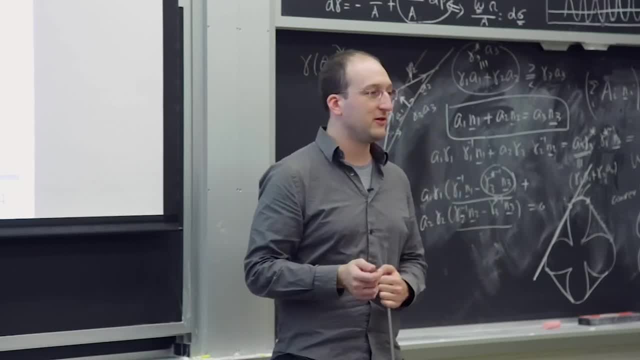 Like again, maybe a heart stress rest test can give you double or triple your normal background dose. This is why you have to declare to airports if you've just had a medical imaging procedure, because this is well more than enough to pick up on any sort of airport radiation monitor. 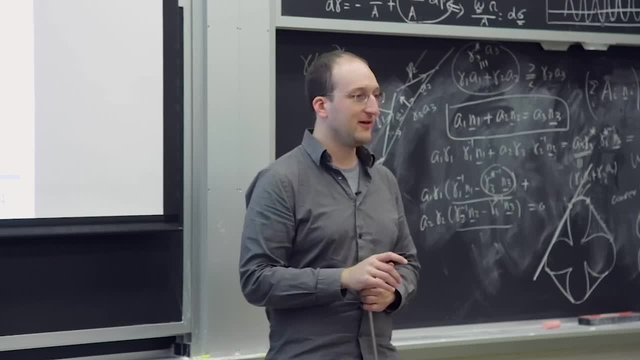 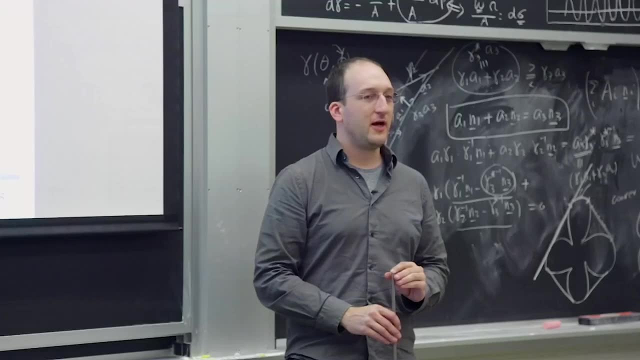 So again, if you ever get a medical procedure with any sort of radiation, anything, do declare it, because it's quite measurable, Yeah. Then there's radiation from altitude. I may have mentioned already that radiation, the reason that pilots can't fly for a certain number of hours. 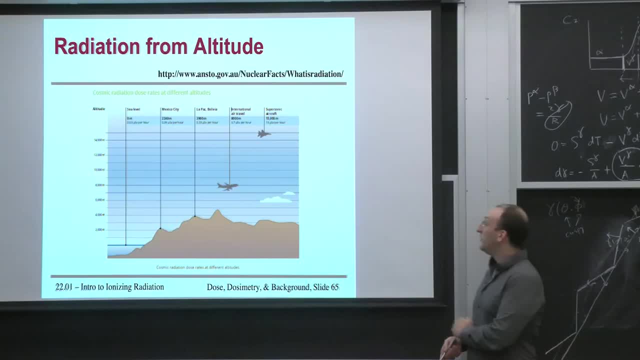 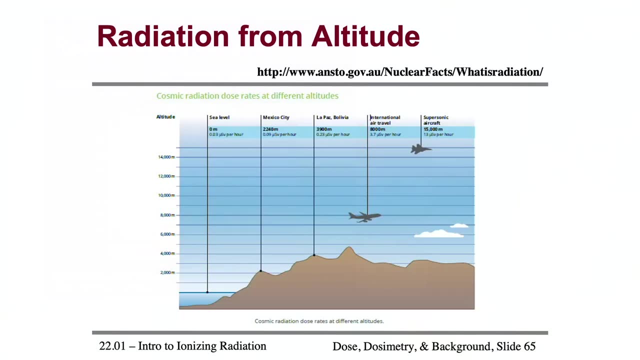 is not fatigue, but it's radiation exposure. When you start to look at how many microsieverts you get per hour on the ground- 0.03.. Right about down at that. hanging around for an hour is a negligible dose. You go up to international air travel. 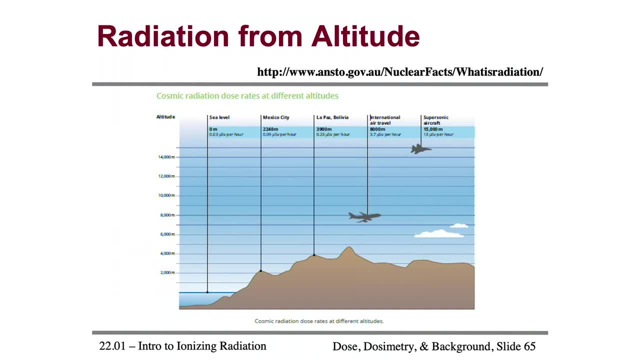 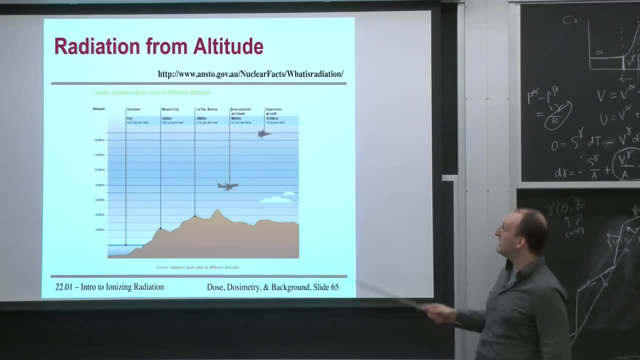 that goes up by a factor of a little more than 100.. And so you get a fair bit of radiation exposure. If you take your annual allowable limit of occupational limit of 50 millisieverts, divide by 3.7 microsieverts, you're. 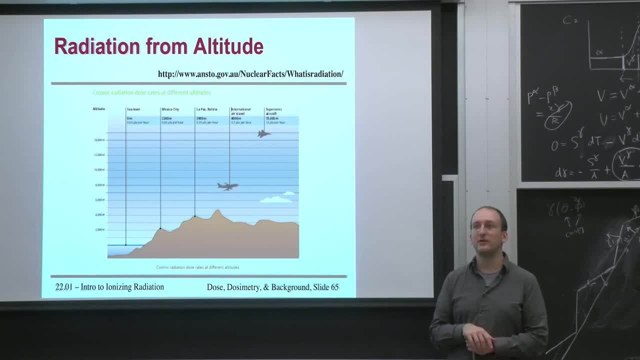 getting close to 86,. what is it? how many hours in a year? Let's see There's 3 times 10 to the 7 seconds in a year. So divide that by 3,600.. That's getting on the realm of 10,000. 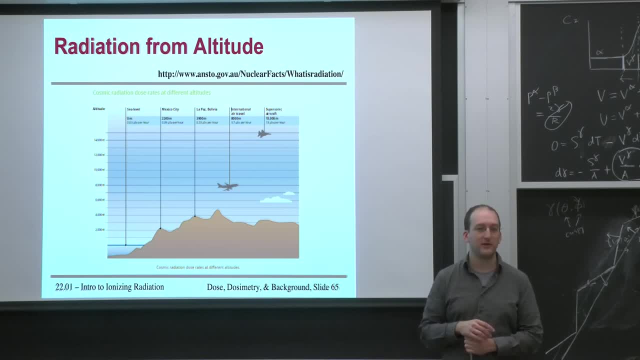 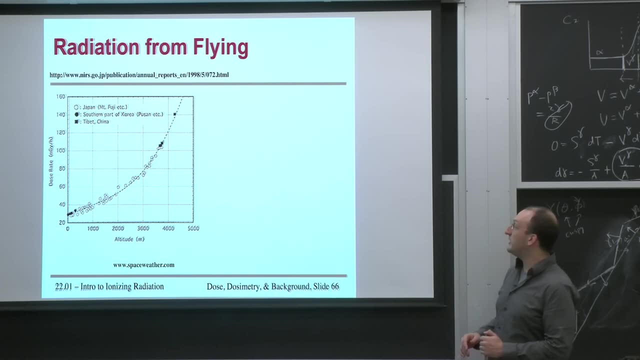 That's about the conversion factor, So you can't spend your life in the air because you'd get too much radiation according to the occupational risks, And so actually, in addition to some interesting measurements that have been published in papers, we've actually had students go out and build. 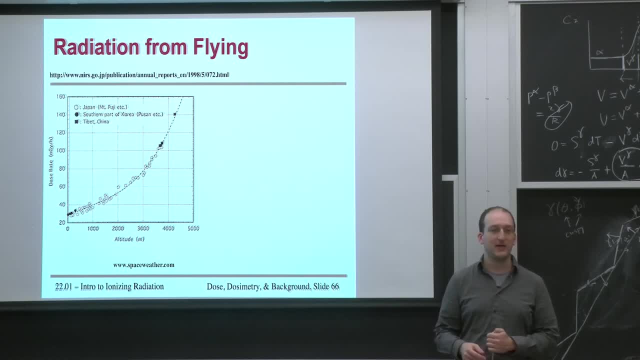 radiation altimeters based on the MIT Geiger counter, removing the speaker, of course, because you don't want a clicking Geiger counter on a plane. That'd be kind of a stressful situation. Let me show you one example of these. These are also published from a paper. 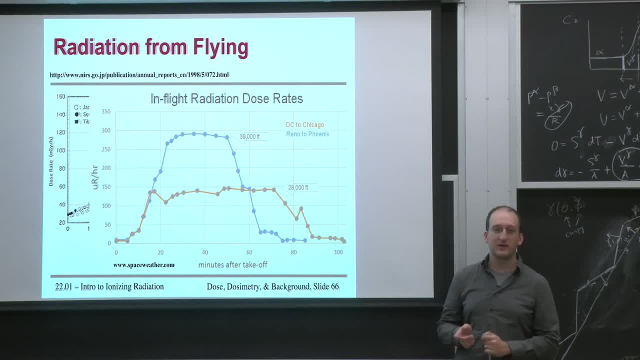 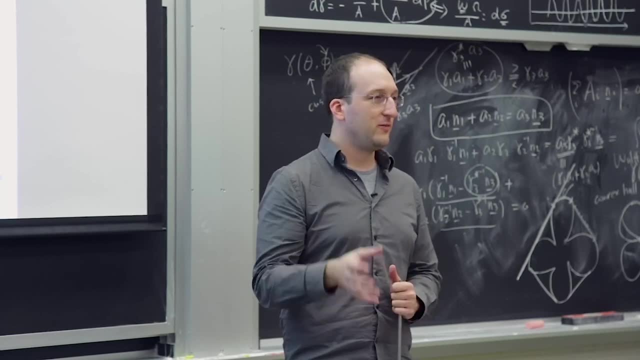 but we have pretty similar data from- if you want, go talk to Max Carlson, one of my graduate students who hooked up his Geiger counter to an alarm clock- the case that had Arduino in it. I think this was a poor choice of case for a plane. 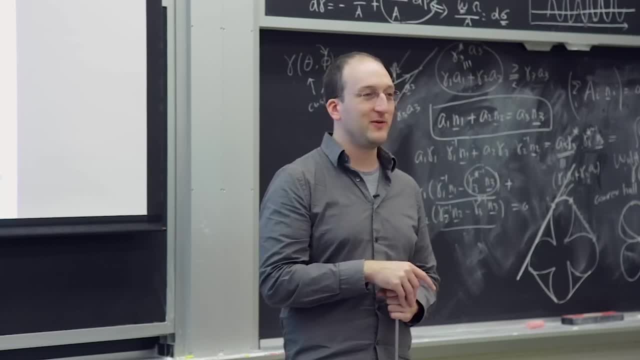 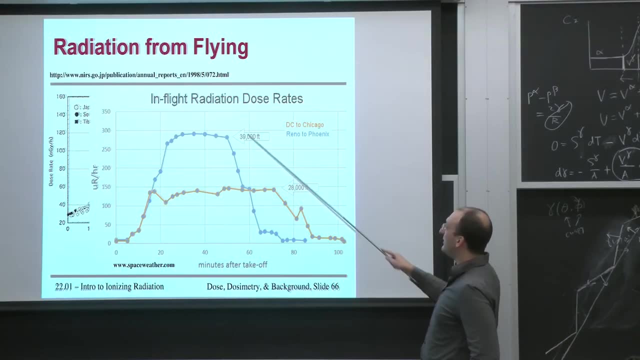 because it looks kind of like a time bomb. But luckily nobody found it and he was able to get the data. Yeah, But you can see just how much more data you get And you can correlate the height that you're at with the dose, in this case micro-Rentgens per hour. 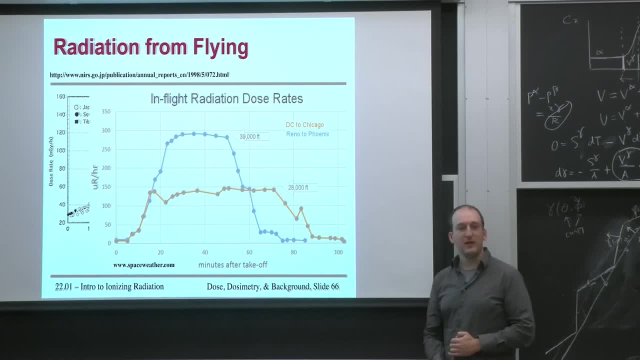 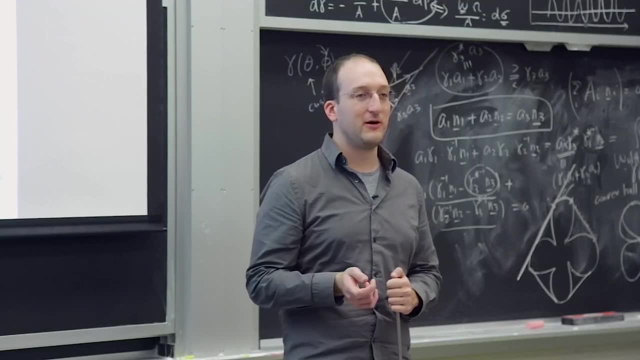 micro-rad. depending on what is it? ambiguous unit definition right there, But it's quite Noticeable. So for those of you who have built Geiger counters and have cell phones and don't want to have a fake time bomb, you can actually hook in your Geiger counter. 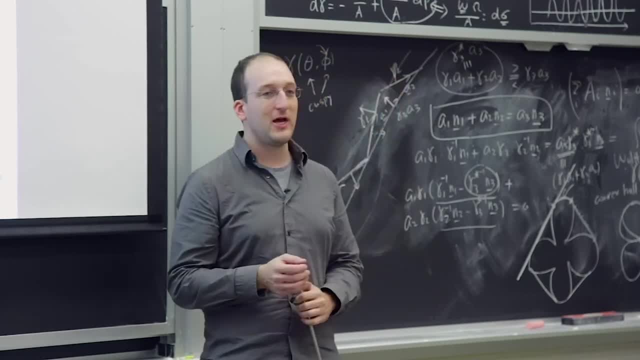 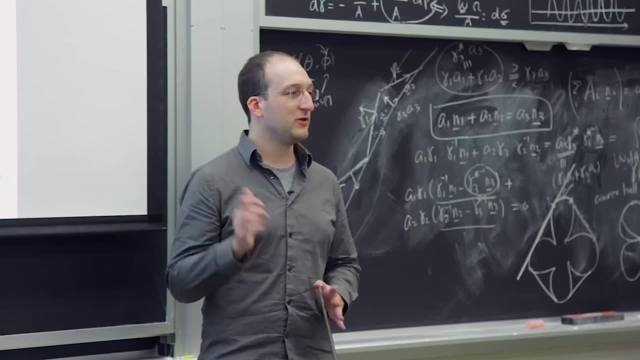 to the microphone port of your cell phone And with a few available radiation apps, you can actually monitor your dose in microsieverts, assuming that it all comes from gamma rays, which is most of what a lot of cosmic rays will produce. So it's a pretty safe approximation. 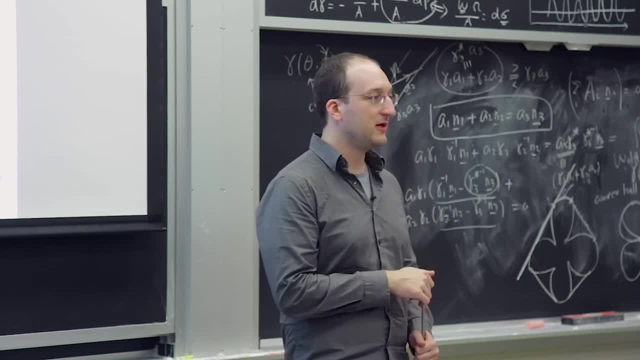 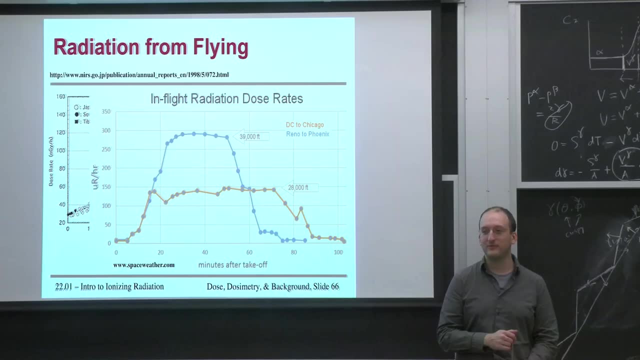 that your dose in gray flying on the plane is also your dose in sieverts, because it's whole body and it's gammas. So I'd say, try this at home, Kids. this is one of those things I recommend you try out. 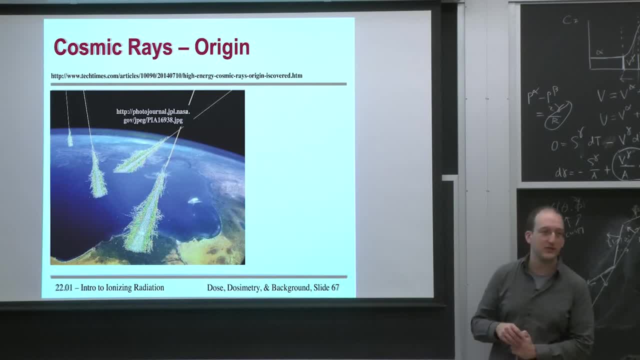 Speaking of these cosmic rays, where did they come from? Well, this is a question that's been under debate and was more completely answered just a few years ago. They come from very high energy particles, from somewhere, It had been argued. do they come mostly from solar flares? 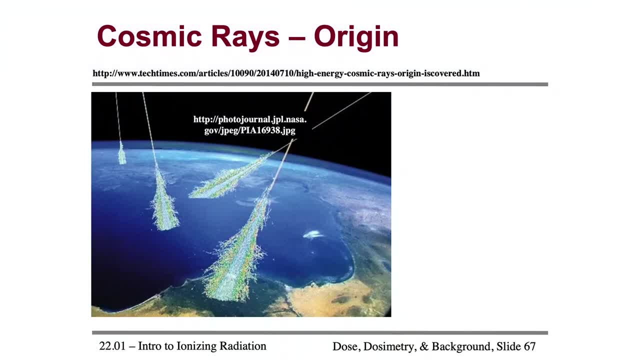 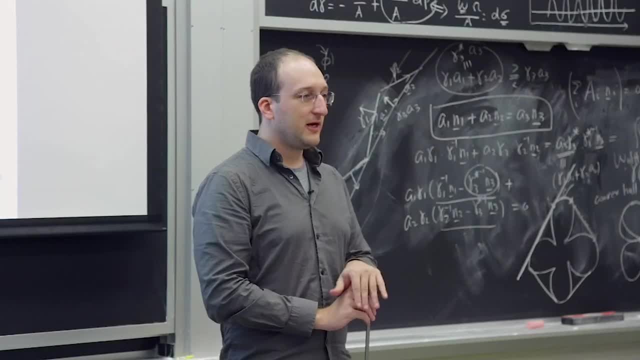 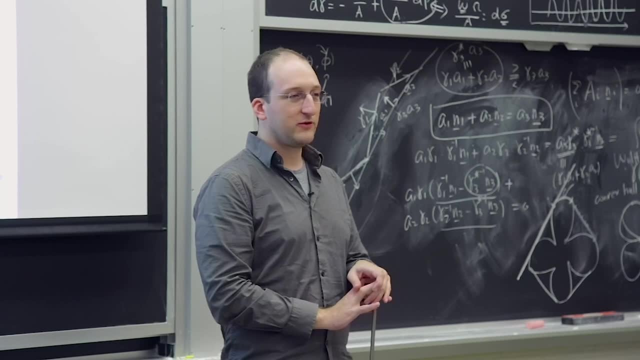 or do they come from elsewhere in the galaxy? Mostly, we're talking about things like high energy protons or other charged particles. We're also talking neutrinos. Anyone know about how many neutrinos are theorized to pass through every second? Trillions, yeah, something like that. 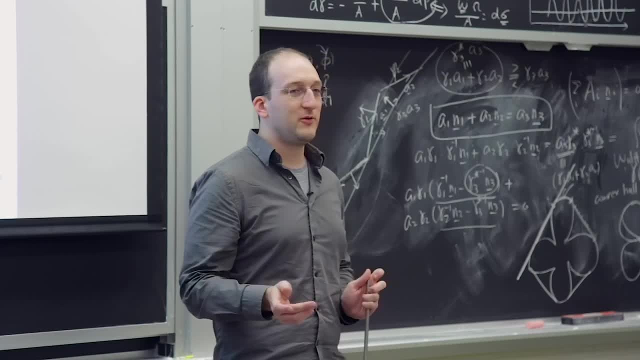 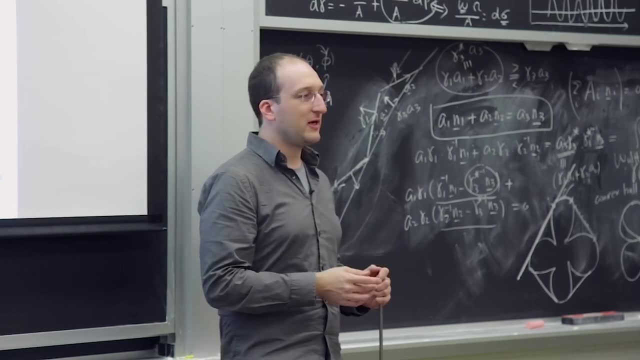 But they basically don't interact with matter. As I showed you guys near the beginning, it takes a gigantic salt mine full of water and exploding photomultiplier tubes in order to catch two or three neutrinos a day, if you're lucky. So let's say those don't really matter in terms of background. 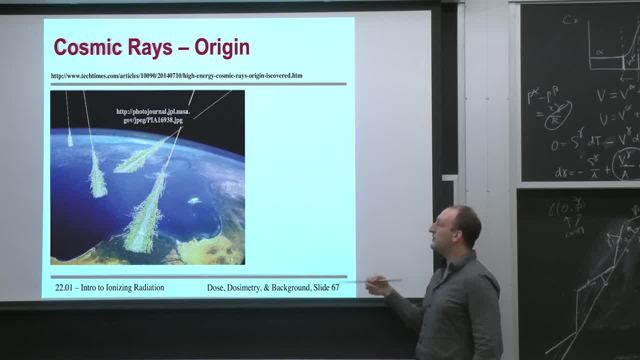 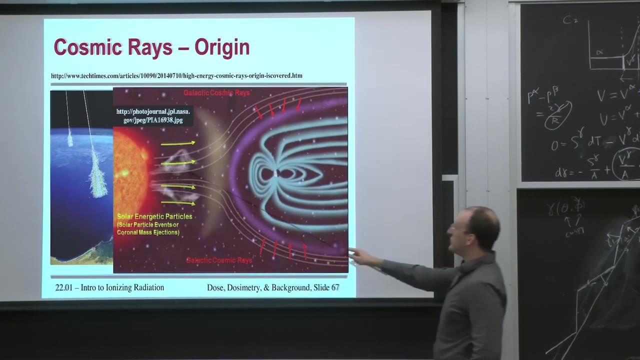 dose. But when those high energy particles interact with the oxygen and nitrogen up here in the atmosphere they produce a shower and cascade of additional ionizations and high energy particles. So it's been said that solar flares and such will accelerate charged particles from the plasma. 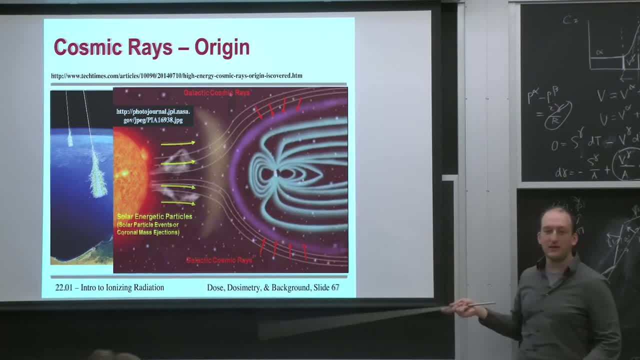 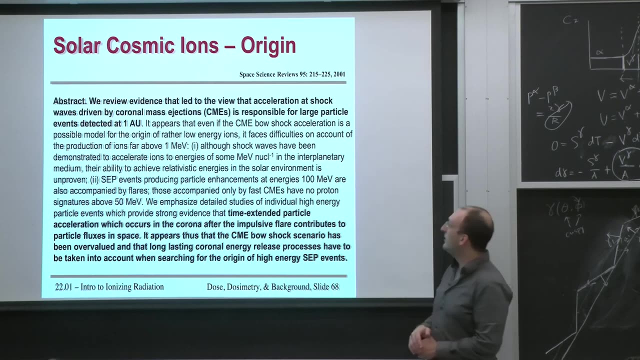 in the sun towards Earth. They're deflected somewhat by the magnetic field of the Earth, but they tend to enter right here at the poles. I'm sorry, that's the simple word I was looking for Until recently in 2001,. they were looking specifically. 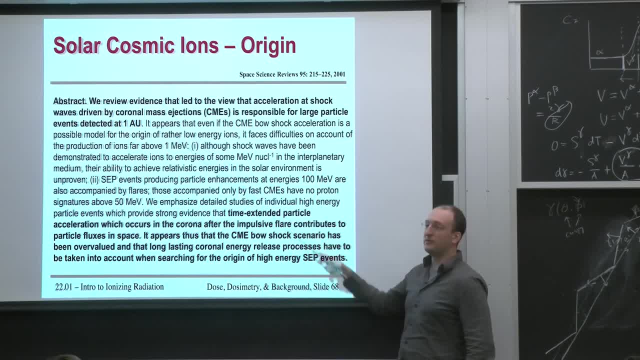 at the evidence for or against the idea that coronal mass ejections, which means large ejections of mass from the outer layers, the sparser layers of the sun, was responsible for most charged particles in cosmic rays. Skipping the stuff that's not in bold. 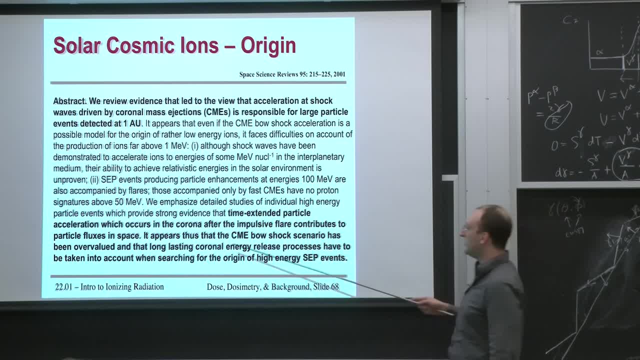 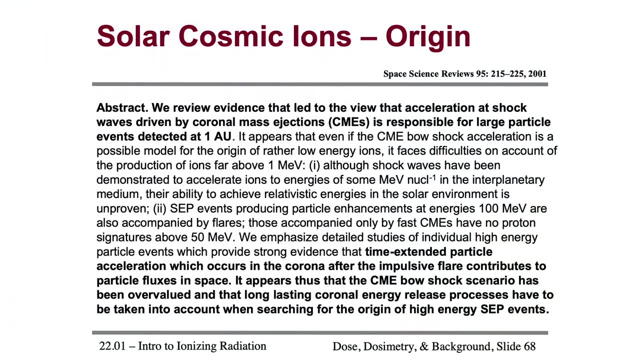 it appears to be that this CME bow shock scenario has been overvalued. So for a while folks were saying: most cosmic rays come from the sun, Most of them are near a star. By making really, really careful measurements of the energy and lifetime of these cosmic rays. 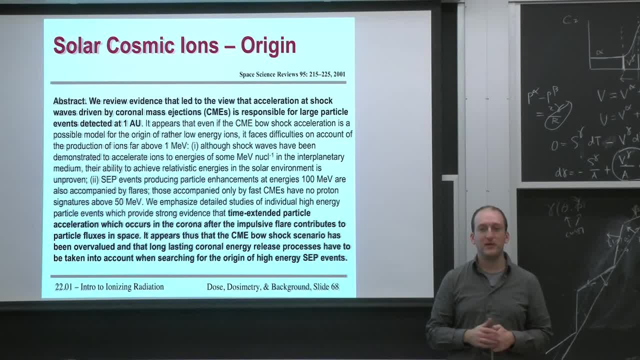 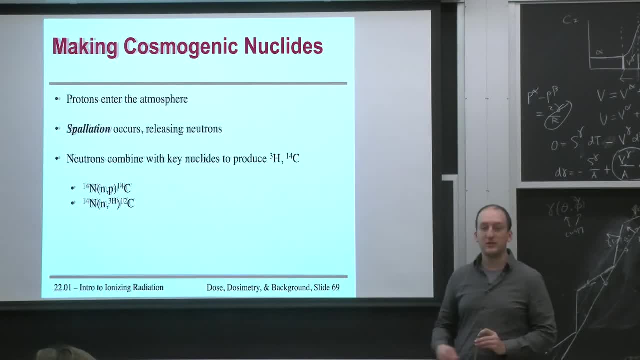 this has actually been somewhat disproven, that this is the major source of cosmic rays, which is pretty cool, But let's talk about where they actually come from, reactions that you can probably understand. So extremely high protons enter the atmosphere. They all start as high energy protons. 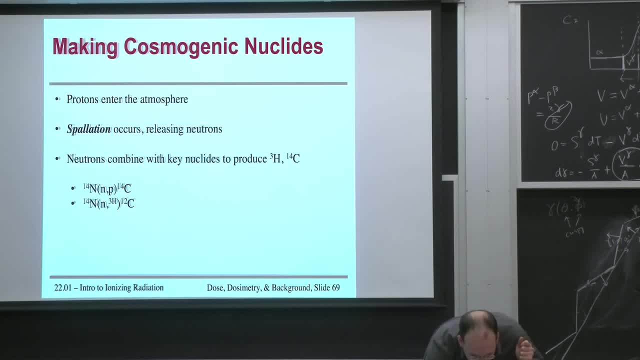 And when protons are high enough energy- and, like I do, probably in every class ever, I'm going to pull up Janice to show you something They can undergo, what's called spallation. It's the same principle that the spallation neutron source. 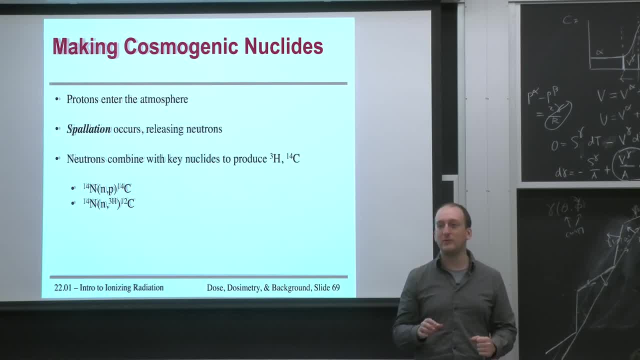 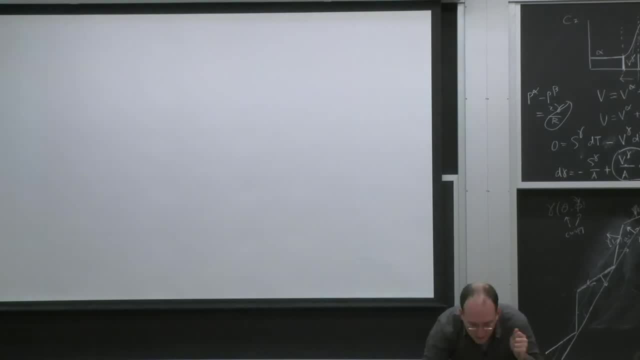 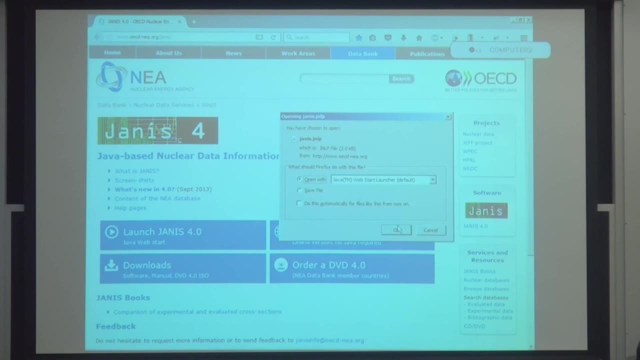 at Oak Ridge National Lab works on is shoot in extremely high energy protons, outcome: neutrons. So usual. it didn't clone the screen right, so just bear with me for a sec. I'd like to, for probably the first time in this course. 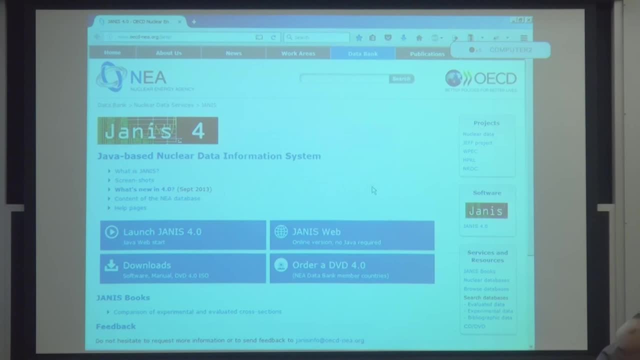 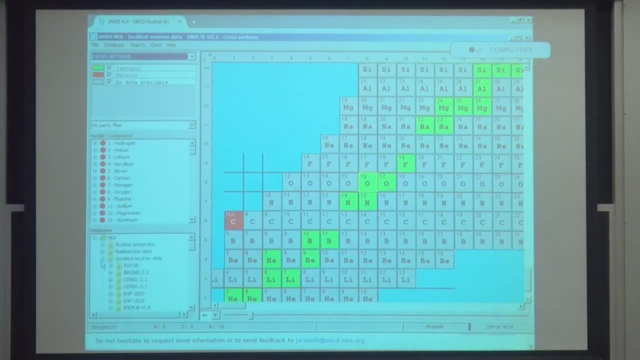 switch databases to the internet. I'm going to go to the incident proton data. Is that actually working? OK, good, So we'll leave the incident neutron data. We'll go to the incident proton data. I think we'll stick with the same library. 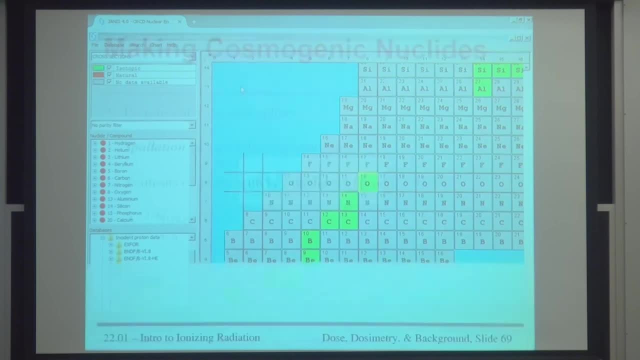 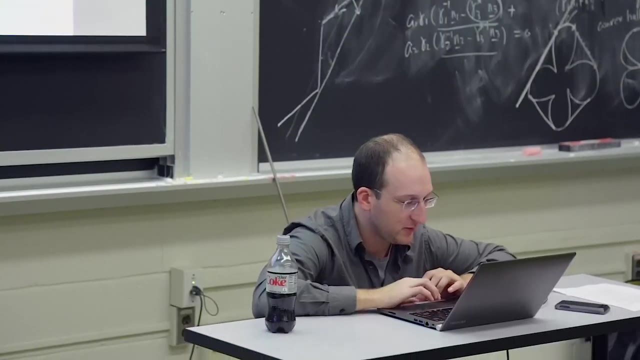 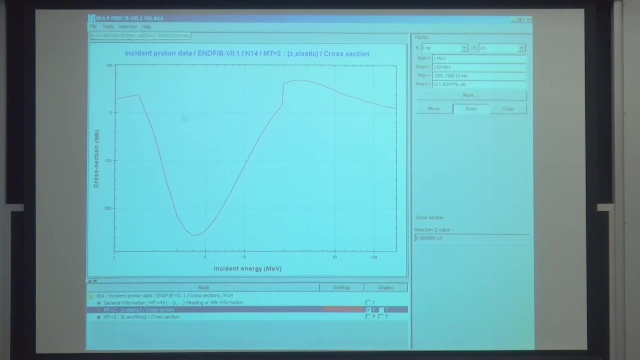 Let's see how much they have. Not much, but enough to matter because there's a lot of nitrogen-14 up in the air. Let's see what happens when protons hit nitrogen-14.. All the way at high energy. so I don't quite. 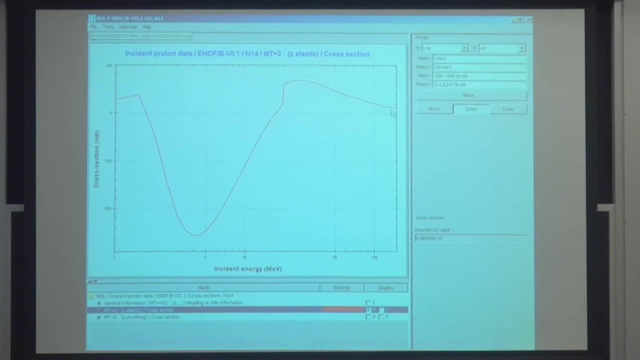 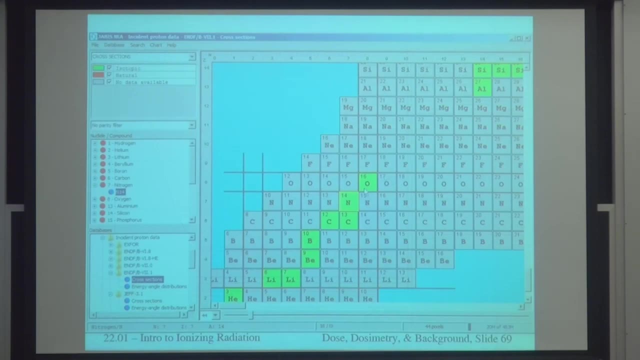 know what a negative cross-section refers to, But at high energies this is definitely a possible event. And let's see, there's not a lot of cross-sections to look at here. Let's try oxygen-16.. Not much. OK, we'll stick to the slides then. 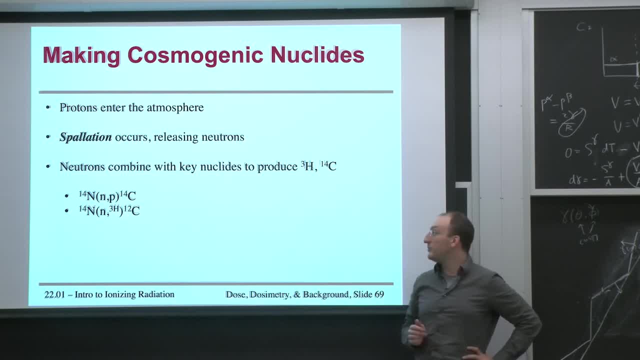 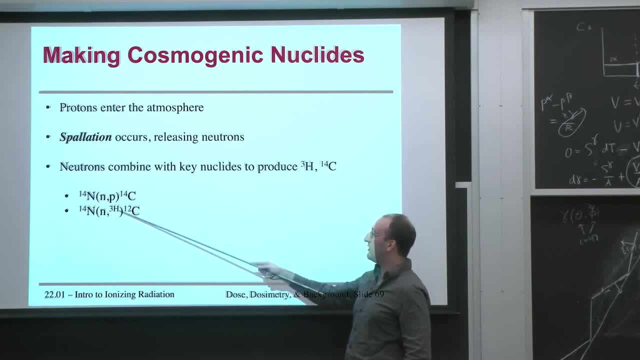 and those neutrons can then cause activation reactions and then emit things like proton or tritium, leading to that's where your carbon-14 comes from: Comes from nitrogen-14.. So in comes a high energy. proton releases a neutron. 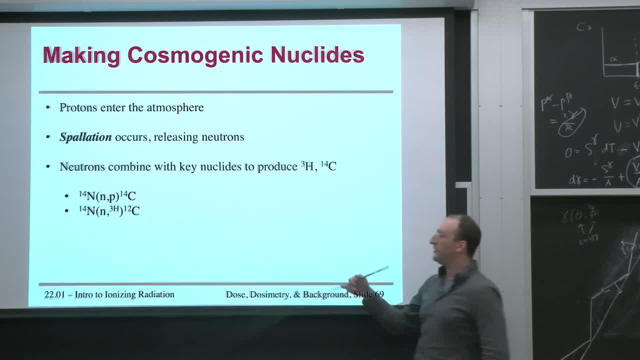 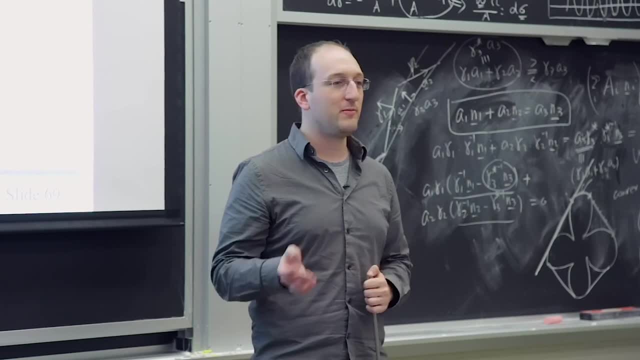 That neutron hits nitrogen-14, releases a proton. out comes carbon-14. So this is why it's being constantly generated in the atmosphere. It's not like there's a certain amount that was there at the beginning of the universe and decays because its half-life is only 5,700 years. 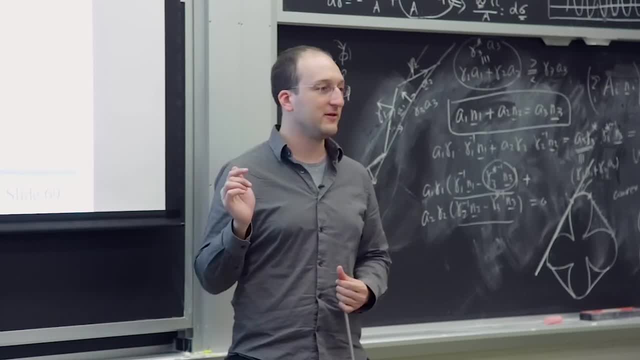 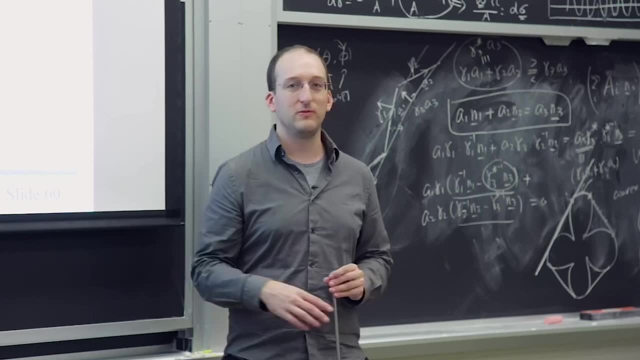 This is part of why radiocarbon dating works, because we have cosmic rays. It's kind of a neat connection to make. If there weren't cosmic rays, all the carbon-14 would decay pretty quickly in the universe time scale and we wouldn't have this form of radiocarbon dating. 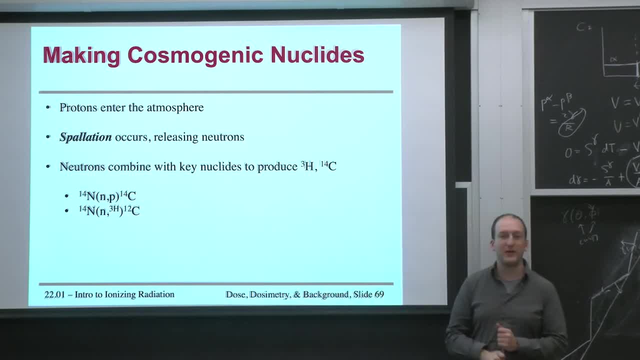 And then same thing for tritium production in the atmosphere. This is where some of that tritium naturally comes from is it makes carbon-12, which is the normal form of carbon, but out comes tritium, which there is going to be some constant isotopic fraction of tritium. 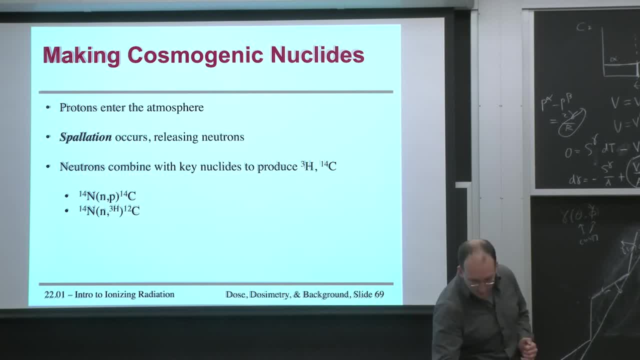 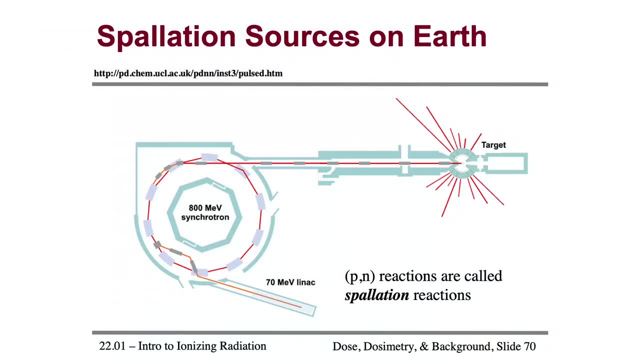 in all the world's hydrogens. Some of it's being generated in real time And we do have these spallation sources on Earth. Like I mentioned, the spallation neutron source has a gigantic synchrotron- We've seen these before- which just injects, in this case. 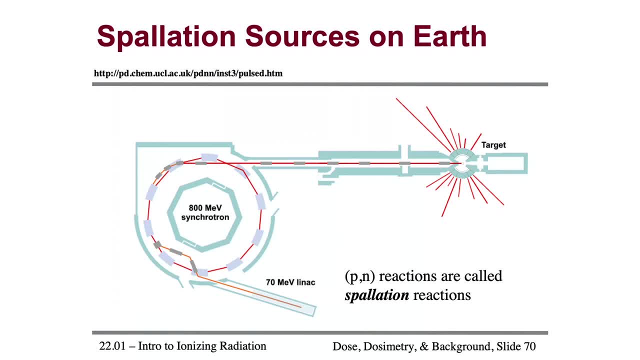 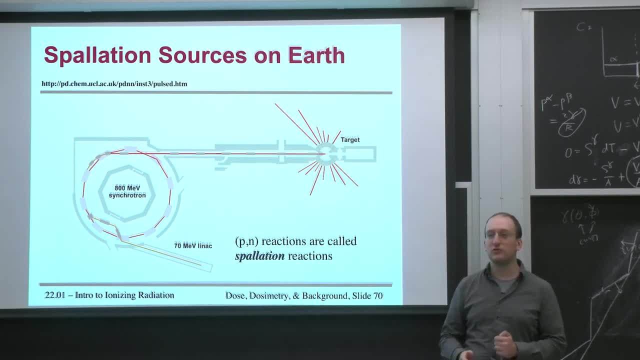 protons which circle around and around and around, accelerating until some of them are extracted and fire onto things like a liquid mercury target, some neutron-rich liquid metal. So you want something that's very neutron-rich. You want something that's very dense. 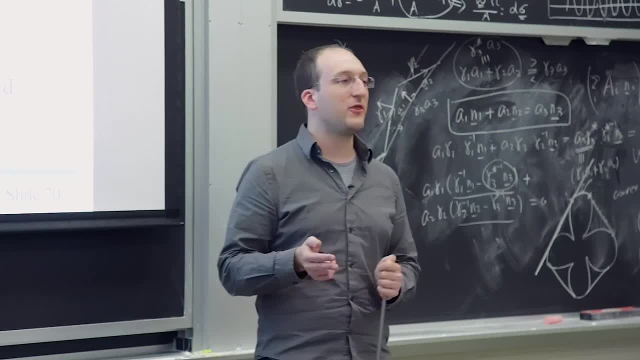 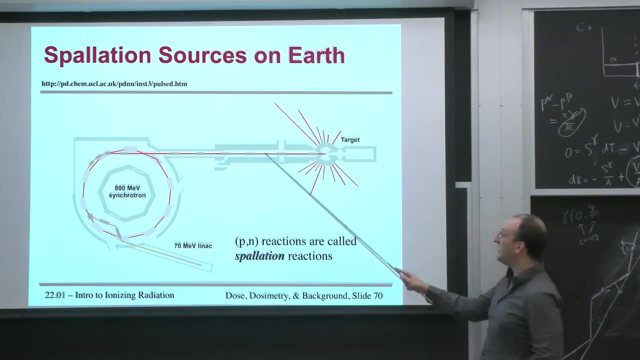 You want something that's fluid so you can cool it better, And you want something with high thermal conductivity. That's where the metal comes in. So a liquid metal you can keep cool really well because when you're firing lots of 800 MeV protons into it, 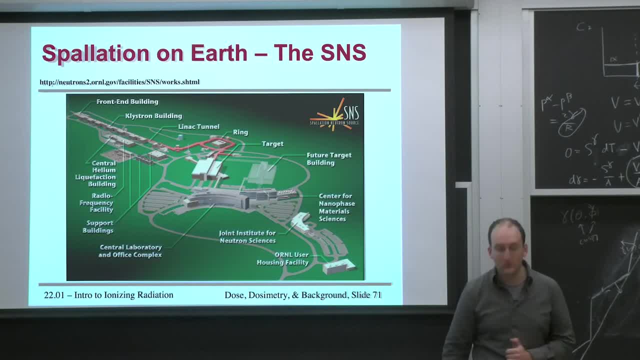 you generate a tremendous amount of heat, And this is what the actual thing looks like. You can get tours of this down in Tennessee at the Oak Ridge National Lab. Actually, I've driven up here before I recognize this from a map. It's pretty cool. 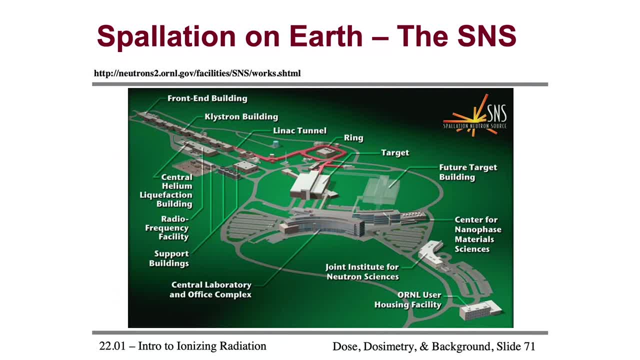 So where does this come from? It comes from the ocean. It comes from the ocean Where the actual neutron sciences stuff happens and where all the scientists sit with their targets. there's quite a bit of stuff going on behind it. So there is a gigantic, you can see, right. 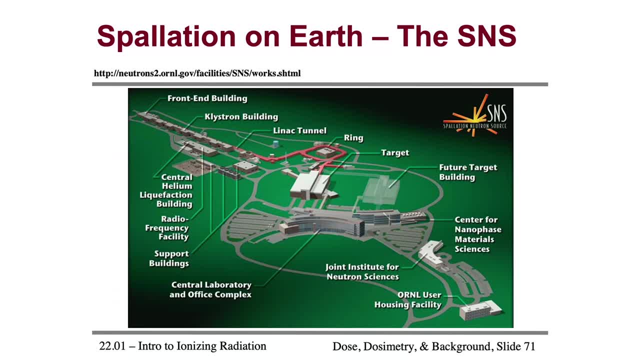 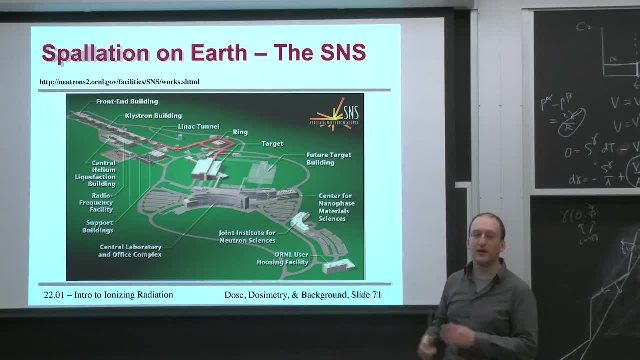 that's a parking lot for scale. There's a gigantic linear accelerator shooting into the synchrotron ring, which then fires the protons here into the target, into one of any number of end stations, which creates an not quite push button but turn-on-able pulsed neutron source. 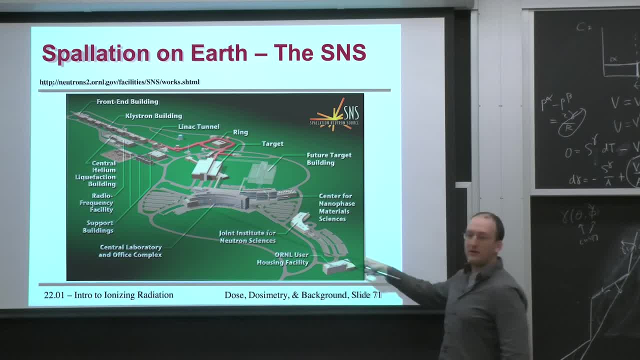 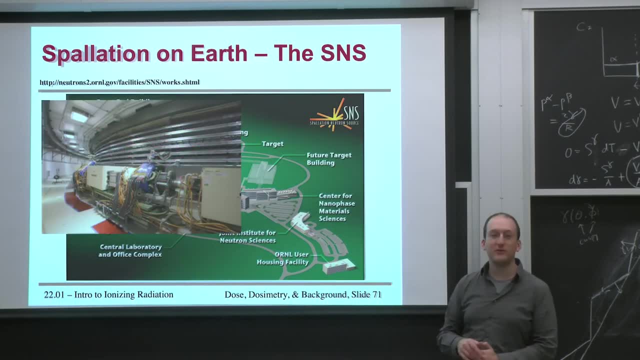 which is pretty slick And, again, parking lot for scale. Takes a lot of magnets to bend an 800 MeV proton. That's what it actually looks like. Has anyone ever seen one of these synchrotrons like at Brookhaven or at Oak Ridge or at anywhere? 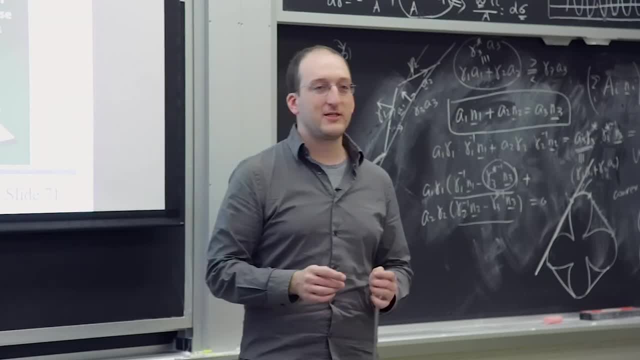 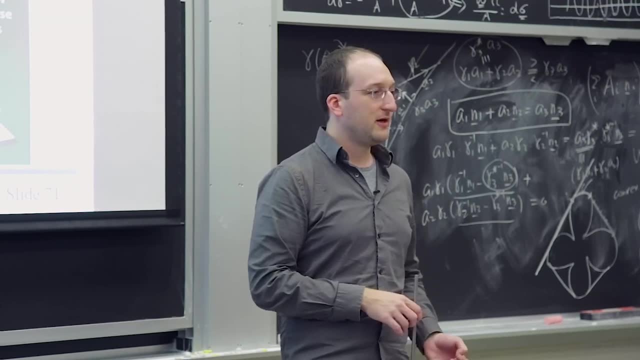 They're quite interesting things. The closest one to us is the NSLS or the National Synchrotron Light Source Version 2, at Brookhaven National Lab. It's like a 2 and 1 half hour drive down in Long Island. 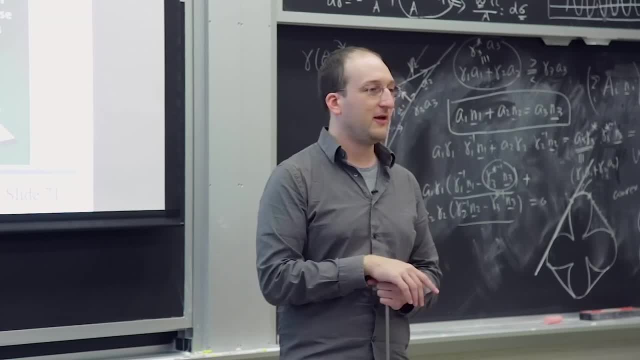 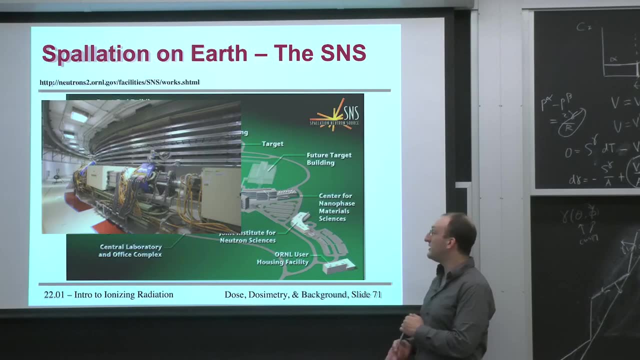 I don't know if they're doing tours yet, but it's about a kilometer around And I was told they did bike races around it to see who could beat the protons, which of course everybody loses, But they are pretty insane collections. 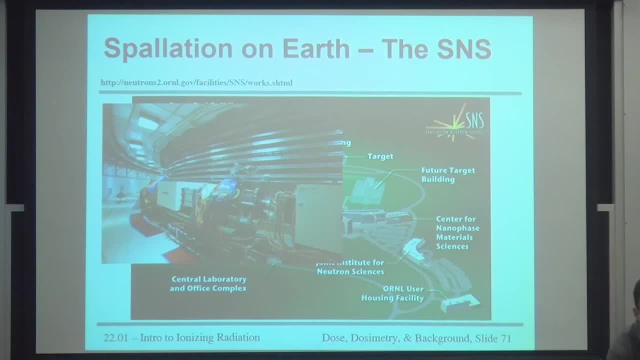 of magnets, vacuum equipment, And once in a while a proton will pass through, And then there's the spallation source itself. So this is what the target looks like. It's going to have to be liquid metal cooled in, And then out of here come lots and lots and lots of neutrons. 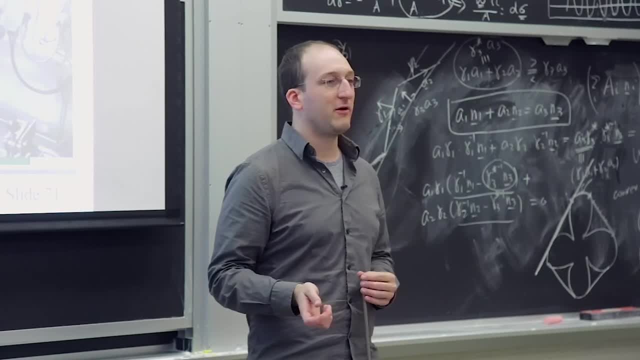 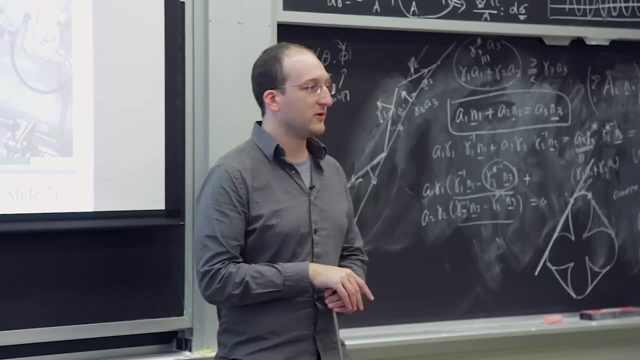 Enough neutrons that you still need hot cells to deal with things. They're still quite radioactive and activated. but it's not a reality, Right, It's a reactor, Other ways of making neutrons Speaking of, has anybody seen the pulsed fusion source? 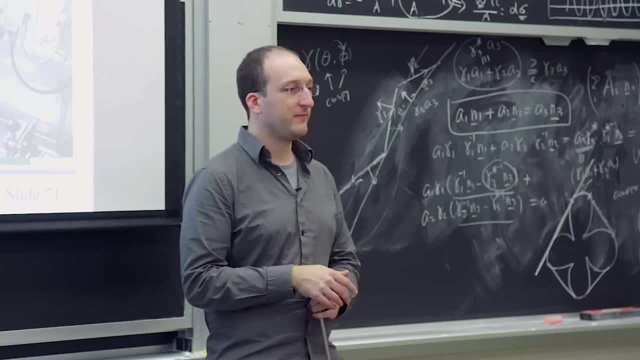 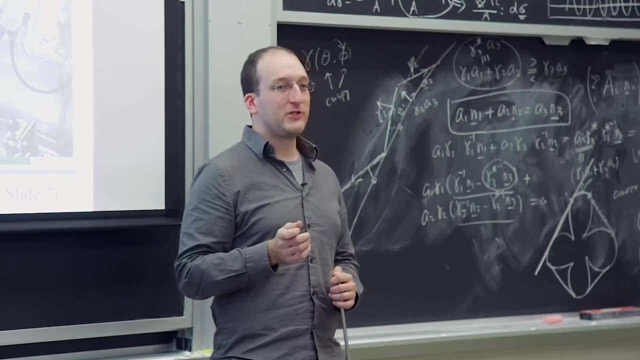 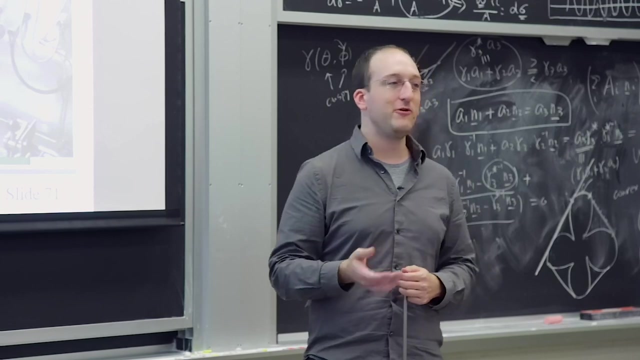 that we have down in Northwest 13?? No, We have a pulsed neutron source that you can come take a look at. It's an electrostatic fusion pulsed machine. There's a whole bunch of tritium and deuterium in this palladium sponge. what happens to hold hydrogen? 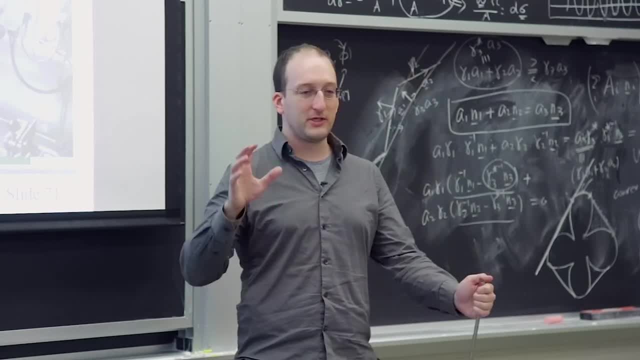 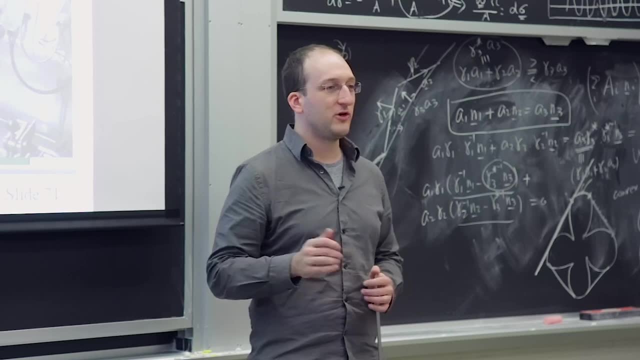 and its isotopes very well And with a very quick pulse. you can have a tiny pulse of fusion and generate about 10 to the eighth neutrons. that it actually is a push button neutron source. So if you want to see a neutron source beyond reactors, 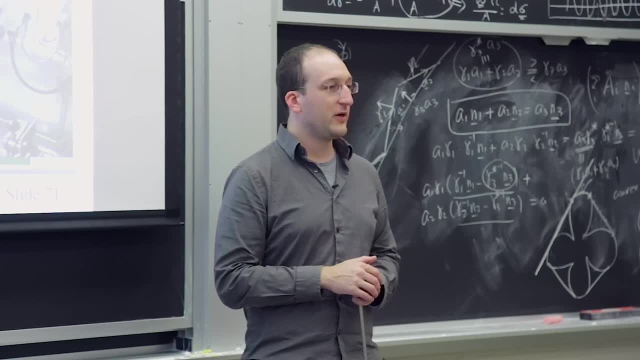 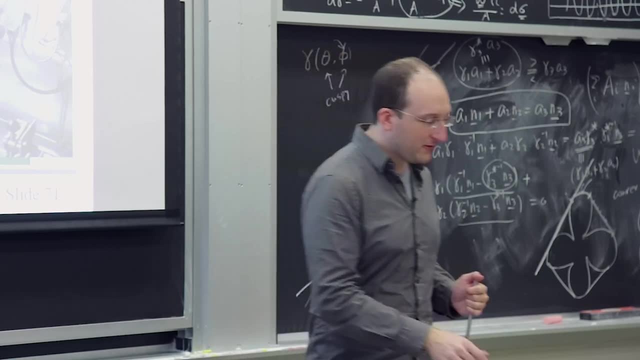 go down to the vault in Northwest 13 and ask to see that. We did a quick experiment before trying to activate cell phones to see what was in them. We did not generate enough neutrons to do so, But this cell phone has definitely seen a few fusion. 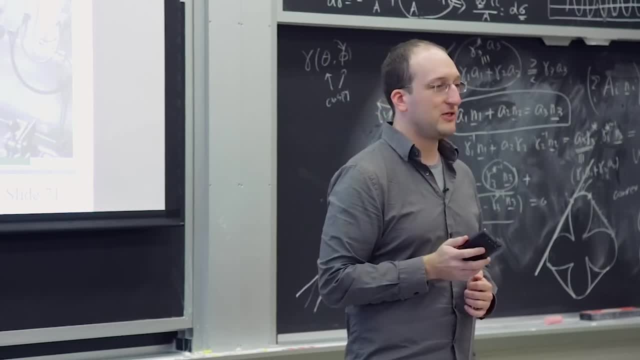 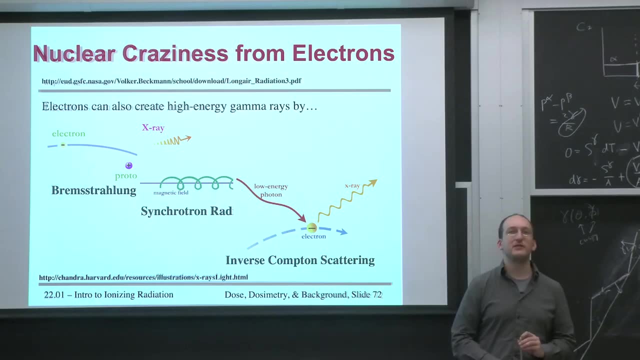 neutron pulses And we checked later. It's not giving off any residual radioactivity. At least we can measure. That was a fun failed experiment. And then comes the craziness. since it's about five of five of, I want to get into things that will definitely. 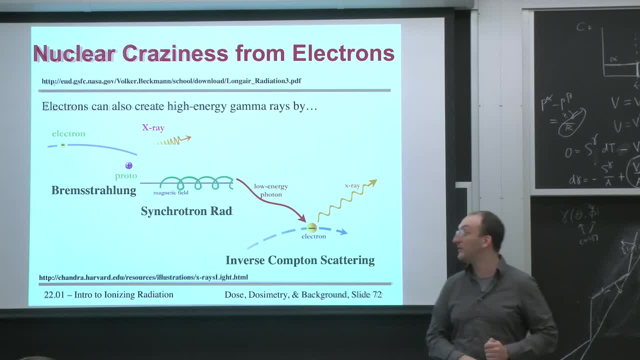 not be on the exam, So just sit back and enjoy and stop taking notes. Complete insanity can happen with super high energy electrons. We've already talked about Bremsstrahlung. We haven't talked about. we have talked about synchrotron. 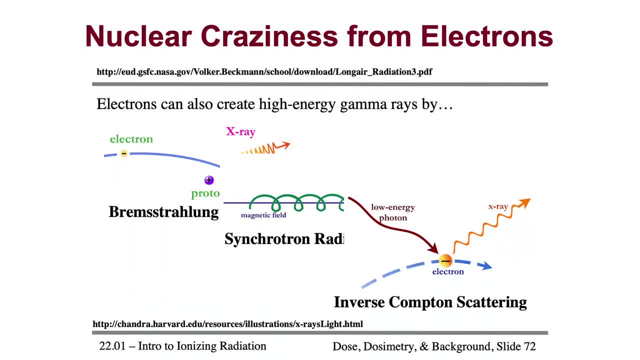 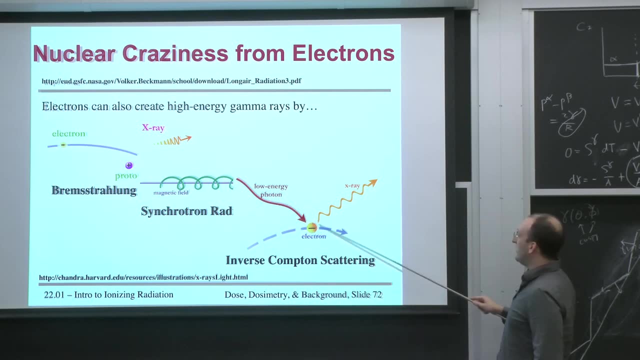 radiation, where you have a charged particle going along a magnetic field line, It changes direction and gives off x-rays. We haven't talked about inverse Compton scattering Interesting process here. In comes a low energy photon, hits an electron. out comes a higher energy photon. 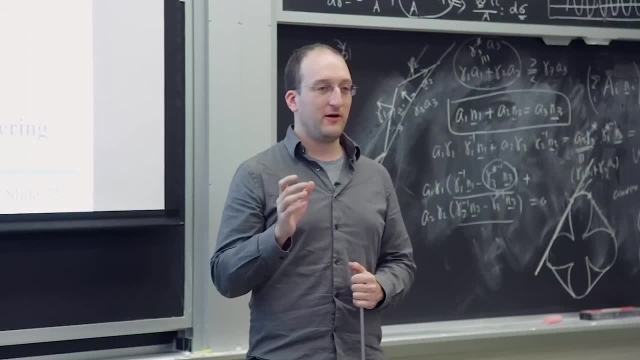 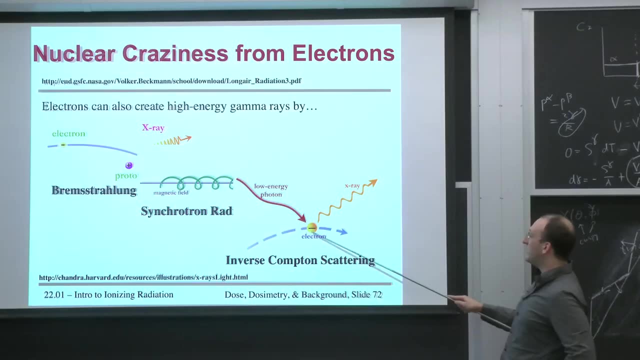 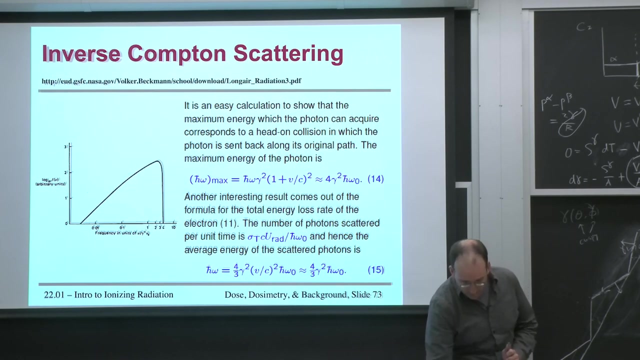 Compton scattering usually think of as the other way around. where a high energy photon comes in, scatters off, an electron loses energy. In this case, a high energy electron colliding with a low energy photon can impart energy to the photon. 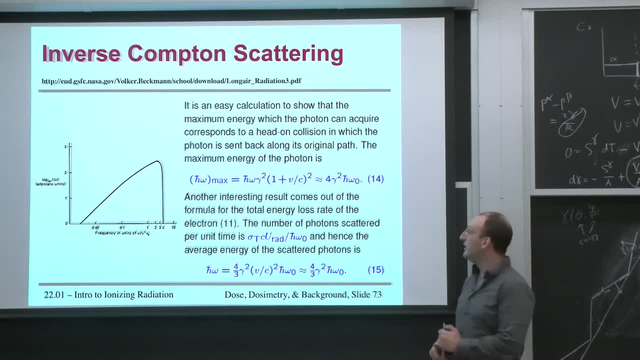 And you can actually calculate- or in this case, I've just taken This is a paper- the energy gain from inverse Compton scattering, as well as whatever cross-section there is, And even though this is a very infrequent process, well, the universe is pretty big and contains. 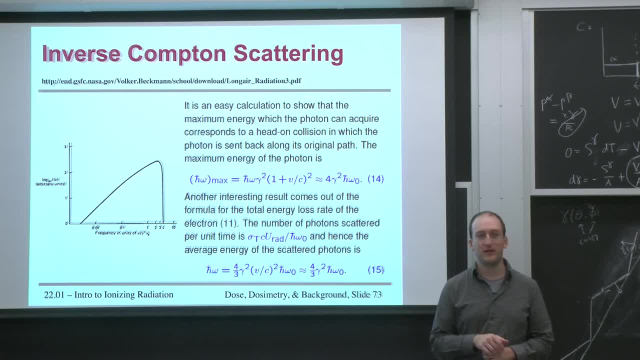 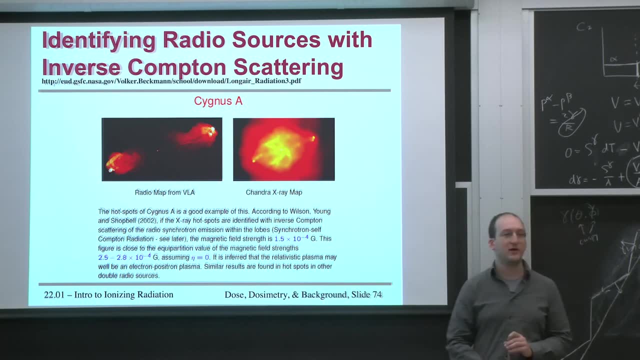 a lot of things that have magnetic fields, like stars and black, whatever else happens to have magnetic fields, And you can identify radio sources by looking for these inverse Compton scattered x-rays. So the Chandra x-ray map, I believe, a piece of which, 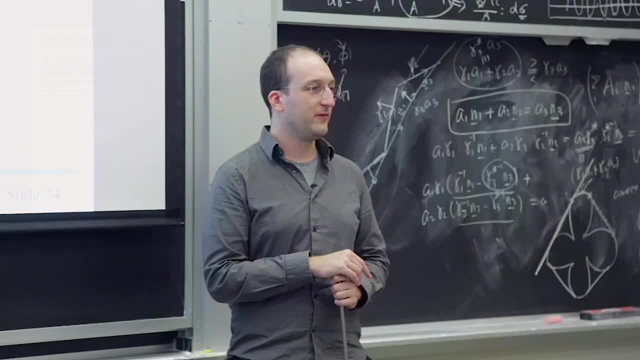 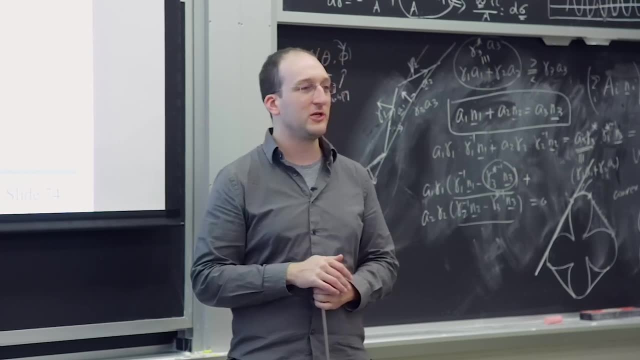 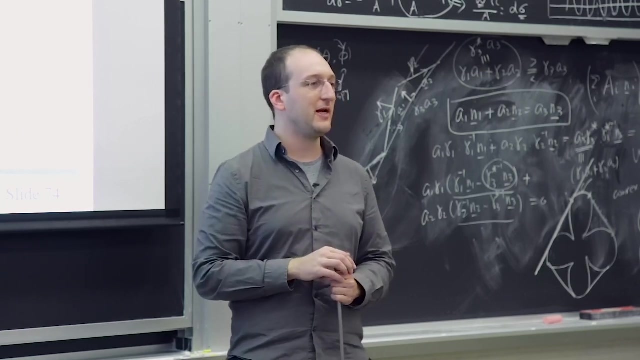 or a receiver for which It's up in the building in Porter Square. If you guys go down three stops on the red line, you'll see this little area full of Japanese noodle shops, Lesley University, a bunch of galleries And in a little I think it's still there in a little sign. 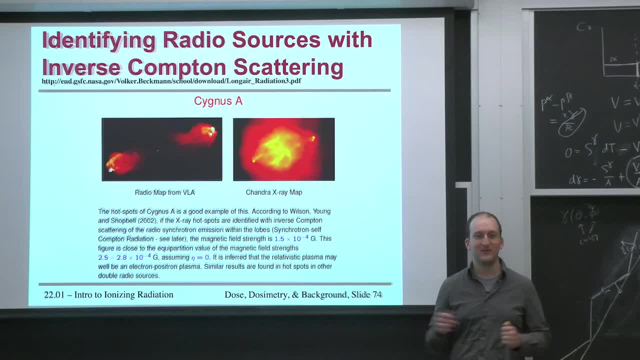 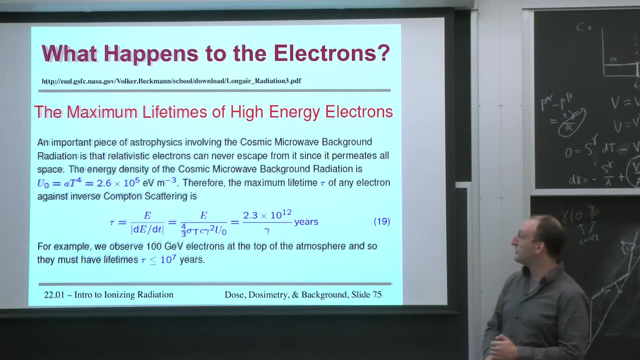 it says: oh, and there's the Chandra x-ray observatory. Whatever They may or may not have moved, but I recommend you check it out. And then what happens to those electrons? Well, they can actually decay. Pretty interesting things. 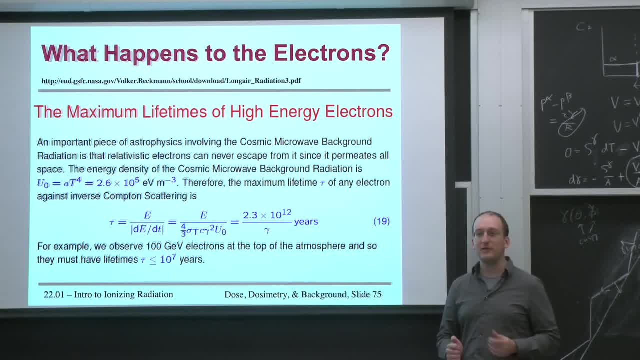 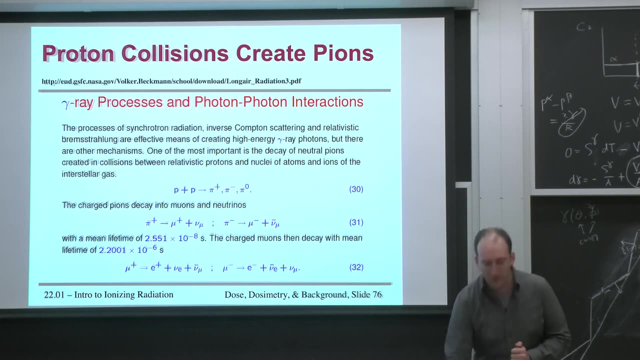 And so some of this inverse Compton scattering has gone into the evidence for or against where cosmic rays come from, because you should see electrons of a certain energy after undergoing this process. I think I will skip ahead. Oh, I won't skip ahead. 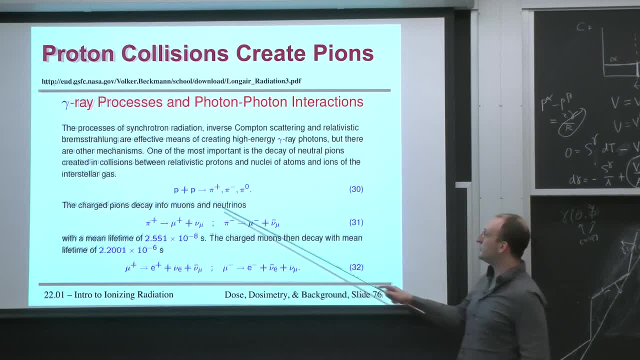 And so what these charged particles, what these cosmic rays can produce is what's called positive, negative or neutral pions, other subatomic particles with masses somewhere between protons and electrons that themselves can undergo different reactions or different decays into muons. 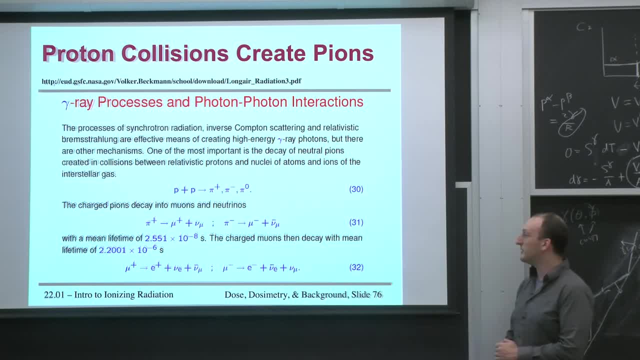 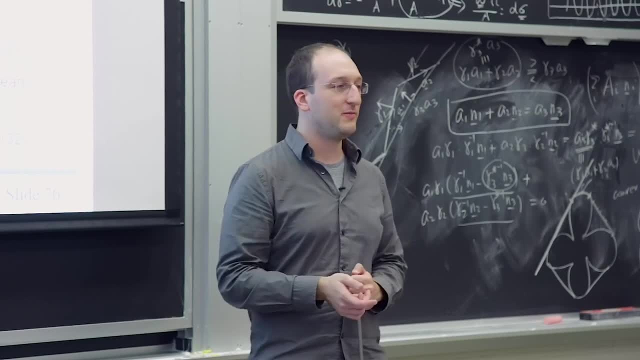 And don't worry, muons and pions and such are not part of the topic of this course, But they do have known lifetimes, They do have known masses and charges. They do have known stopping powers. We should be able to measure them. 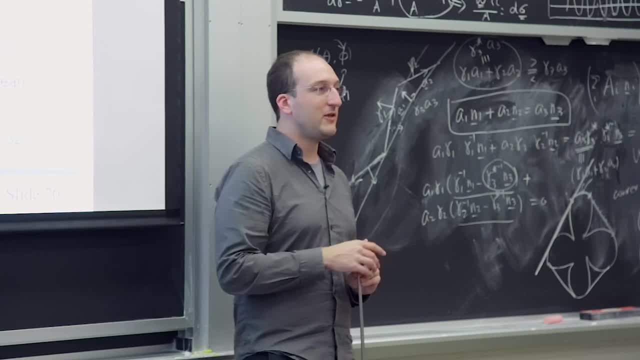 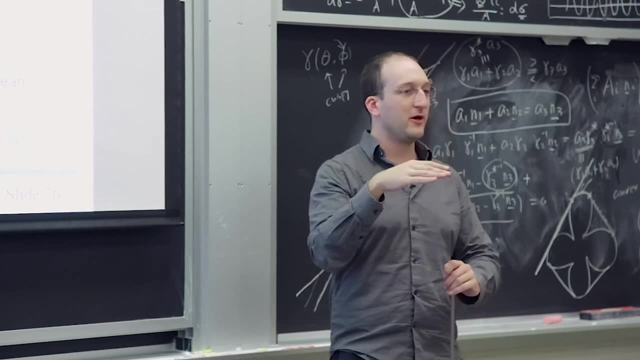 And there is a cosmic muon detector at Boston University- Rather, it's a pair of detectors that looks for this coincidence of one muon scattering off one detector or interacting and another particle being sensed and directly beneath, So we can actually sense these muons. 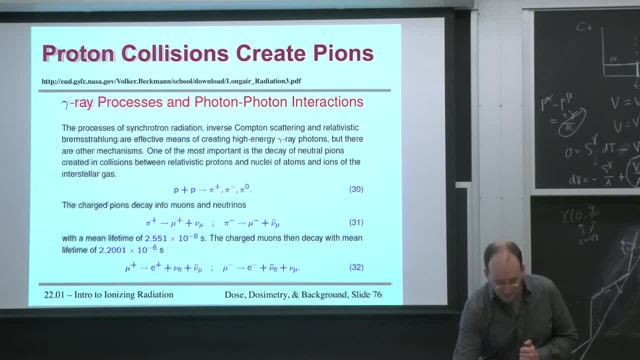 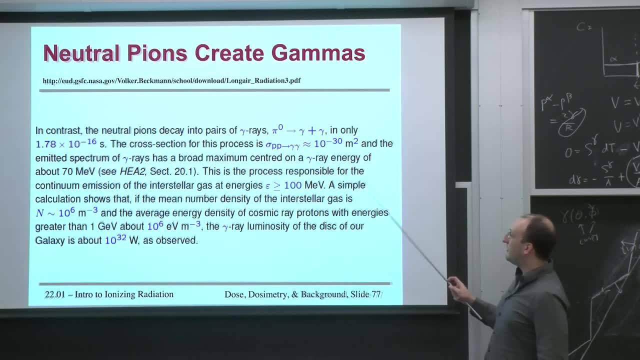 to confirm or refute the theories about where they come from in terms of cosmic rays, And these neutral pions are what end up creating these gamma rays. I think they were around like the 70-something MEV range. So if these theories about them are correct, 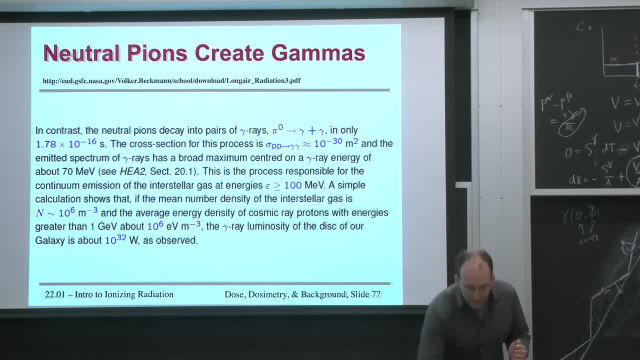 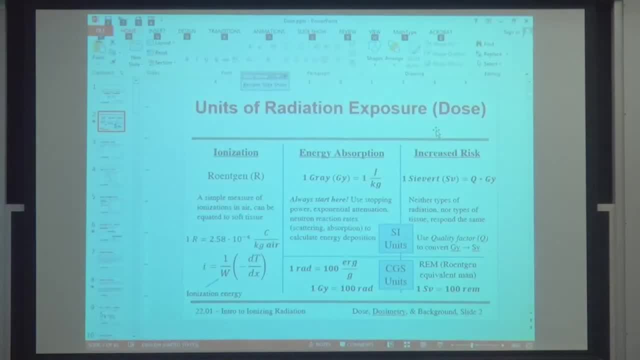 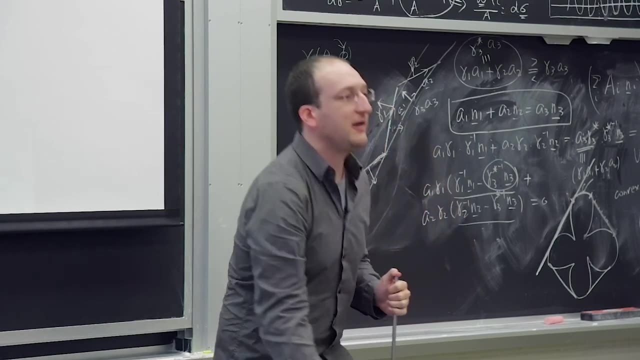 we should be able to sense these gamma rays and sense how many of them there are as a function of energy. That's not what I wanted to do. Let me recreate presentation mode, because this is definitely delving into the kind of stuff that, well, I'm not an expert in. 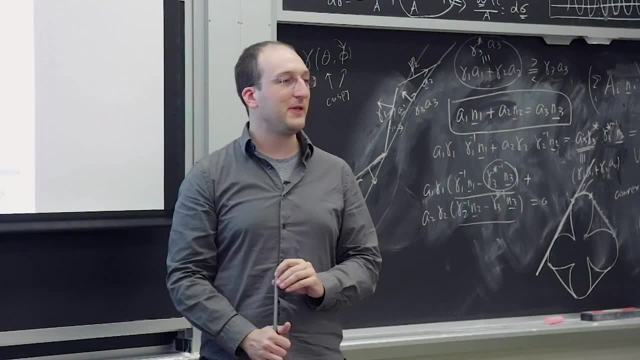 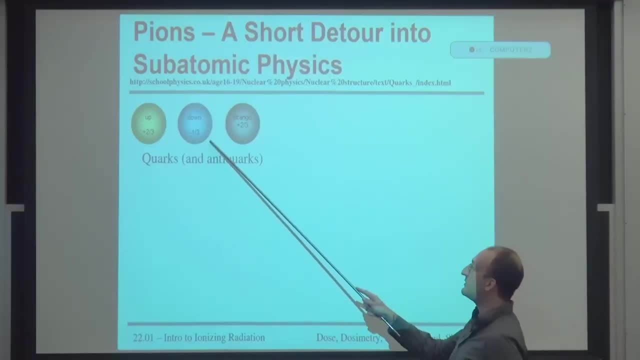 So a quick detour into some atomic physics. You guys probably have heard of that. protons and neutrons are not the smallest building blocks of matter. They themselves can be composed of quarks and anti-quarks with different charges and different masses. They're given different flavors. 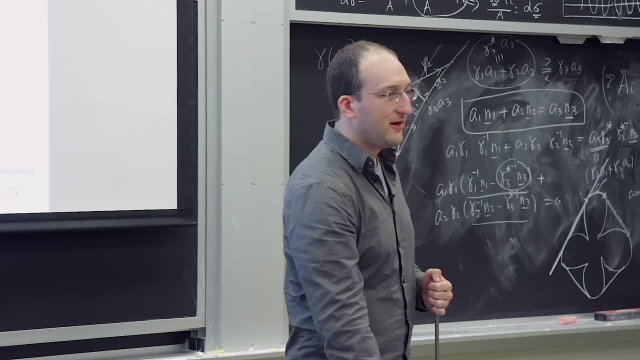 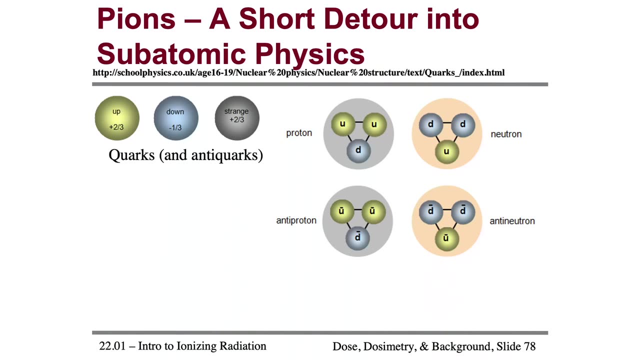 I don't know who came up with this term. It's terminology but it's kind of fun. Things get kind of whimsical when you get into subatomic physics. And these quarks and the gluons between them are what composes protons, neutrons. 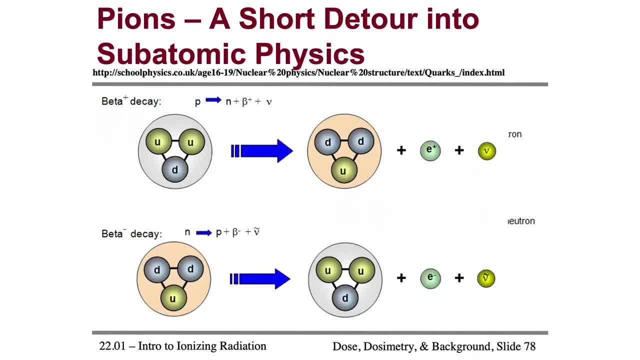 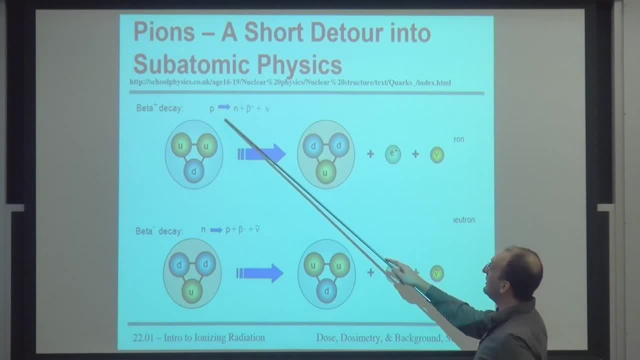 and their antimatter counterparts, And these sorts of things can also undergo their own decay and reactions. So when beta decay occurs, it's actually one of these up quarks turning into a down quark and releasing an electron and an anti-neutrino. 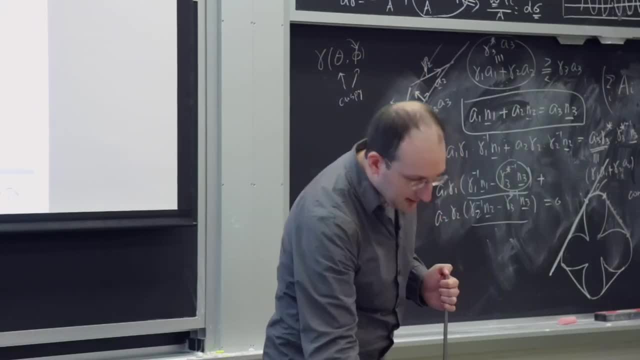 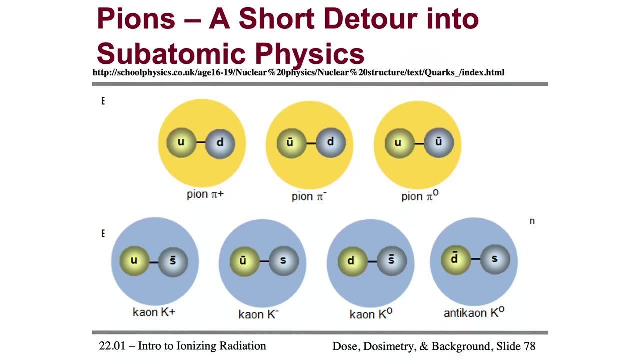 But again, we're not going to. We're going to delve even deeper into this. There are other particles composed of other arrangements of quarks. So if you have just an up and a down, you have a positive pion which should have a charge. 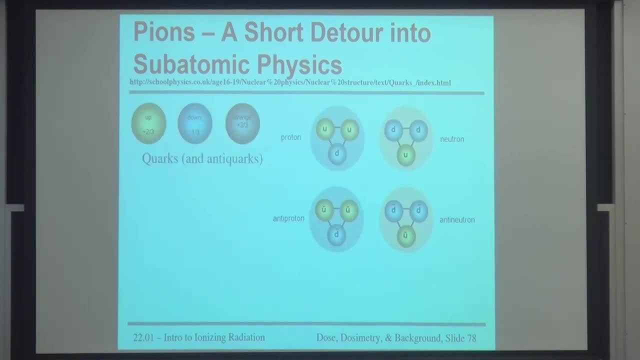 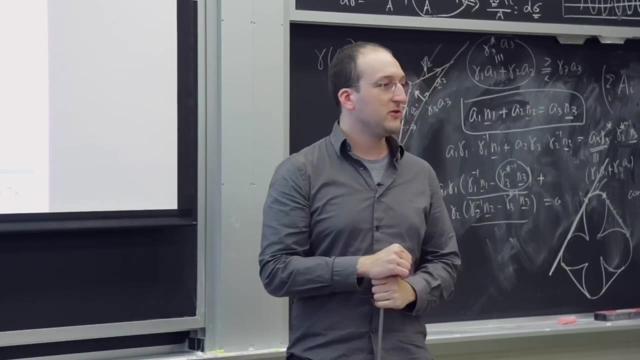 I think one's 2 thirds and one's minus 1 third. Yep, that is correct. So a plus pion should have a charge of 1 thirds, the charge of an electron. So you know the mass of some particle because you know the number of quarks. 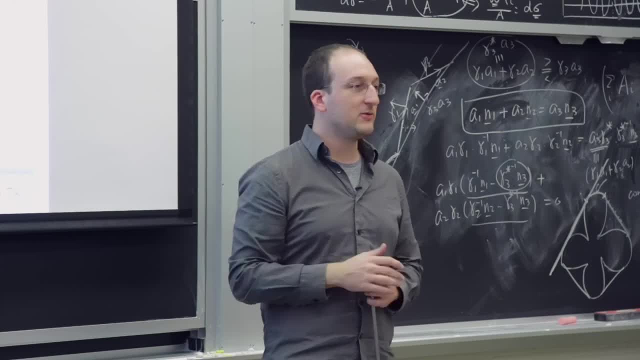 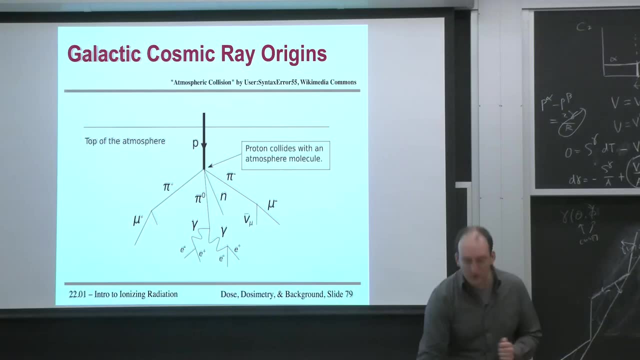 And you know the charge of it. You should be able to calculate It's own stopping power and figure out how many should get through the atmosphere and such or how many get absorbed in your detector. And so, when a very high energy proton collides with an atmospheric molecule, it creates neutrons, creates a shower of pions. These neutral pions, much like electron positron interaction, can produce their own gammas, So they can spontaneously decay from particles that are mass into gamma rays of pure energy, which then go. 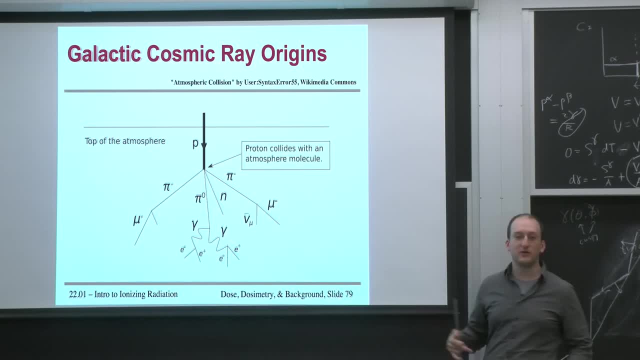 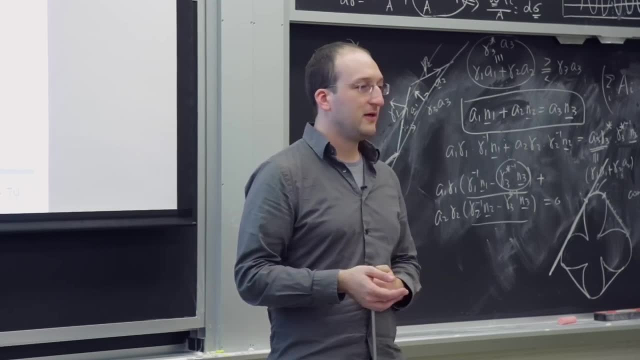 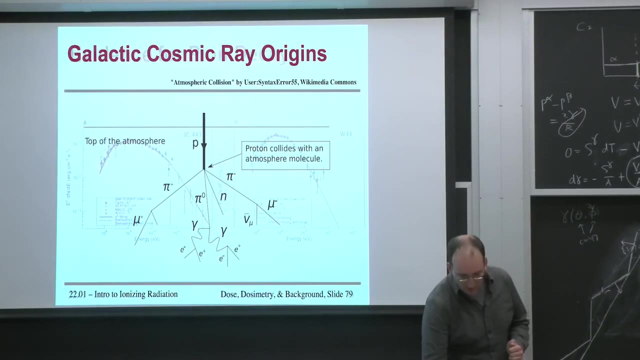 on to create their own shower of electrons and positrons by pair production, Because, as we saw, the higher in energy you go for photons, the more likely pair production becomes. And there you have it. This is part of the 2201 stuff, but taken to the nth degree. 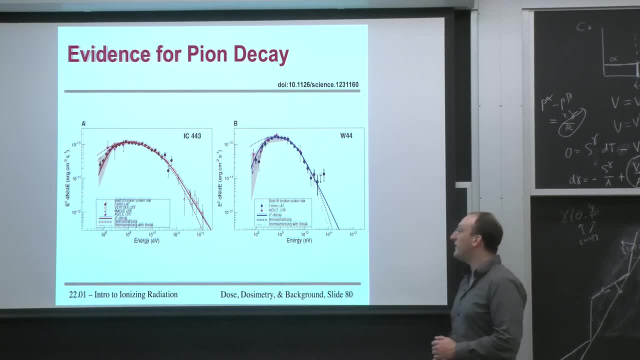 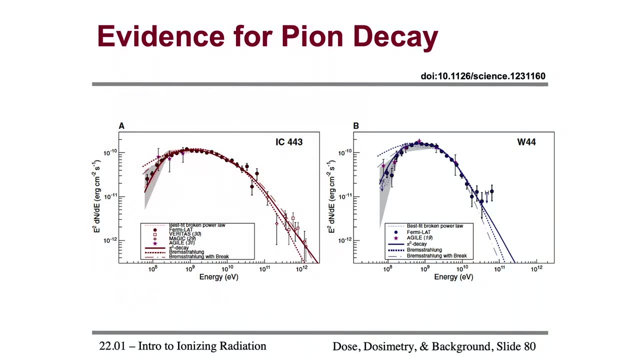 And then the evidence for pion decay comes from extremely fine measurements of the number of these pions as a function of energy. Or in this case, look at that: What is it? Berg's percent of mu squared? Yeah, Berg per second. 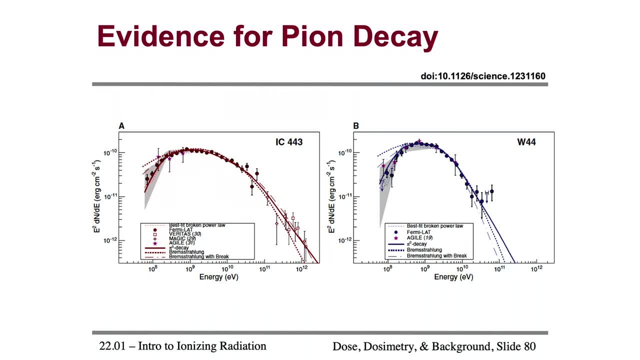 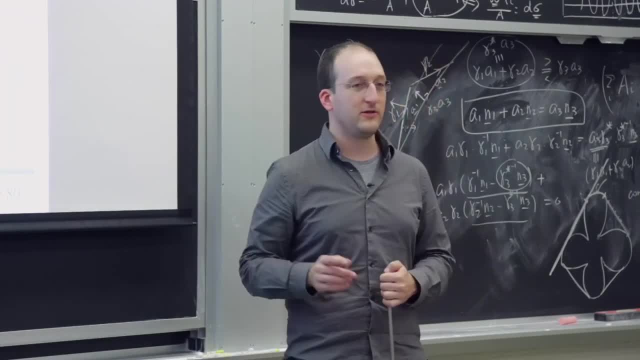 What does that unit physically mean? I'm not going to get into that, But at any rate there are different models for how many of these pions and their high energy gamma decay products should be observed, And by looking at those very carefully. 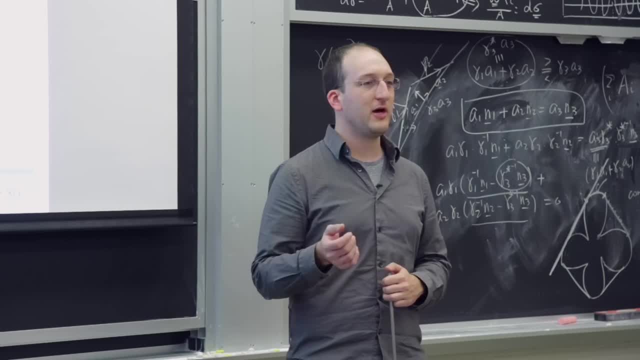 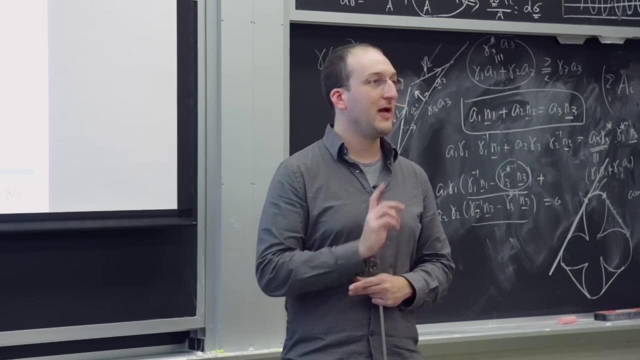 you can tell where they came from. Should they have come from coronal mass discharges? so we should know what energy those protons should be, or some other source? I am going to stop there because it is five of. So, after that crazy detour, give you guys 10 minutes to degas. 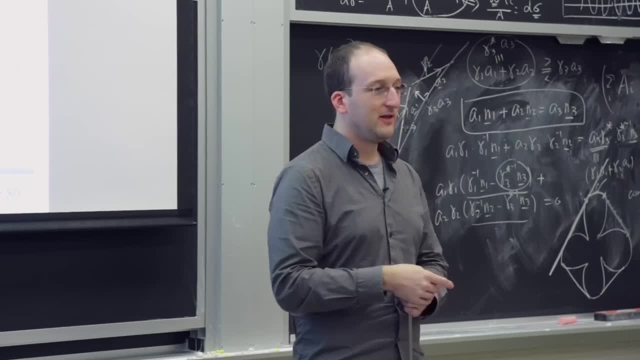 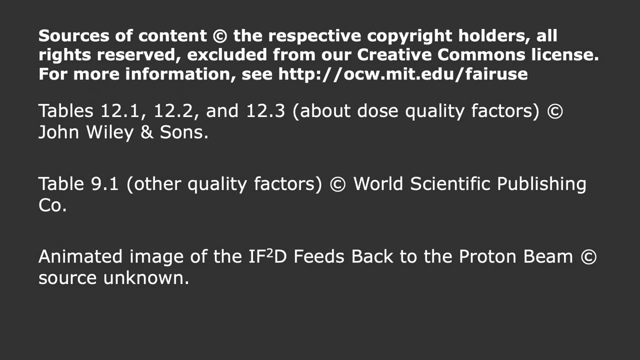 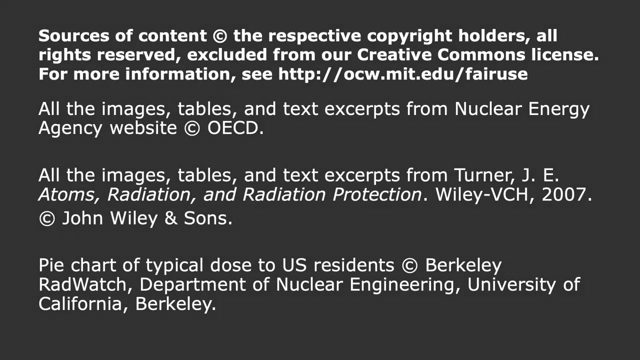 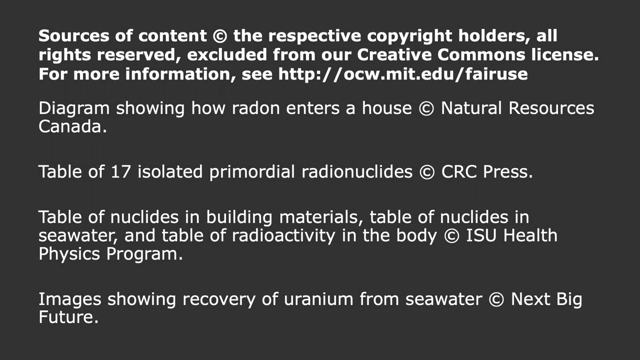 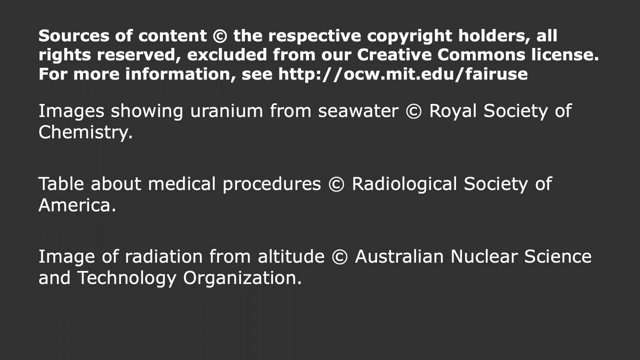 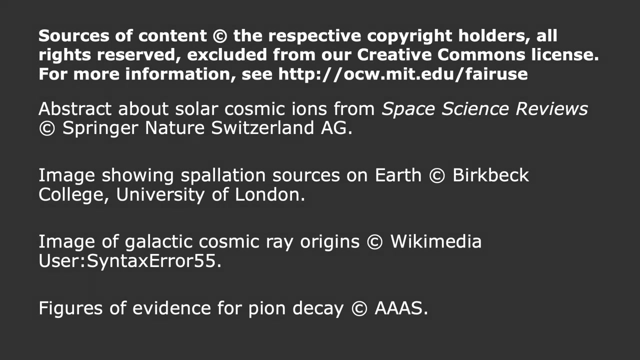 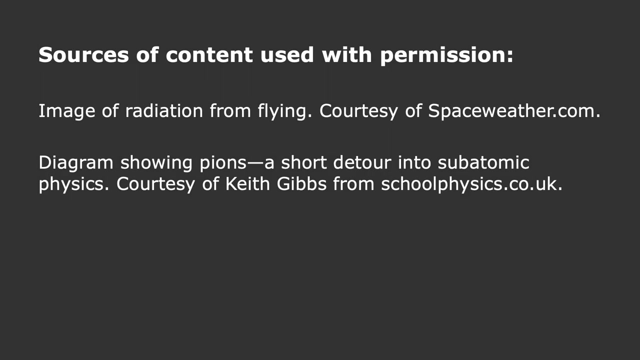 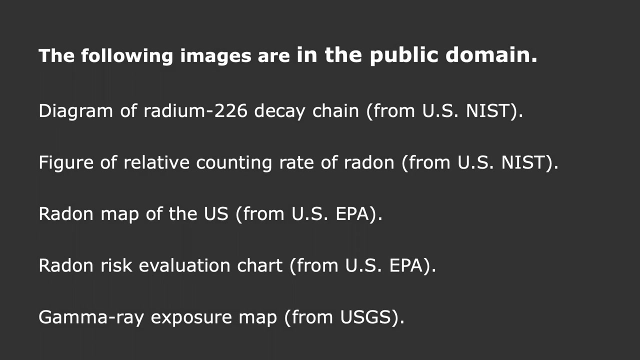 and absorb some neutral pion gamma decay products. We'll meet upstairs in 10 minutes for an exam review. All right, guys. thanks so much for watching and I'll see you guys next time. Bye.